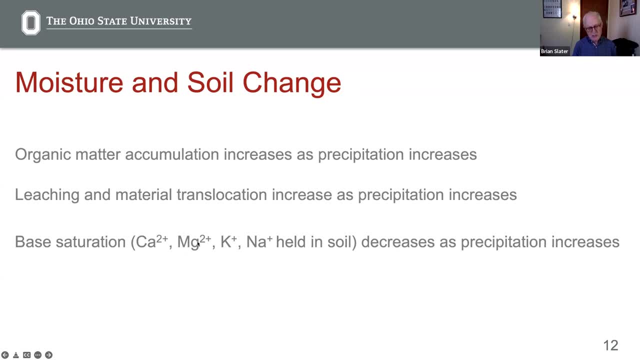 So as precipitation increases, the amount of these metal cation nutrients is decreased. So if we compare, say, the southeastern part of the United States or tropical soils, they typically have much lower levels of these metal cations than soil, say, in relatively young environment like the western part of Ohio, where they've only had 12,000 years of leaching. 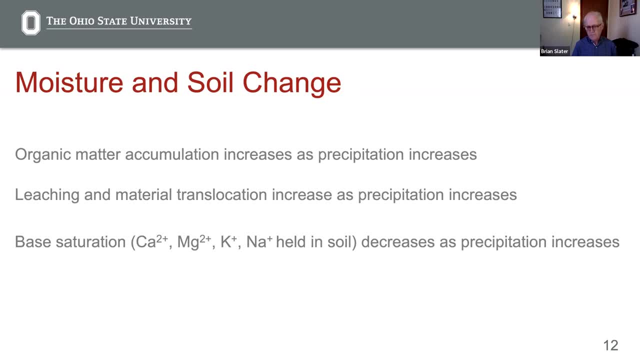 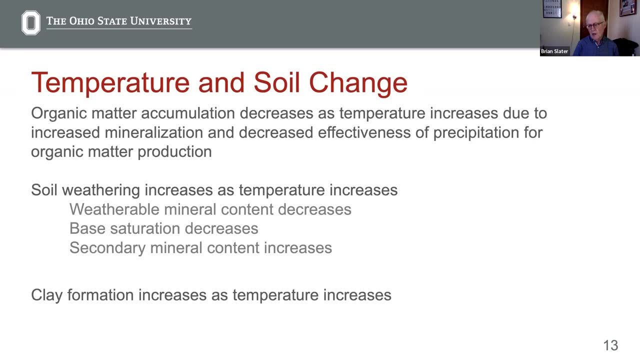 Even under a 40-inch rainfall condition. So there's some just very general rules about precipitation, And we can also say similar things about temperature. So organic matter accumulation decreases as temperature increases due to the increased breakdown of organic matter that we call mineralization and decreased effectiveness of precipitation. 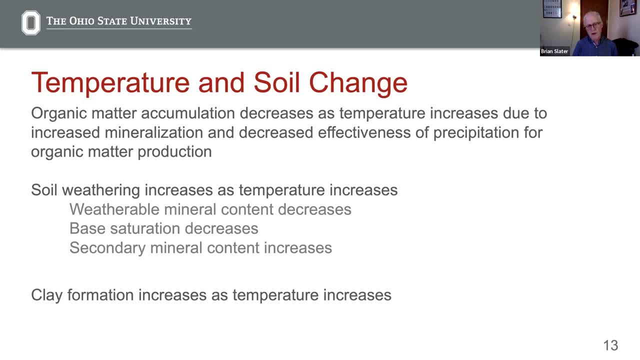 Because if we have higher temperatures we get more of that transpiration and therefore drier soils typically. So we can see that if climate change influences temperature- and we know it already is influencing that increasing temperature- then we would actually expect that organic matter in soils is going to break down. 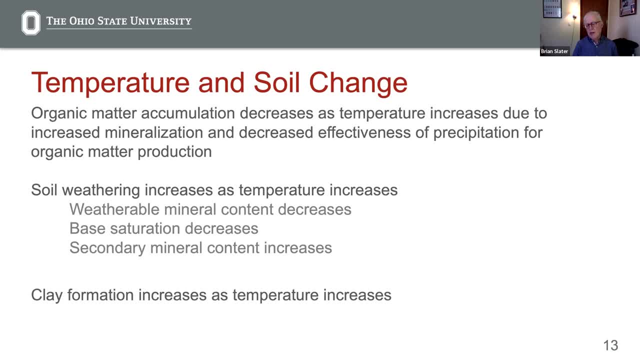 But remember, we also get increased production to some extent with higher temperatures. But it's complicated, of course, because it depends on the seasons. But another long-term effect is how soils form. That process we call weathering. Soil weathering increases as temperature increases. 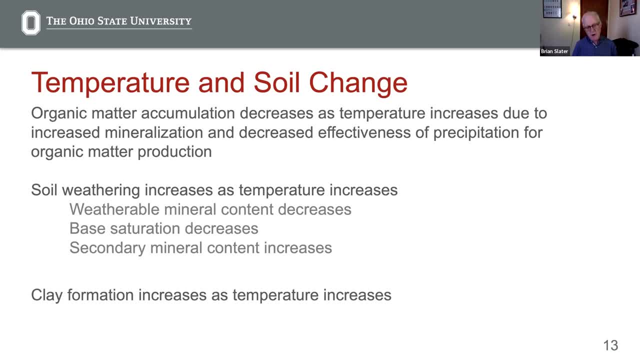 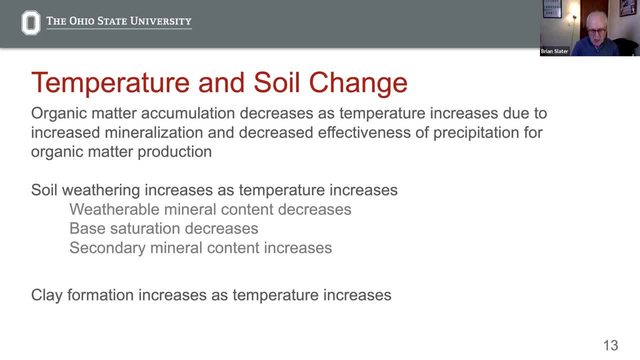 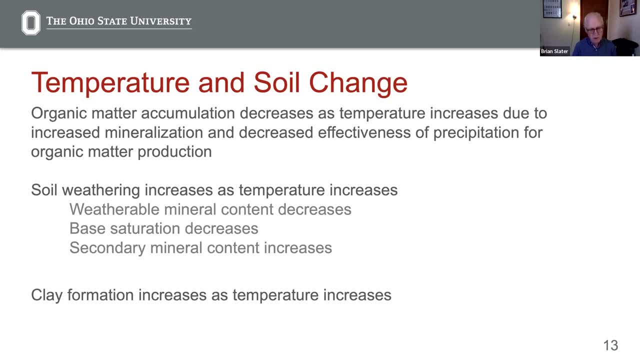 So as we go to the southern states of the United States, soils tend to get redder, and even more so into the tropics. But other forms of soil weathering also increase. Remember that as temperature increases, Soil weathering increases, Microorganisms can and plants can grow faster. 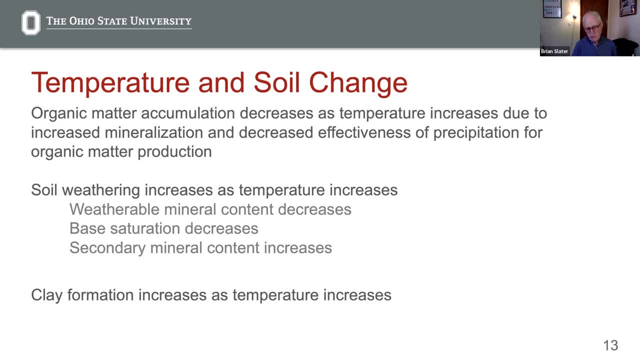 So we talk about weathering the change of the original minerals in the soil parent material. The amount of residual weatherable minerals decreases as temperature increases. So in Ohio we have some residual minerals. If you look in many Ohio soils we can see things like micas and deep in the soil 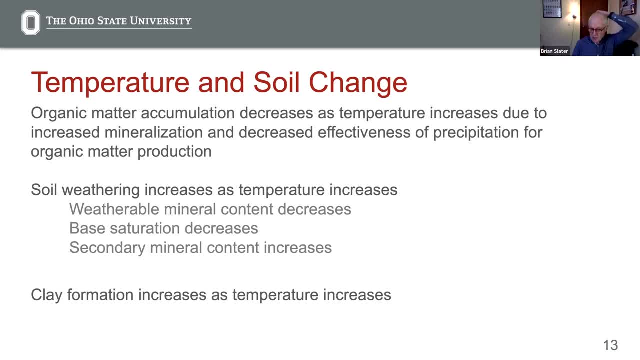 We might see calcium carbonate, The ice in the soil from the limestone or lime-rich glacial deposits. we still have some of these minerals that can break down over time, because we're in kind of this mid-latitude climate, But as temperature increases, weathering will increase. 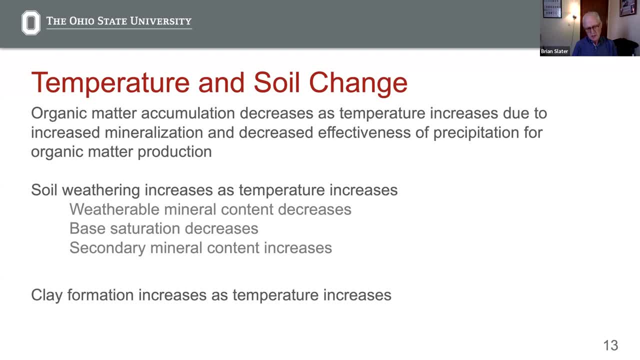 and therefore the amount of these residual minerals will decrease. We've already talked about a saturation decreasing. It also decreases as temperature goes up Because of the faster rate of chemical reactions in soils, And then minerals formed in soils like clay. clay is produced in soils as they weather. 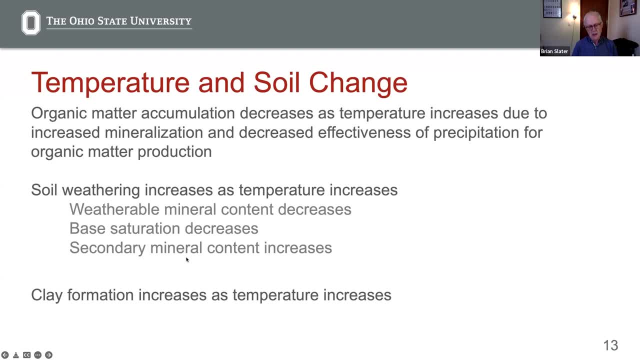 these will tend to increase as temperature increases. So hot places tend to have more clay. everything else being equal, Clay formation increases as temperature increases. So these are just some kind of generalizations of what we're seeing in the climate. So these are just some kind of generalizations of what we're seeing in the climate. 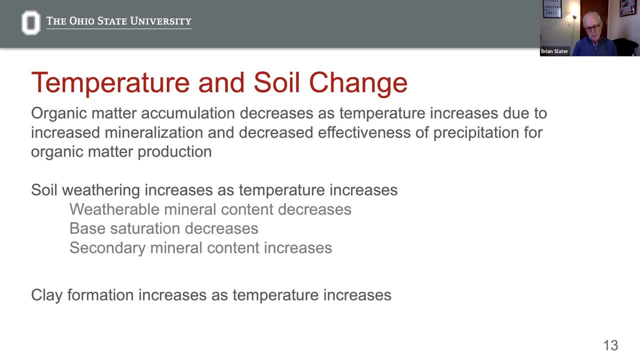 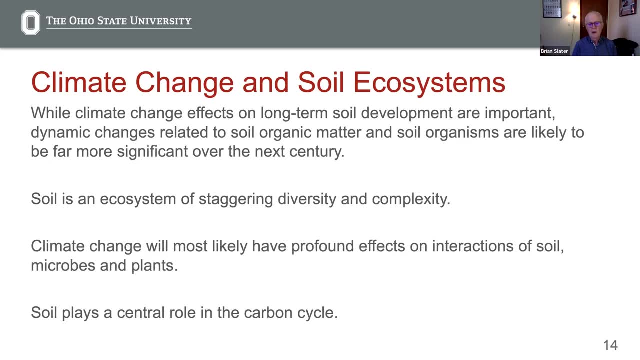 So these are just some kind of general rules of thumb And again they operate sort of at the continental and regional scale, not so much at the scale of farm fields and forests. So these are kind of climate changes that affect long-term soil development. 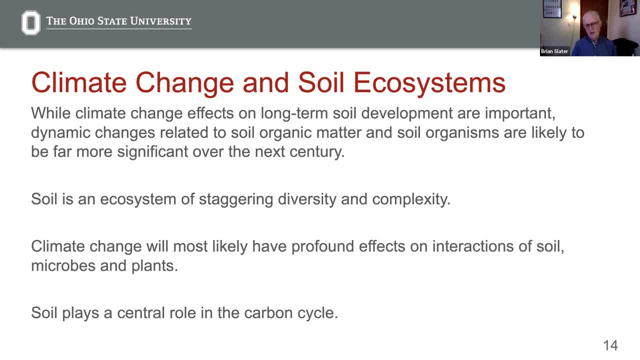 So what kind of soils do we get in different places? So climate has affected those things. But much more important to us, I think, when we think about climate change, is dynamic changes related to things like soil, organic matter and the microorganisms and plants and animals that live in the soils. 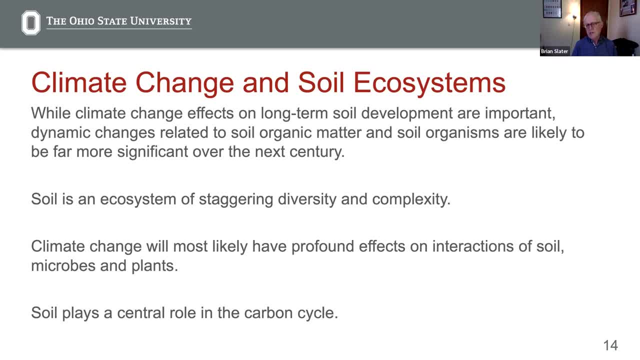 And I think these are where most of our thinking and concentration is in terms of climate change, And we know that soil is a staringly diverse environment or ecosystem that we really don't understand very well. As I mentioned earlier the effects on the microbial community, 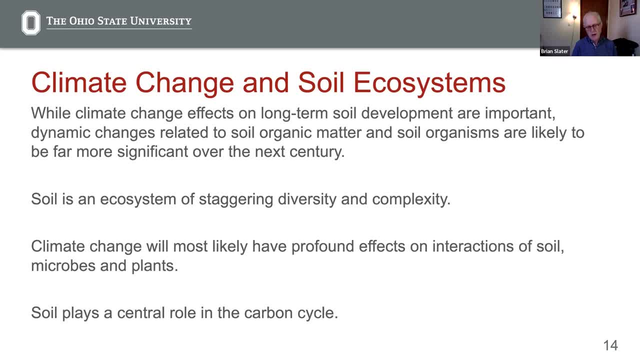 and relationships between microbes, plants and the soil matrix is really just in its infancy in terms of science, So we don't know as much as we need to to be able to make predictions or even manage the system well, But we know that climate change is going to have profound effects. 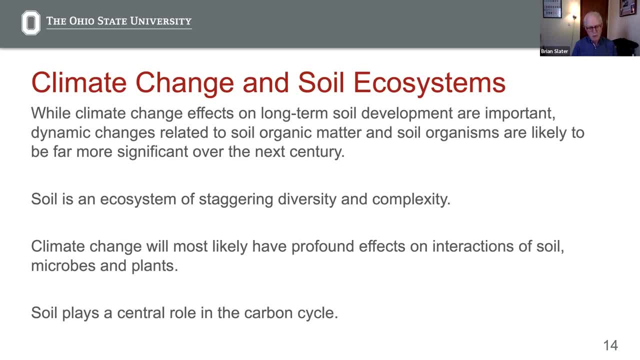 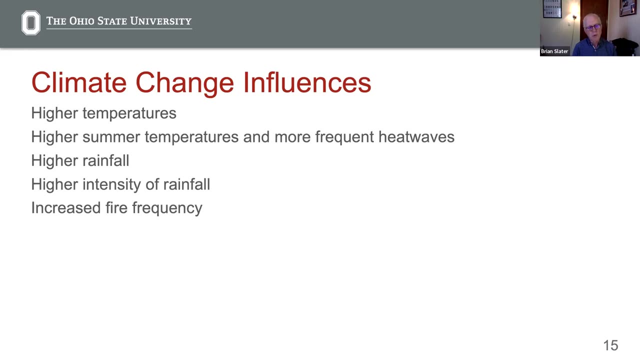 on interactions between soils, microorganisms and plants, And this is important because soils play the central role in the global carbon cycle. So if we think about how climate is changing and will change, we are aware of ideas and models that show and measurements. 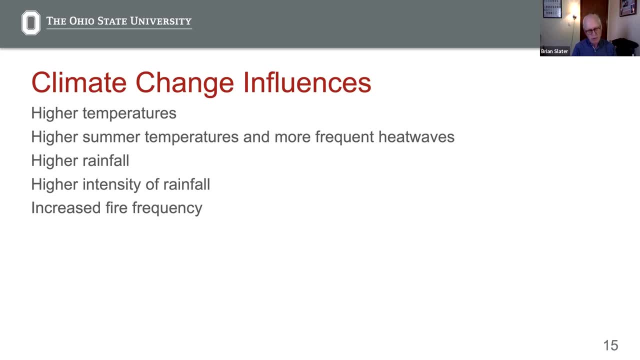 that show higher temperatures. Probably we're already seeing effects of higher summer temperatures and more frequent heat waves. You know we're already seeing effects of higher summer temperatures and more frequent heat waves in our environment. Probably we're already seeing effects of higher summer temperatures and more frequent heat waves in our environment. 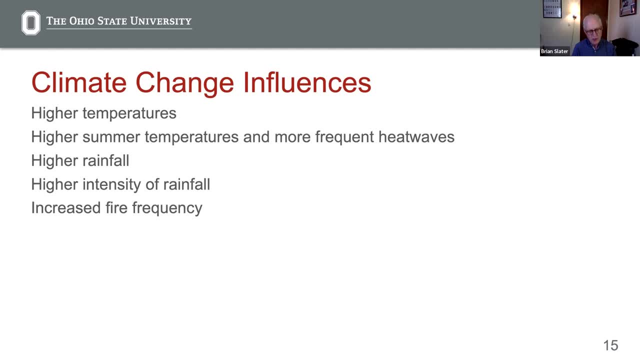 Between Ohio and across many parts of the United States and the world Generally. rainfall is increasing to some extent And we, As far as models go. there's some uncertainty here, but higher rainfall is likely, But even more likely is higher intensity rainfall. 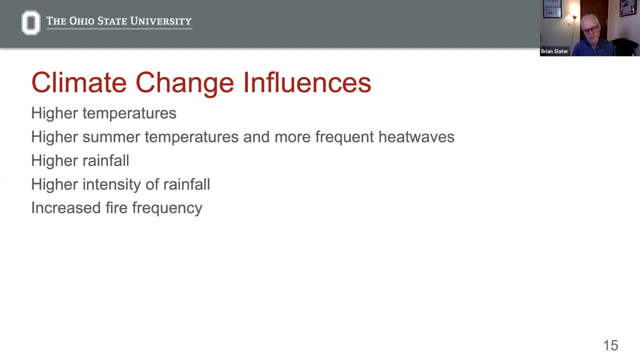 So if we think about how this might affect soils, You know, if we get very intense, short storms, that's actually less effective for getting water into the soil. that's actually less effective for getting water into the soil because more water is likely to come out. 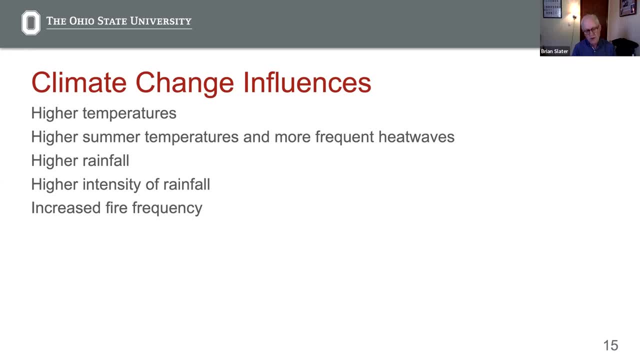 that's actually less effective for getting water into the soil to run off. under those conditions, we are also likely to get much more potential for soil erosion, where we have high intensity storms increasing and then we have influences on fire frequency, which can remove vegetation that protects the soil in various ways. 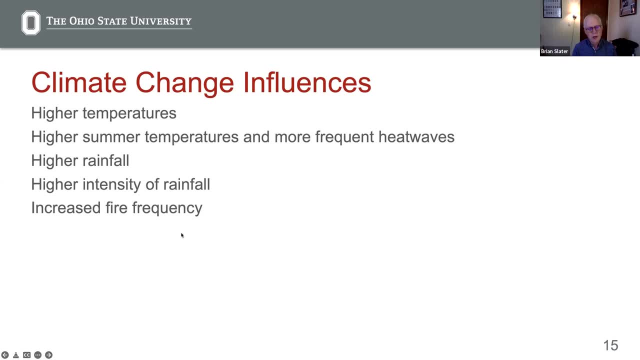 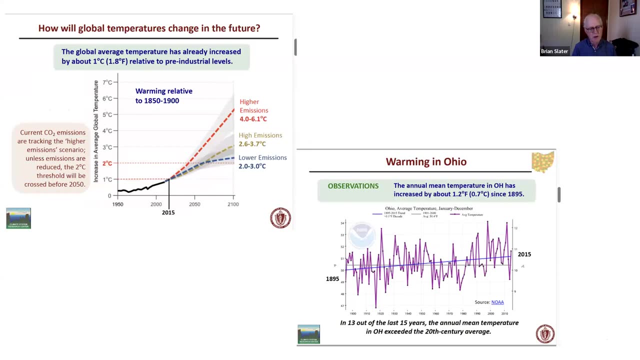 and adds carbon to the soil. um, i'm not going to reiterate uh for much time, uh, what we expect and know about climate change. i'll just very quickly summarize uh from this is uh, from some work done, uh at uh university of massachusetts. uh, and i acknowledge that i'll provide references to all- 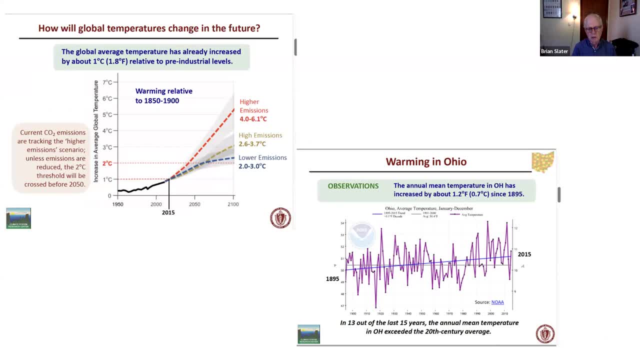 of this material, uh, uh in, uh in the powerpoint. i will uh that we will be posting later. so we we know that temperature is increasing and we know that there are various models that relate to different levels of emissions. but we've already had uh changes, uh in ohio, uh over, you know, even in the last 150, 150 years, and we see this, we expect. 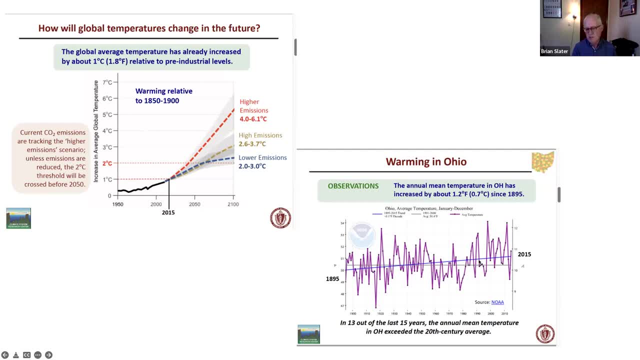 these things to increase, uh, and so you know, within the noisy signal, uh, we know that the temperature is increasing. this is the, the mean annual temperature. so, uh, since 1895 it's been about 1.2 degrees uh fahrenheit, uh, 0.7 celsius in ohio, and- and we know that models are going to show- 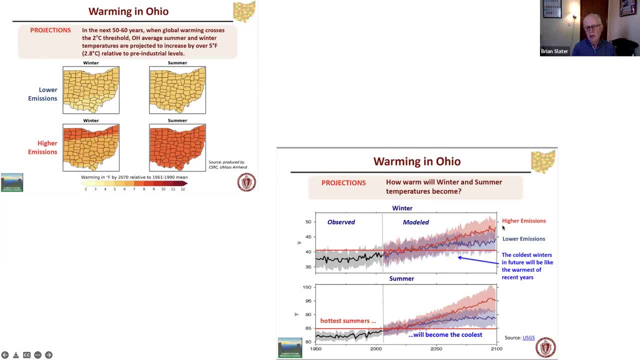 uh, uh, this this happening, um, and it will be something that is dependent on the season. so, uh, depending on what happens with the climate, uh, we may get warmer winters, but we may even have, uh, you know, some summers. the very warmest ones actually may end up being cooler, uh, but we can see this overall effect over time. uh, but it will depend. 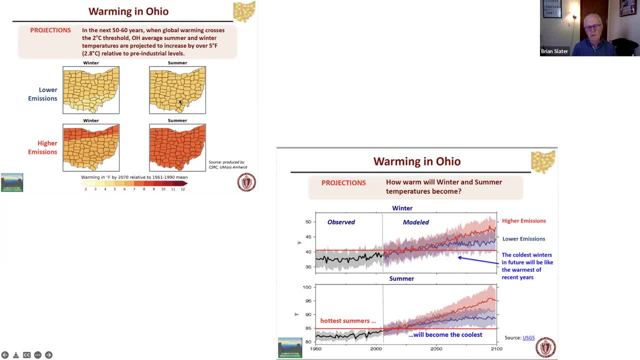 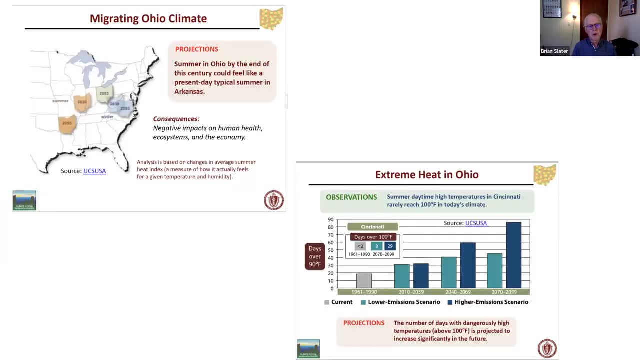 a lot on uh on on what kind of emissions targets we can meet, um, if, if we we just kind of look at this, you know, in an overall way, i think this is quite a a sort of useful way to think about what can happen or or what might be the extremes. uh. so if we think about uh, uh, forests and farms and 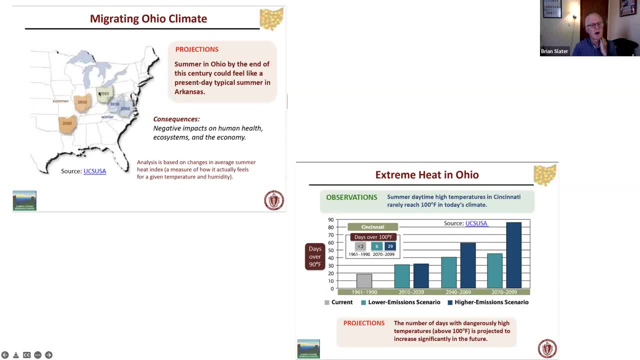 gardens. uh, you know what kind of conditions we have in ohio for our, uh, uh, the northern part of the deciduous forests zone. uh, we're going to be much more, uh, like arkansas, probably later in the century, so you can see the kinds of summer conditions that we're going to have. 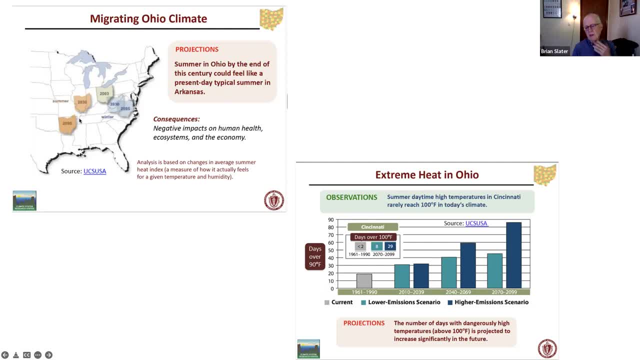 and uh, and then the winter conditions might be more like, uh, the mid-atlantic, and again these you know, no one knows, uh, and i'm not claiming anything more than just uh showing what some models are are showing, but we, we, we know, as well as the seasonal changes that will have extremes, uh, and 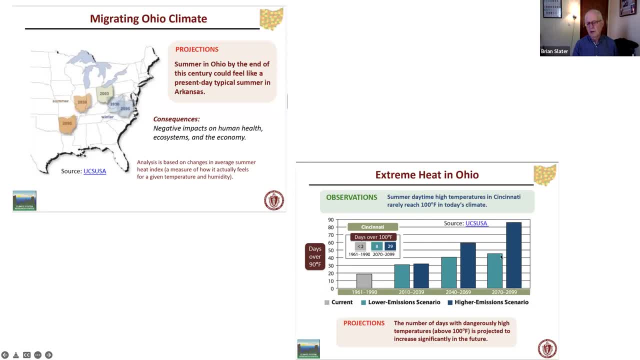 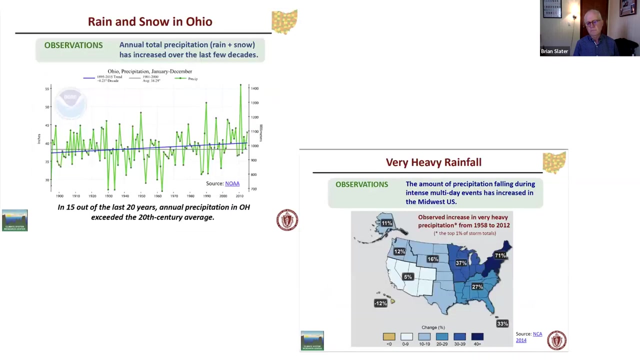 so we we expect that uh dependent on uh the the atmospheric greenhouse gases that we may have uh hot days, uh very hot days in in the future in our summers, and that's going to influence soil development and the relationship between soils, plants and microorganisms um rainfall uh similar. 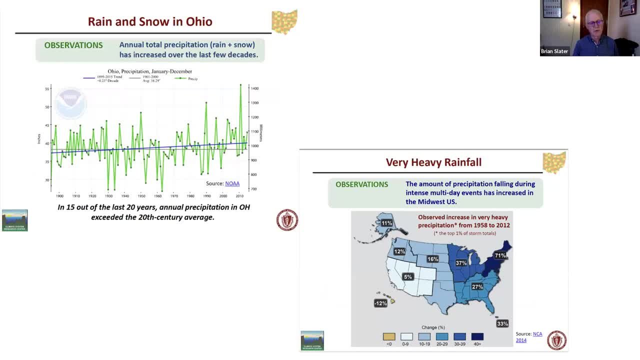 effects: uh, 15 of the last 20 years. this was up until 2015, i think, but precipitation had somewhat increased. uh, but probably more important in terms of influences on the soil, uh, heavy precipitation, uh, you know the top one percent of storms that create most soil erosion, for example? uh, those 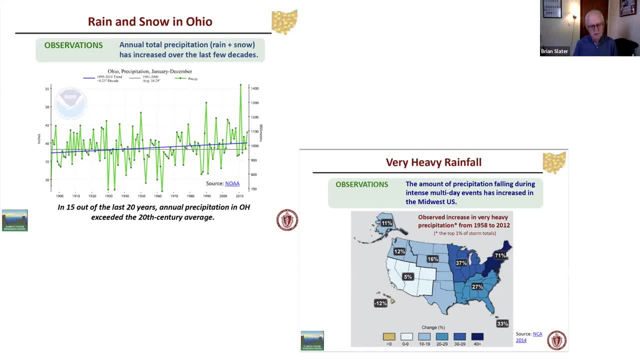 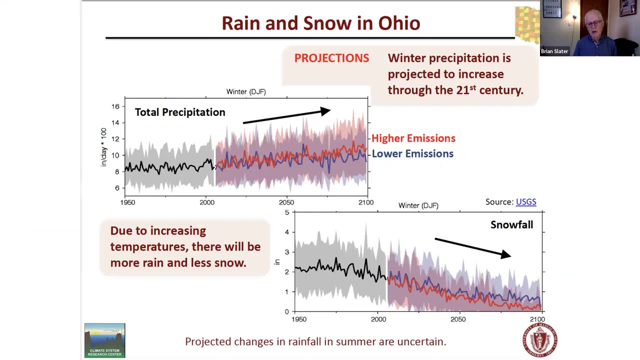 kinds of events are definitely increasing and will continue to increase. so, uh, uh, we will have probably cooler, moisture, uh, winters to some extent, um, uh, but our snowfall may go down again. these are just some model ideas that may influence how our soils develop. um, i won't spend more time. 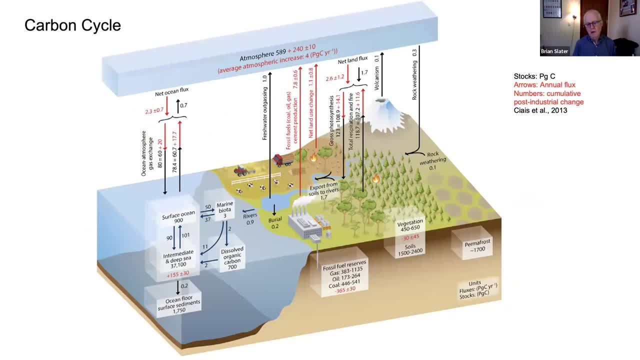 on that. we've all seen that kind of ad nauseum, but i did want to uh, since i talked about what general effects uh climate have on soils. uh, just put it in the context of the kind of changes that we may see. well, this all brings us back to soil's role in the carbon cycle. uh, so this work from uh. 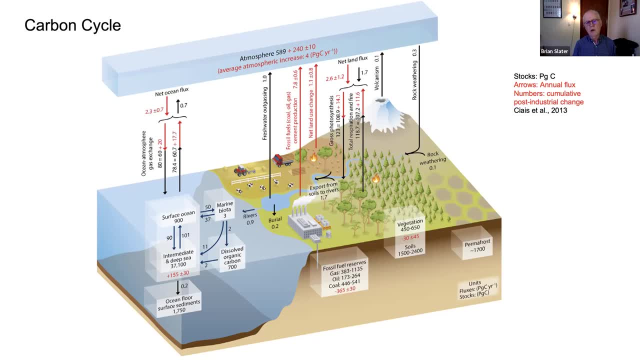 the uh, the ipcc, uh work, um, uh, this is not the most recent data, but i think it. you know the these numbers are at least generally uh accepted, um, for how much uh carbon is moving and being stored in various parts of the environment. so, uh, i just wanted to point out a few parts of 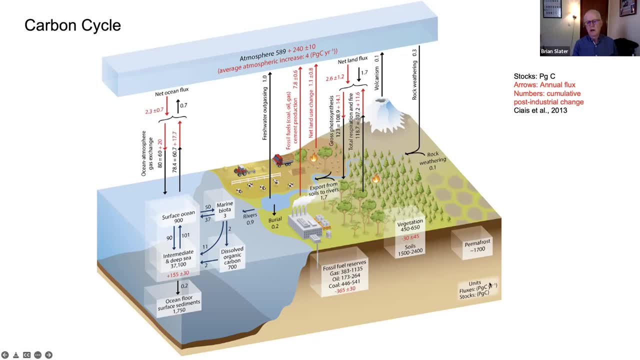 the carbon cycle literature important to us, uh, and so these numbers are in in in petagrams. uh, it's very hard to wrap our minds, uh, our brains, around how much that is, but if we think about billions of tons of of carbon, uh, that's probably a little bit more relatable than. 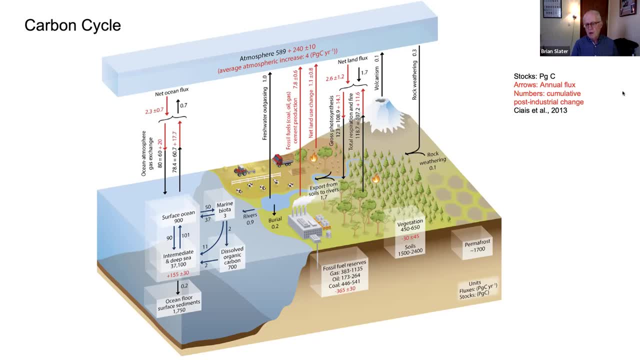 than the standard international unit of petagrams. but we we we can see here uh that we know uh or you know. various estimates uh you know are averaging about 2000 pg uh of long-term carbon. uh, organic carbon is is stored in soils. so these box numbers uh give the amount uh of of the stock. 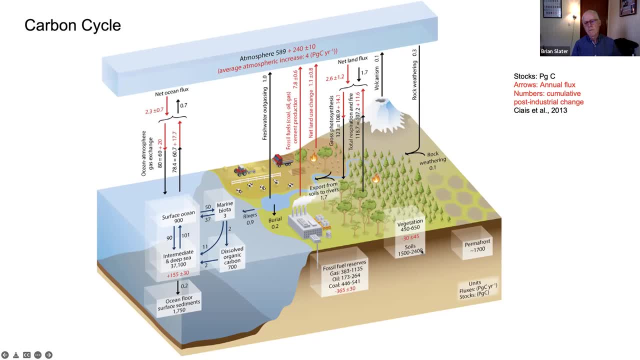 or the amount of stored carbon. we can see, then, that soils- the organic carbon in soils, on an average across our planet, globally, is significantly higher than that stored in the above-ground biomass or even the total biomass of vegetation. We can see that it's also significantly higher, at least three times as high- as the amount of carbon in the. 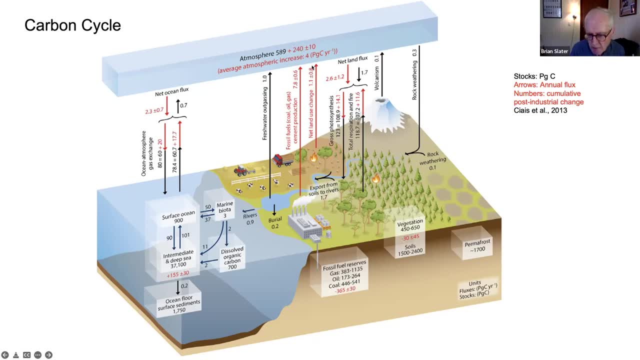 atmosphere. So that's the significant thing: to remember that soils are the most important terrestrial solid. you know, in terms of the landmass, Soils are the most important sink for carbon, But we also need to be aware of the range of these numbers and the fluxes. 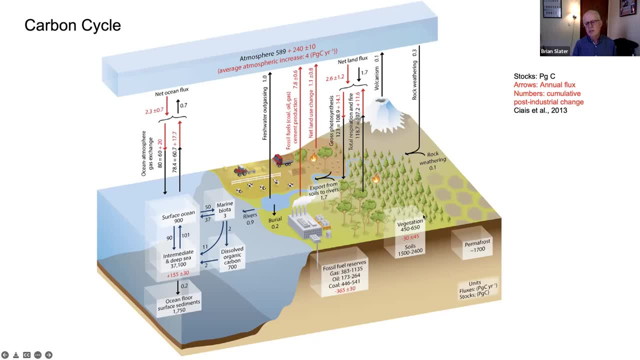 That much. you know how much is being removed in a given year And, depending on where we are and measurements, you know we may be losing every year in some places 30 pg, or we may actually be gaining carbon, depending on where we are and how this is. 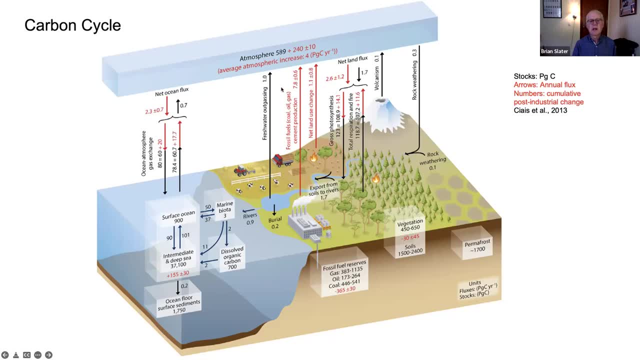 measured. That puts in context how much is being generated into the atmosphere From the burning of fossil fuels. So the fluxes from soil are significantly higher than those of fossil fuel use. And this is what drives our conclusion, as soil scientists and others involved in this, that we may have important influence over what happens in the global. 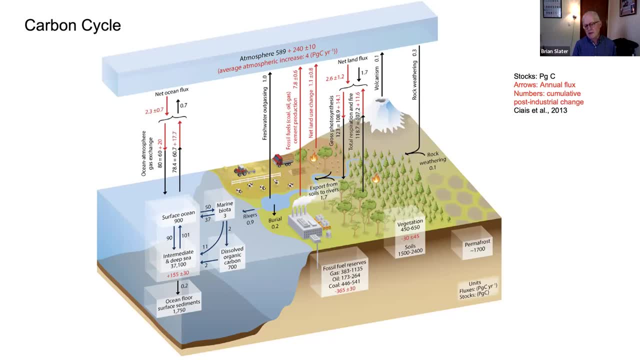 carbon cycle by what we do with soils. you know, if we can maximize, we can minimize the flux and maximize the storage. obviously that will have a very strong influence. The same thing, of course, goes for above ground biomass. So if we can, 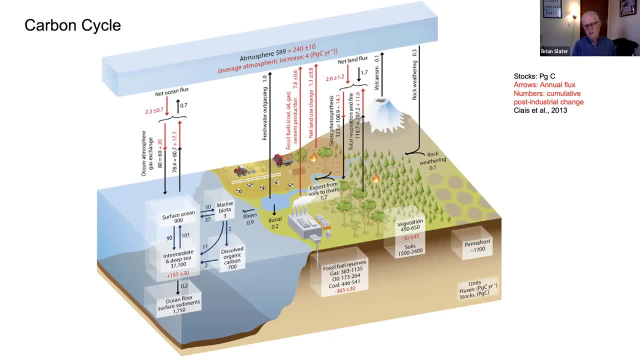 store carbon. as woodland owners, as foresters, we want to do that too. So this is not an either or situation. There's no competition here, but we do need to recognize this important issue with soils. And so what's important, You know, are they annual fluxes, Right, But also this long term flux. 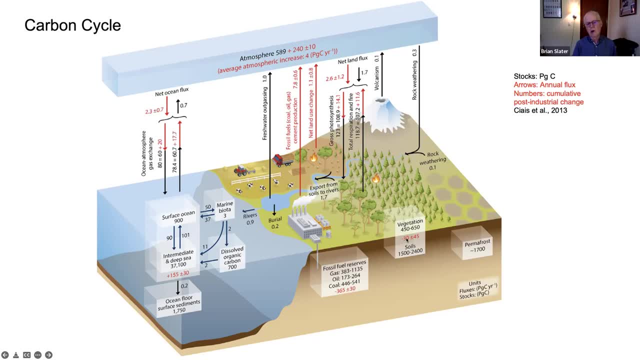 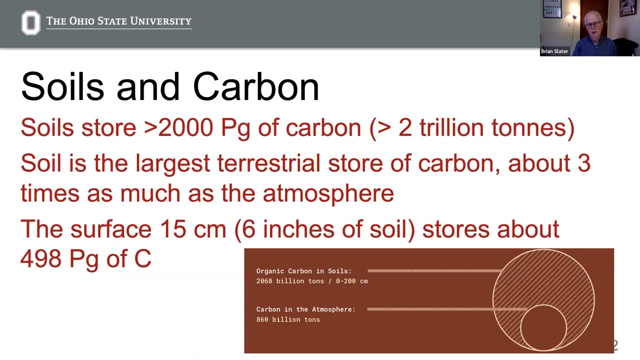 And so large amounts of carbon have been lost from soil over time, mostly due to agriculture. So that's the kind of global carbon cycle, Putting this more in context of soils. So We believe that soils store about, or more than 2,000 PG of carbon. 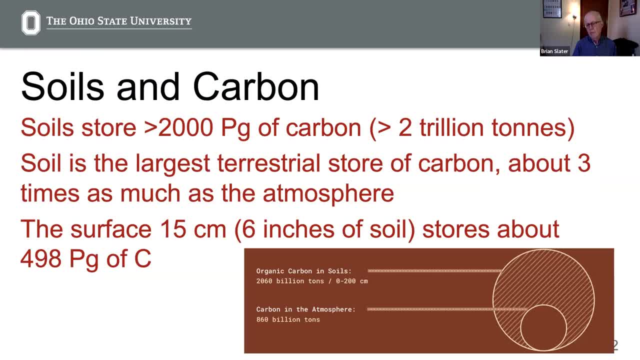 in the organic fraction, or more than 2 trillion tonnes, or 2,000 billion tonnes of carbon. It's a lot. So we can see, then, that soil is the largest terrestrial store of carbon, you know, roughly three times as much as the atmosphere. 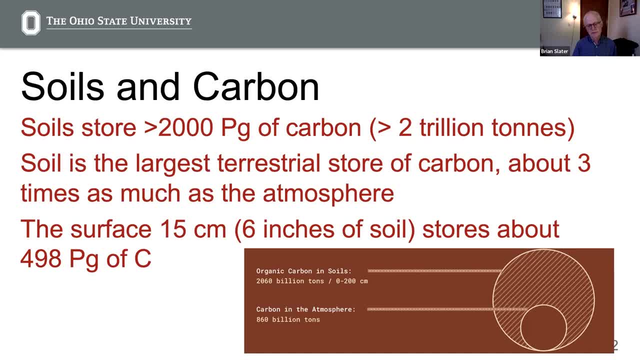 If we think about the top part of the soil, the top six inches or 15 centimetres or so of the soil, it's got a lot of carbon. So I'd like to point out how much is in the surface, because this is the part that we have the highest influence over. 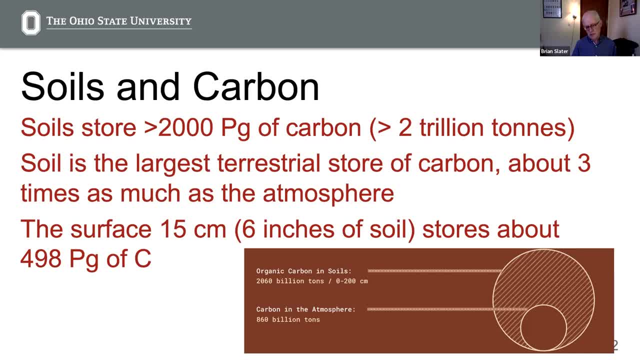 You know we manage the soil at the surface. mostly. We add materials to soils, We take it away. That's the part of the soil that's most influenced by erosion and land management. So that's a lot of carbon and this can change fairly quickly. 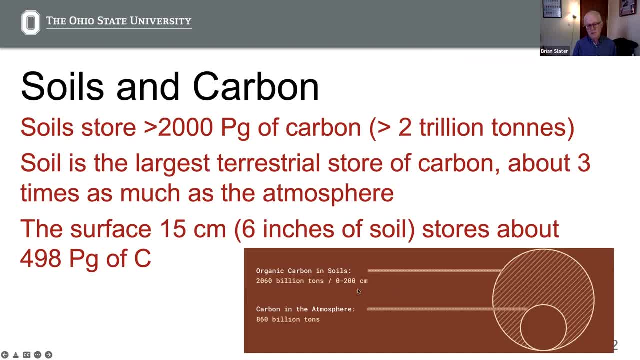 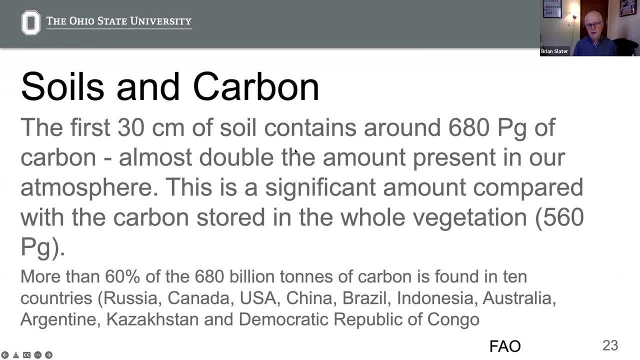 Okay, so you can see again, in the top 200 centimetres we have a lot more carbon than in the atmosphere. So the first 30 centimetres of soil contains about that much, almost a double amount. You know again, these numbers are very dependent. 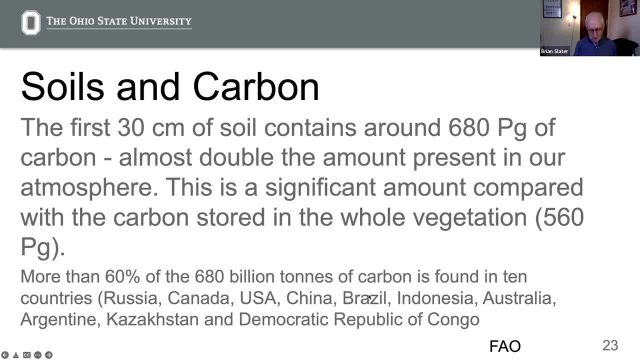 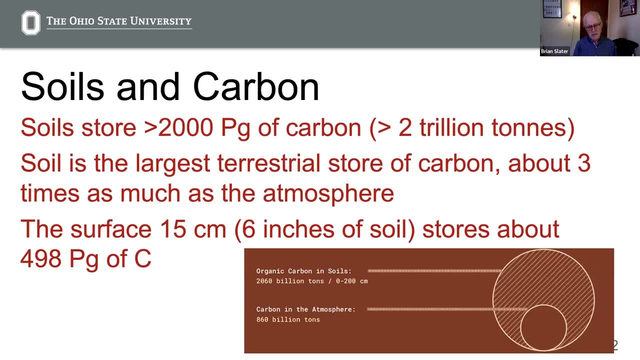 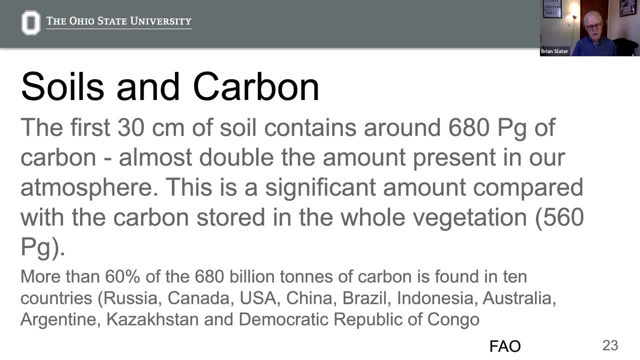 on where you get these numbers. So this information here is from the International Soil Resource Information Centre, which is an agency in Western Europe, and this is from the Food and Agriculture Organisation of the United Nations. So more than 60% of the carbon, more than 60% of stored carbon, 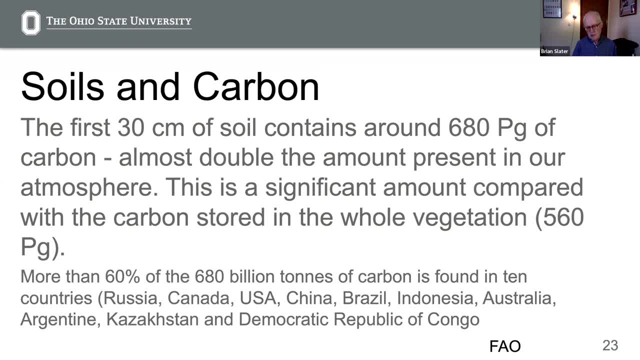 in the top 30 centimetres, And so you can see that what you're seeing here in the top 30 centimetres is in only a relatively few large countries: Russia, Canada, the United States, China, Brazil, Indonesia, Australia and some others. 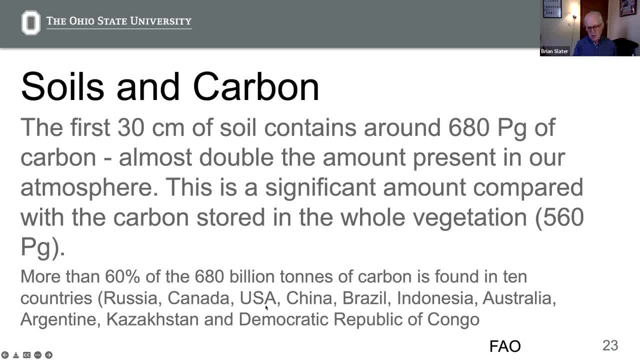 And you will recognise many of these as major agricultural and forest products producers in the world, And so these are where. these are the places where most carbon is stored, and they're also the places where you know there's a lot of carbon. 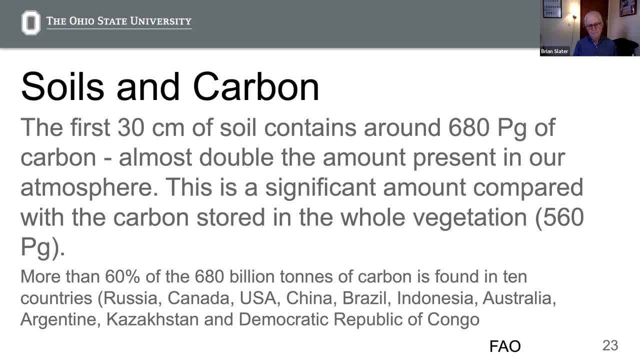 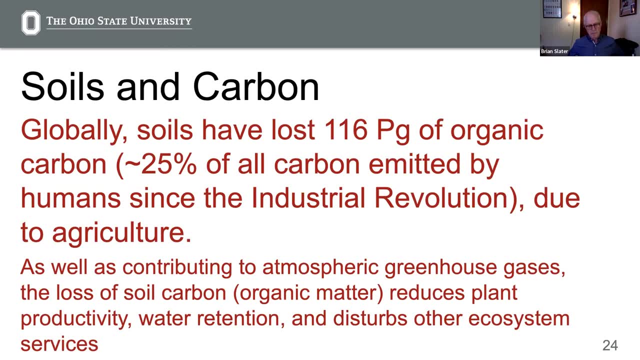 most carbon is influenced. um, so let's talk about the fluxes uh in the post-industrial period. mostly the period are, you know, here in terms of soils? we're mostly talking about, uh, modern agriculture. uh, about 25 of all the carbon that's been emitted, uh emitted into the atmosphere, came 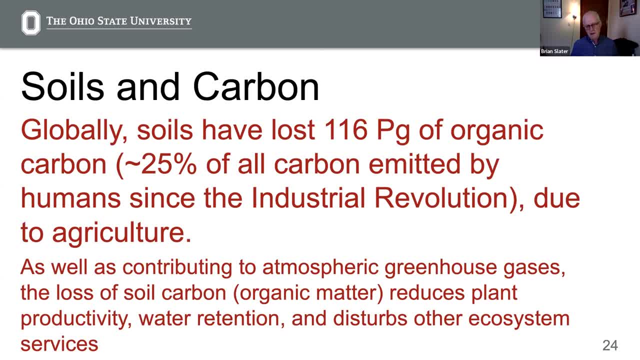 from uh came from agriculture, uh, and that's that's very significant. um, so what we do in the future in agriculture, uh, to a large extent will have a very, uh big influence on how much carbon dioxide and other greenhouse gases are in the atmosphere. uh, but it's, it's. 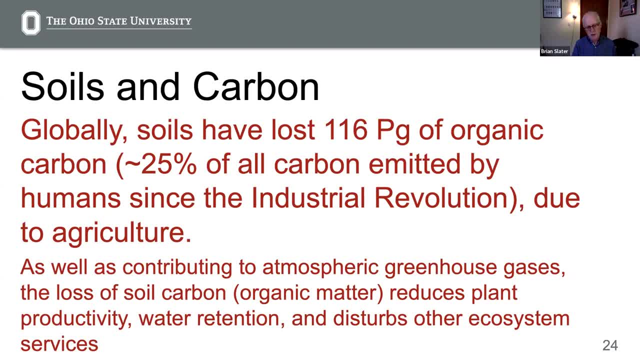 it's a kind of uh complex and and uh and multi-level story here, because as well as contributing to atmospheric greenhouse gases the lot, this loss of carbon of organic matter from agriculture and other managed soils reduces plant productivity because soil carbon is involved in nutrient cycling and water movement in soils, in water storage in soils, in the relationship between 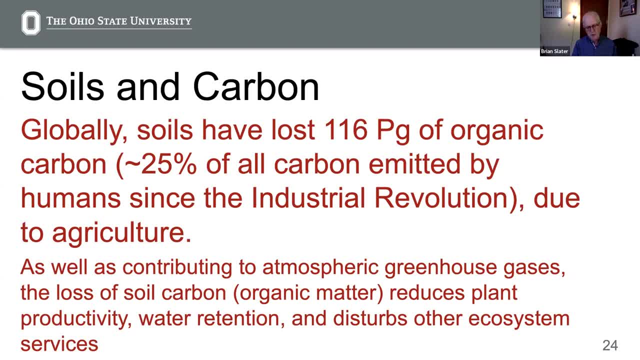 contribute in Messiah. 될ock, yo-yono and those in fortress management are going to be going back to how it used to want to waste�� nossas umism. uh, mild major. so the big bias thing that's going to play from now to next year is: 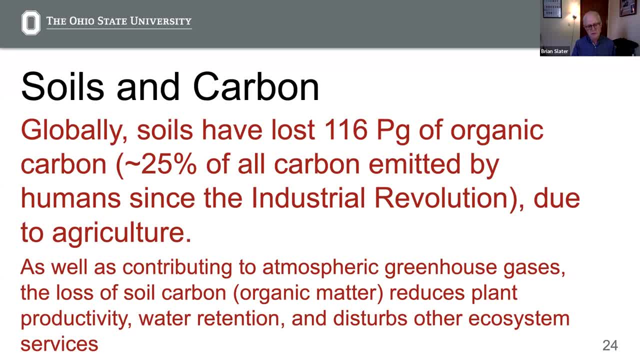 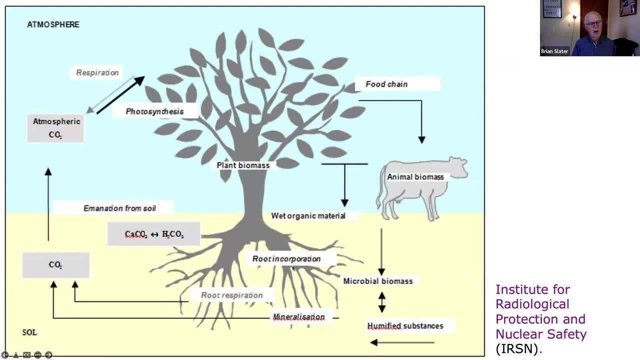 a much r highlighter for the global Wyoming, arid climate And so, you know, bringing the carbon cycle down to the more local level. here we can see how carbon gets into soil via breakdown of the plant biomass and its incorporation into the soil as organic matter. incorporation of senescent plant roots. But we also get losses. Organisms respire to some extent and most of these will produce carbon dioxide in that respiration process. There are also going to be effects from organisms on the inorganic carbon components. So if we add acids to the soil, via the breakdown of organic matter these will dissolve some of this calcium carbonate in soils and also generate carbon dioxide. 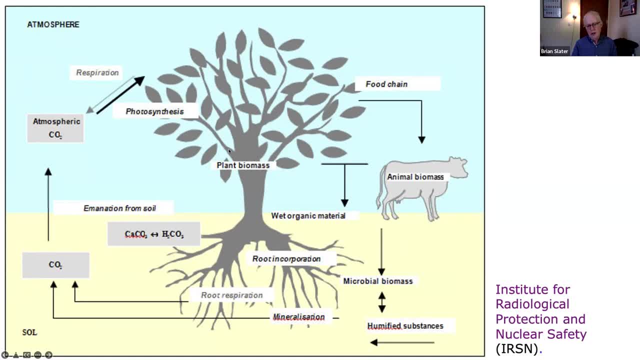 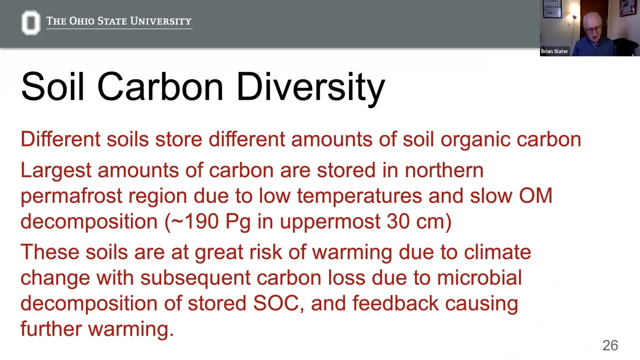 So this is the kind of local carbon cycle That influences the amount of carbon in the soil and, to some extent, atmospheric carbon. But it's not simple and it's highly spatially variable. Different soils store different amounts of soil organic carbon. The largest amounts of carbon in soils are stored in the northern permafrost region due to low temperatures and slow organic matter decomposition and generally wet soil. 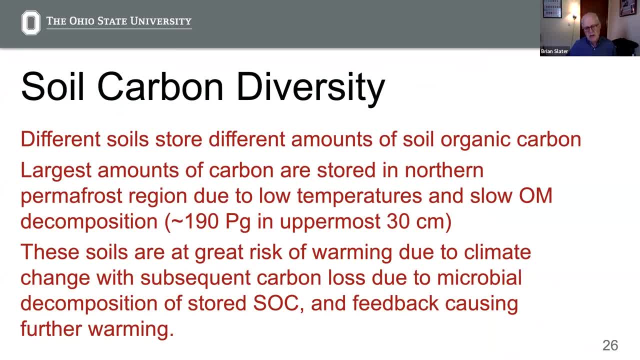 So. So if we look to the permafrost areas, the tundra, that's where the largest amounts of carbon are stored: 190 PG just in those permafrosted soils. So that's a you know. a third of you know. almost a third of all stored carbon in soils is in those permafrosted soils. 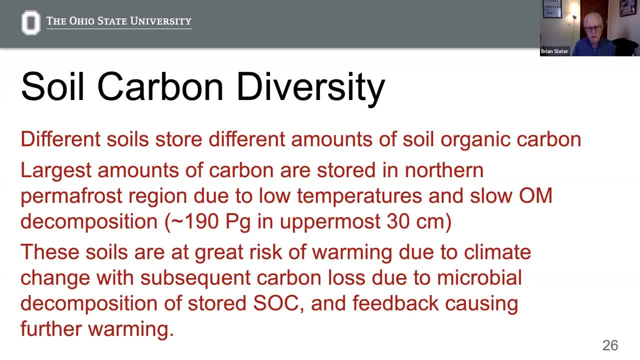 This is, of course, a very big concern because these soils- Soils- are at great risk of warming due to global climate change. as these soils warm up, carbon loss due to microbial decomposition and even melting of some of that permafrost will liberate some of that stored organic carbon. that will then send more greenhouse gases into the atmosphere, creating a strong feedback loop. 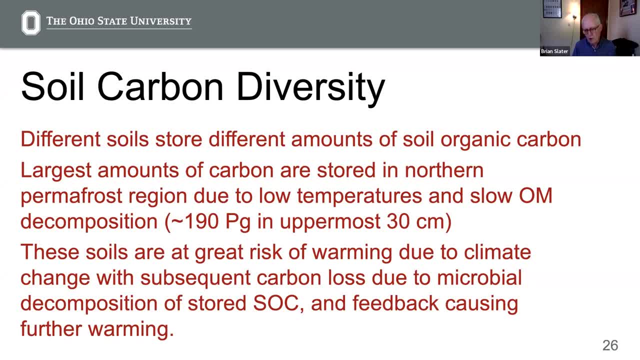 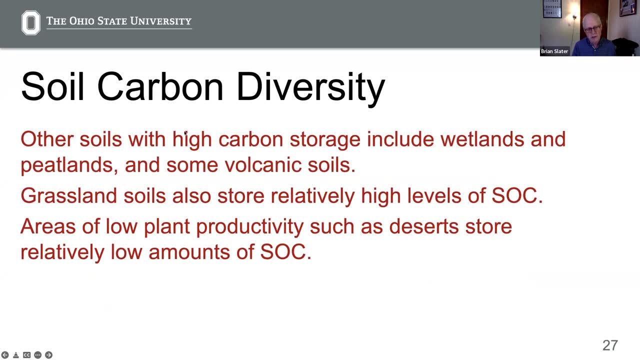 And this is one of the main concerns for for long term climate change- That as those soils warm, they're going to even Generate more carbon into the atmosphere and then create this feedback loop. Other soils that have high carbon storage include wetlands and peatlands and some areas of volcanic soils in various parts of the world. 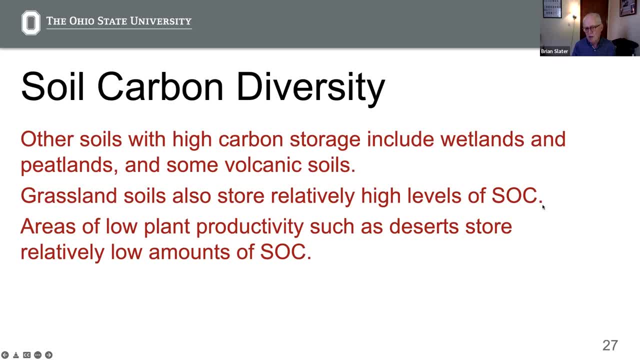 Typically grassland soils store relatively high levels of carbon because of the below ground biomass associated with grasses and and forbs in those ecosystems. So if you want to get more Carbon into the soil long term, you know grasslands may be a good choice in some parts of, in some ecosystems. 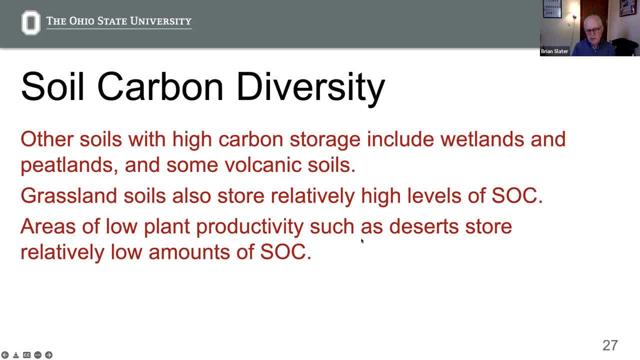 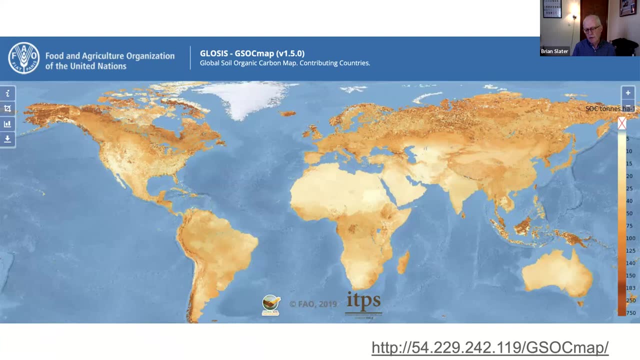 Particularly perennial grasslands. areas of low plant productivity are places where we have relatively small amounts of carbon, such as deserts. So this is a relatively recent mapping application On soil Soil carbon. given given time, I don't think I was going to get into this, but you can. 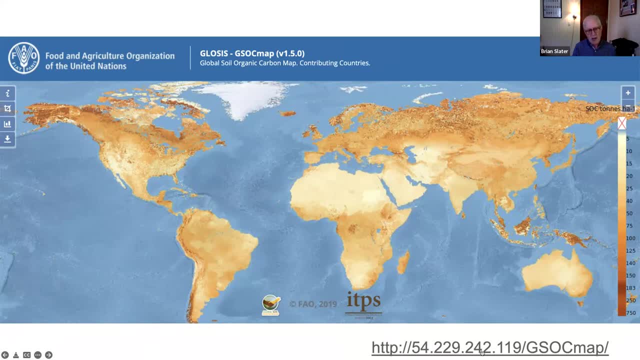 You can go to this application and map Global estimates of carbon. it's, it's, it's on a fairly detailed scale, so we could go to Ohio here And and see the amounts of Of carbon stocks, of stored carbon in in various places. so it's, it's, it's an interesting application to look at, just generally, looking at these overall map here. 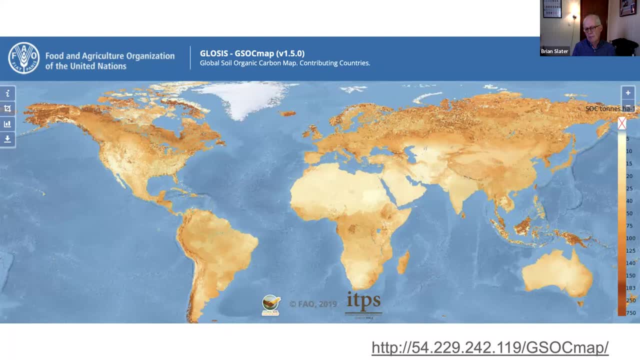 We can see the places where larger amounts of soil carbon is stored. so, as I mentioned, the permafrosted regions, the tundra across Alaska and northern Canada, through northern Europe, northern Russia, Siberia- We have very large amounts of of carbon and stored on on on a broad scale, places like Iceland. 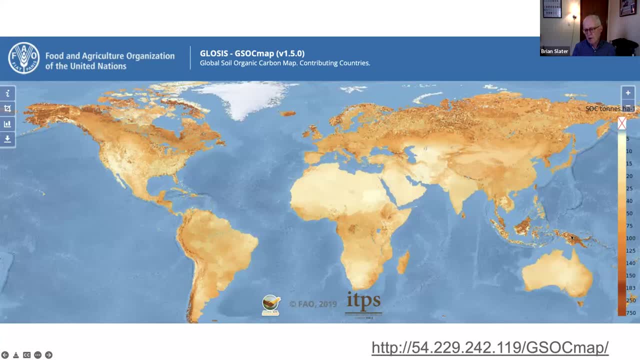 Through some parts of the, The volcanic areas of the tropics, like Indonesia, we have got tropical rainforest and and volcanic soils. these are also areas of high carbon storage. The world's grasslands Come next, so wetlands and and permafrosted areas have the highest levels. but if we look at the large areas of the world's grasslands here we can see through here to set steps of Central Asia. 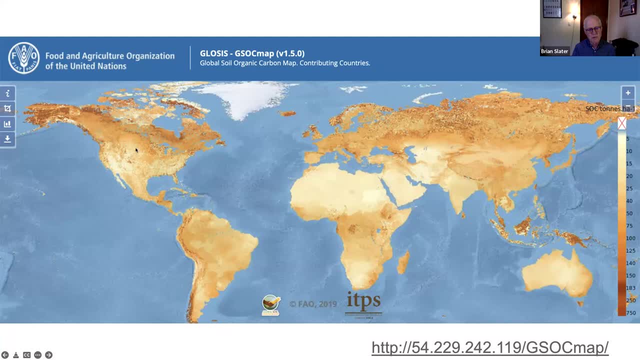 The Pampas in South America. the prairies of the United States have moderately high levels of stored carbon, And then the low areas of carbon stored in soils include the world's deserts, large areas in Australia and the Sahel in Africa, the Middle East and western parts of North America. 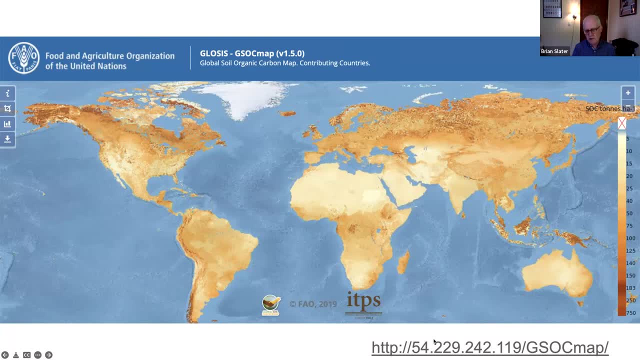 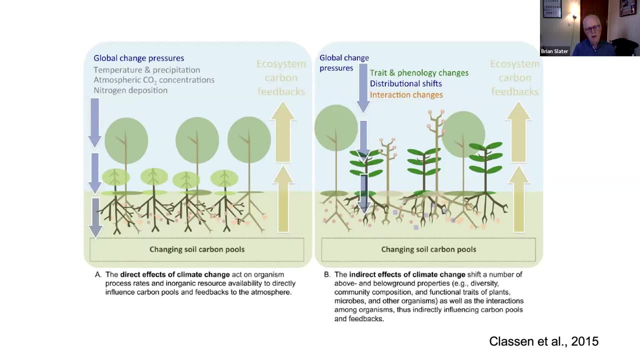 So it's. it's worthwhile having a look at this if you want to get a sense of where carbon exists. So let's talk about a little bit about the effects on soil, microbial and plant relationships. These diagrams come for a very interesting paper by class and 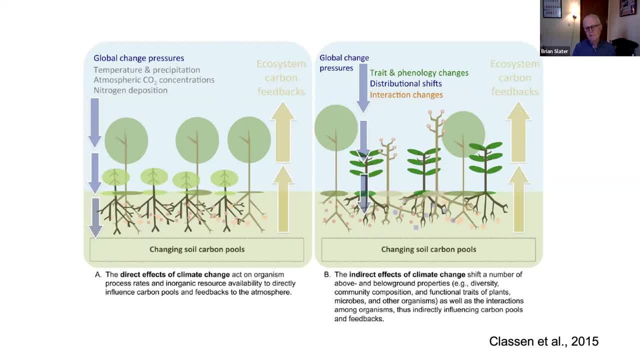 That talks about what is known about the influences of climate change on on microbial and plant relationships in the soil. so we can, we can understand that we have these various carbon feedbacks and then There will be A Direct effect then on organisms that live in on the soil as climate changes. so direct effects on climate act as. 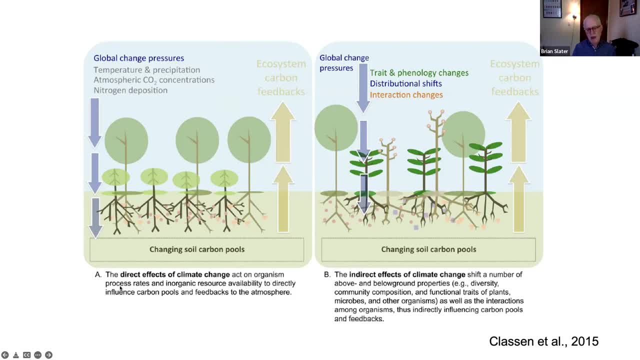 Act directly on organism processes and the amount of organic matter that's added and lost, and also influences on inorganic carbon as well, to directly move carbon either into the soil or back into the atmosphere. So, depending on what happens with climate change- changes in temperature and precipitation, concentrations of atmospheric carbon dioxide and even the deposition of nitrogen, that will change productivity. 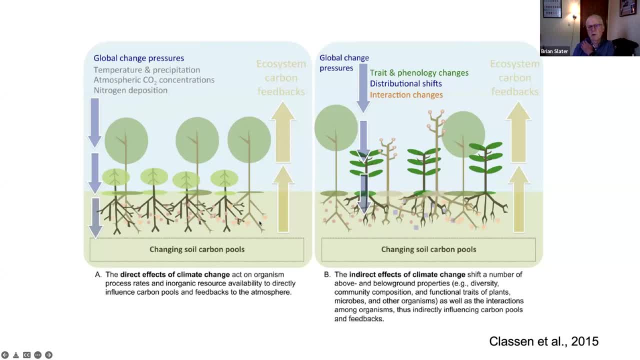 And the influences of various organisms, but it's extremely complex. But as well as that, we have indirect effects regarding organisms. this might include A shift in the above ground and below ground property. A shift in the above ground and below ground property. 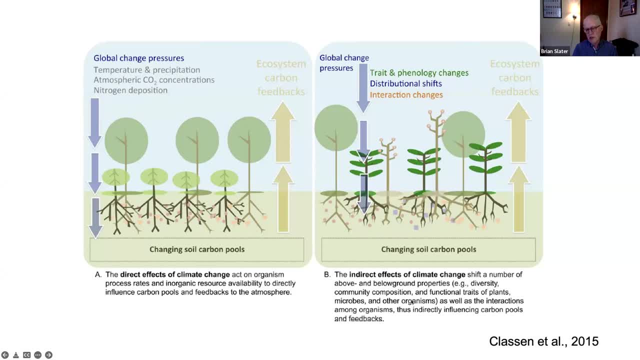 A shift in the above ground and below ground property, A shift in the above ground and below ground properties. So diversity, a composition of plant and microorganism communities, the different kinds of plants and what functions they perform in the environment, and the same goes for microbes and other organisms in the soil. 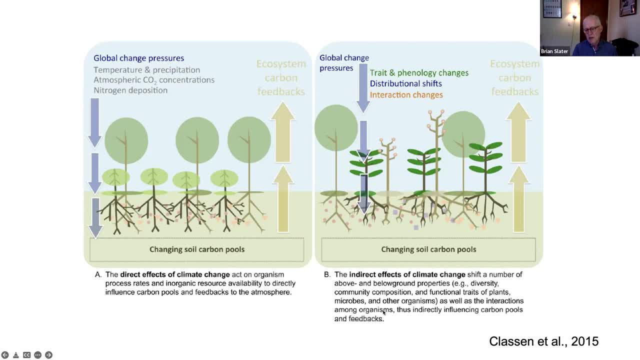 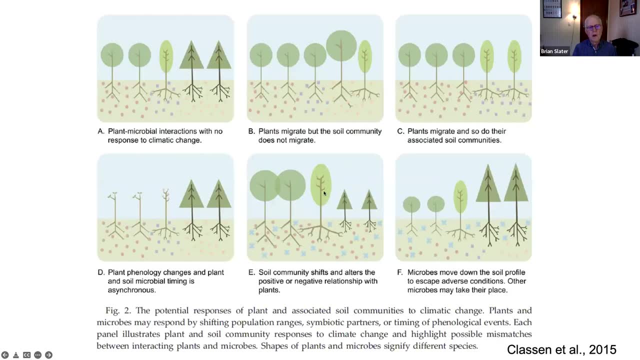 And interactions among these are going to indirectly influence carbon pools and feedbacks. So we could expect a very broad range of responses from the complex community of plants and microorganisms in and on soils. So this could range from those that have absolutely no response to climate change to various ways in which microorganisms and plants are going to be affected. 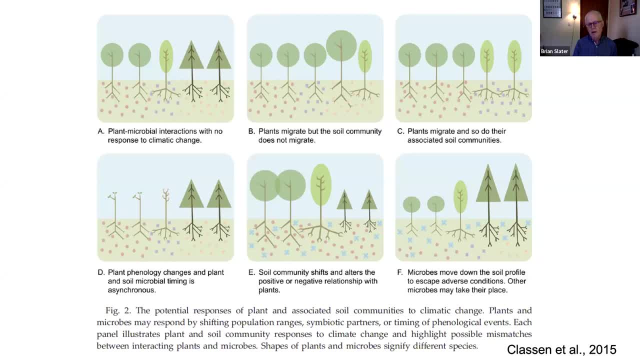 So we might have a change in the kinds of plants that can grow. So imagine if our summer temperatures are more like the southern states of the United States. then there's going to be some changes, for example to plant understory and definite changes. 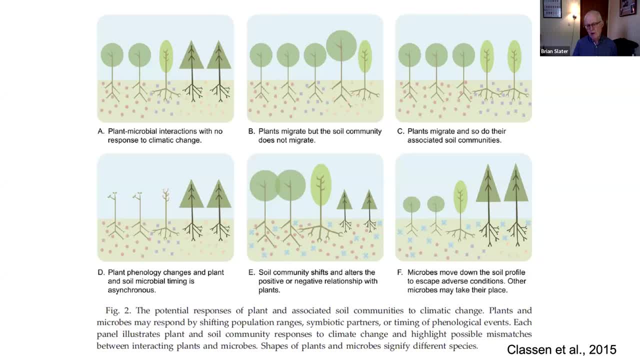 long term. So we may have migration of species and some change to species composition, at least in terms of vegetation, But we might not have much change in potential, in particular soil microbial communities. But it may be that microbial communities as well as the plants that they are associated with- and this seems much more likely in many cases because there will be a response in both the plant and microorganism communities- 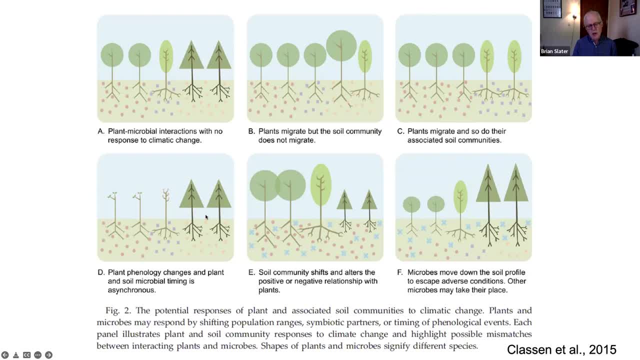 We may have major changes in the phenology of plants as well. We may change our forest types even, or even our soil types, Even our understory types. Their form and shape will also change And that may change seasonal effects on microorganisms. 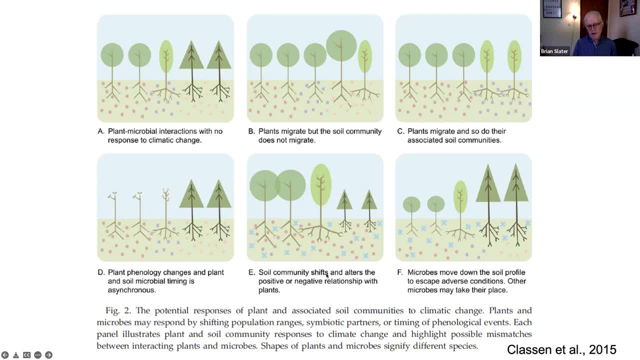 There may be effects that relate to positive and negative relationships between plants and microorganisms. If we think about things like mycorrhizae and nitrogen fixing organisms related to nitrogen fixation in plant roots or pre-living in the soil, these kind of community shifts may also happen. 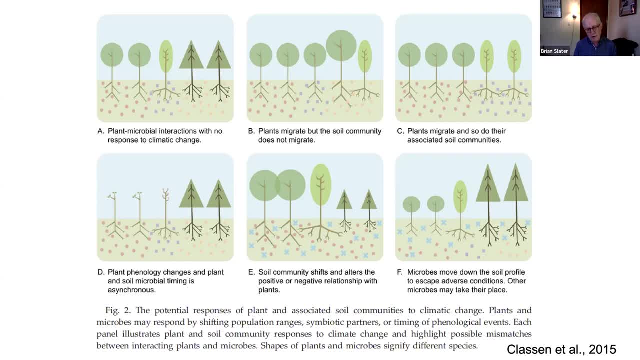 You know, we may get warmer temperatures, different plants might grow different legumes, for example, different kinds of trees that may be nitrogen fixes. So many different kinds of effects will happen And then we may have adverse conditions. So we have very hot surface soils that might create downward movement or downshifts. 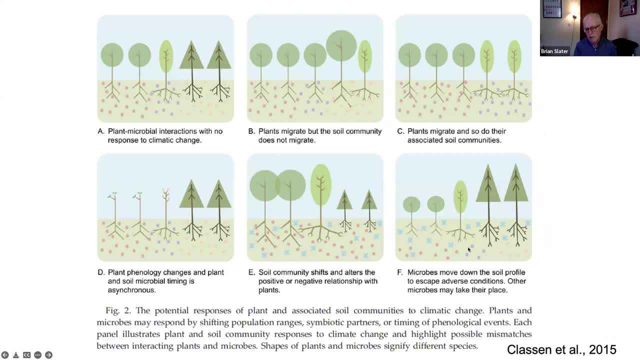 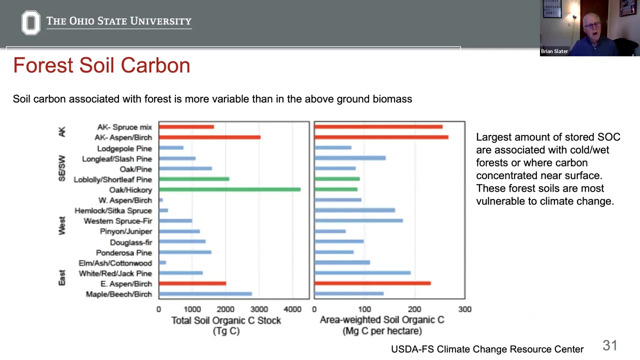 Downshifts spatially are microorganism communities in soil. So you know, again, these things are kind of general ideas about what may happen with climate change And long-term studies are going to have to be established to understand the actual numbers and changes that we see there. 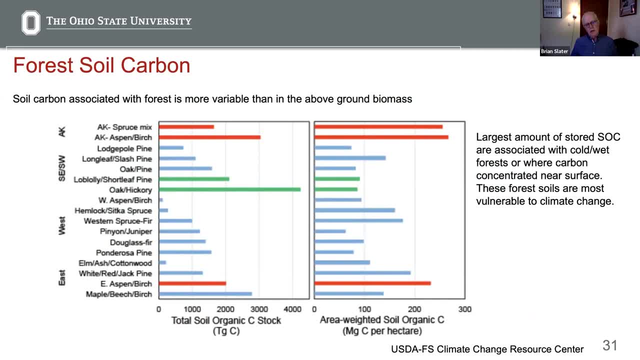 I do want to bring this back a little bit Related to forests. So one thing that we know from various studies is that the soil carbon below ground is variable, more variable than the above ground biomass in time and space. So there are various aspects of this. 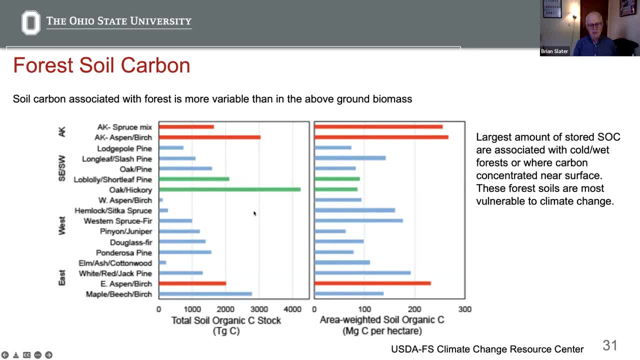 You know we can see that total carbon stocks are the highest in oak-hickory forests- Sorry about that, Highest in oak-hickory forests, But that's largely a result of the area, of those kinds of forests We can see. if we look at the area weighted, this tells us what kinds of environments or forest systems. 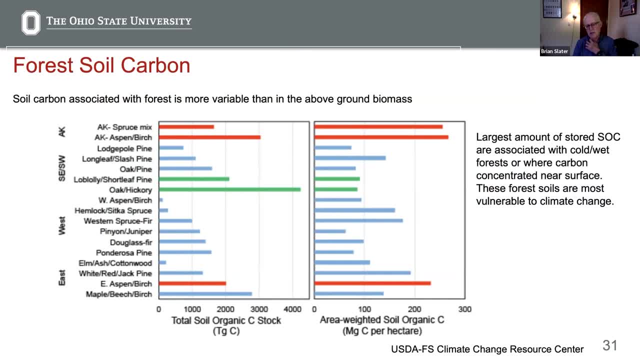 Or vegetation soil systems where we have the largest amounts of stored carbon. So these are mostly associated with wet forests, wetlands and also areas where we might have relatively cold conditions. So cold, wet forests are where carbon is also concentrated closer to the surface. 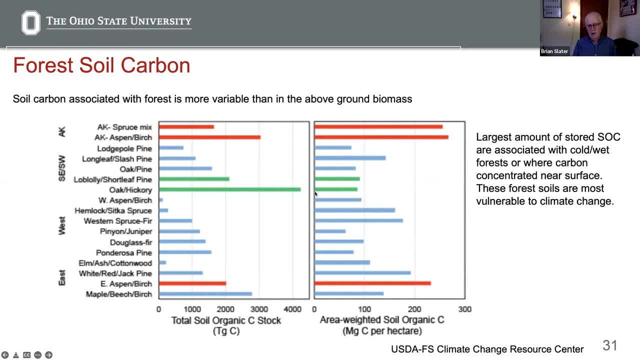 In oak-hickory forests, for example, and more deciduous forests, we tend to get more distribution of carbon down the soil profile and less towards the surface. We have fewer over-horizons or duff layers and more active distribution down the soil profile. 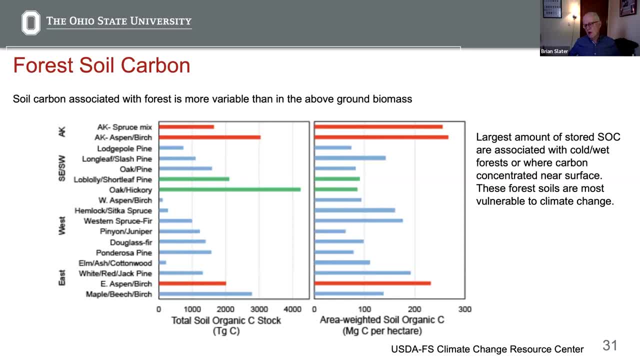 So this might have an interaction with climate change, for example. So surface soils are going to be colder, They're going to be far more vulnerable to changes in temperature and moisture, for example, And so you know the kinds of forests where we have more carbon concentrated towards the surface. those situations may be much more vulnerable to climate change. 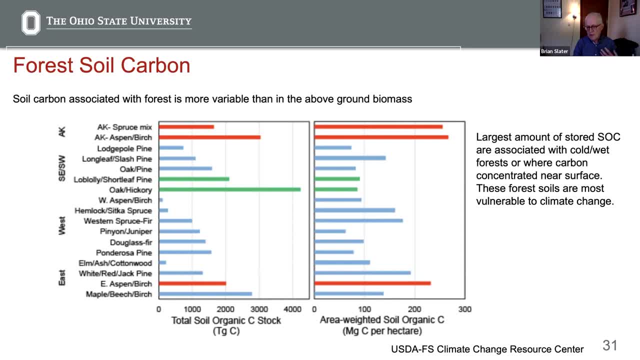 And another corollary of that might be that there may be more long-term potential for increasing soil carbon, And so you know the kinds of forests where we have more carbon concentrated towards the surface. those situations may be much more vulnerable to climate change. 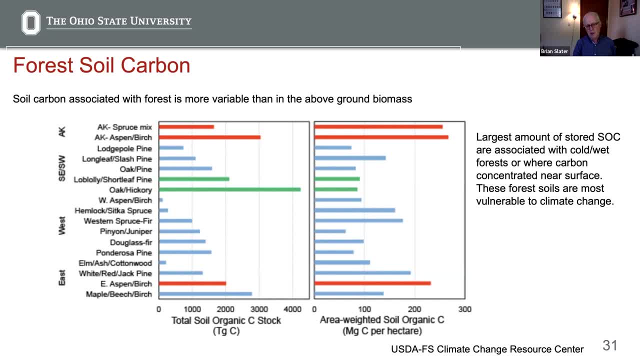 And so you know, there may be more long-term potential for increasing soil carbon in moderate carbon storage systems that have a large area and distribute that carbon more generally into the soil profile, such as the oak-hickory forests. So just some kind of broad generalisations there. 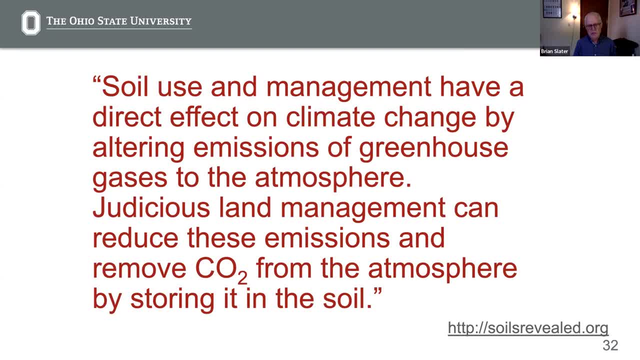 So to kind of bring this to a conclusion, to some extent, soil use and management definitely have a direct effect. onará. So to kind of bring this to a conclusion, to some extent soil use and management definitely have a direct effect. oná have a direct effect on climate change as well as soils being affected by climate change. 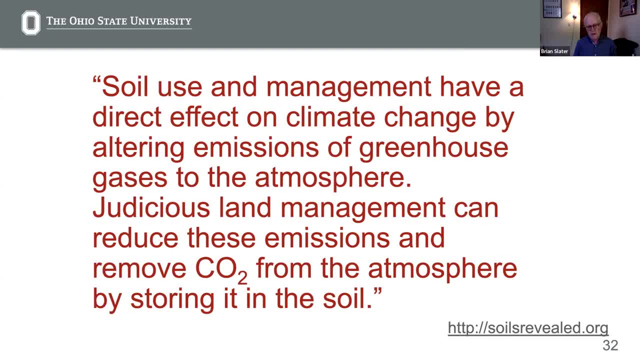 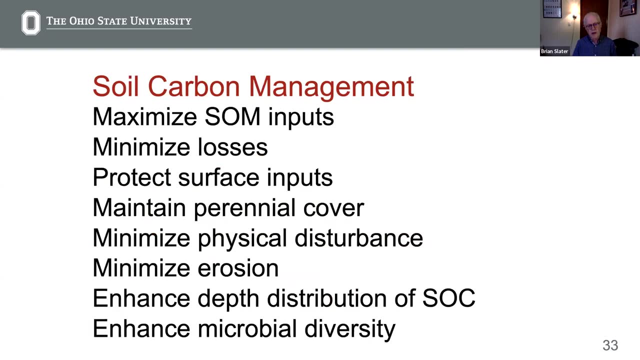 but soils do this by altering the emissions of greenhouse gases to the atmosphere, and we can influence this via our judicious land management. so I'll just spend a couple of minutes talking about what broad general options are for managing that. So if we think about this there, 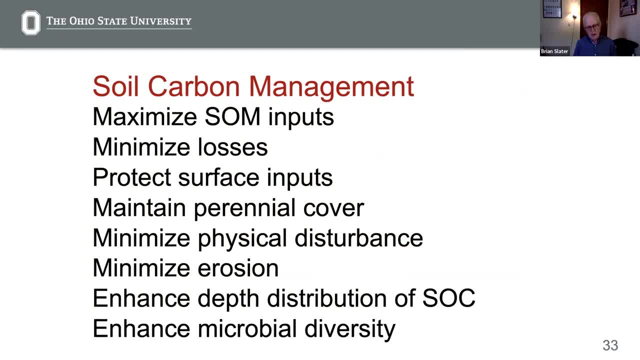 are so many different things to do and this could be the subject of a whole series of webinars. I think you know how we could manage soil carbon to maximize storage and minimize losses in all kinds of ecosystems, including forest ecosystems, but basically anything that we can do. 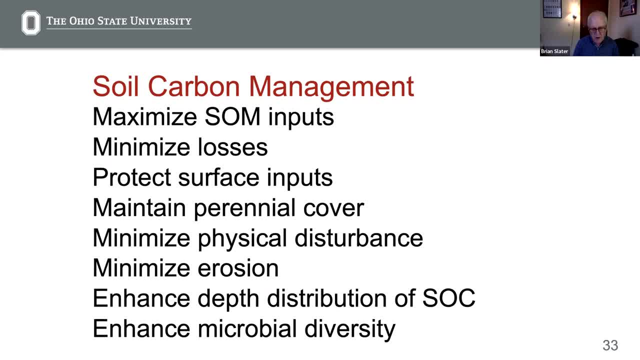 to maximize input. so productivity is a very important part of this puzzle, but it's it's much more complex than that, because soil organic matter is a balance between imports and losses, so in order to maintain and increase soil carbon, we need to minimize losses as well as maximize imports, and in some cases, minimizing losses can be just as important. 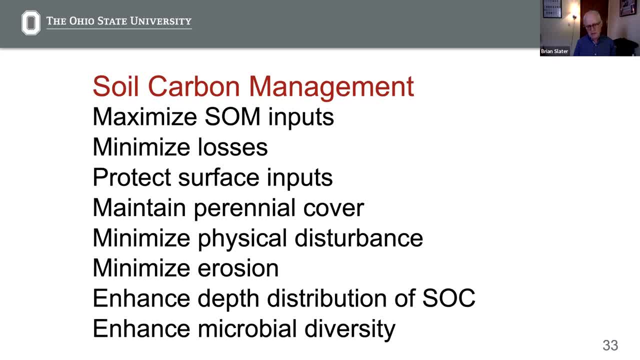 this means protecting what we add to the surface and protecting those high concentrations of carbon near the surface of soils. this can be done through maintaining cover over the soil right through the year. this would be true in agriculture and forest systems- anything we can do to maintain some kind of cover. 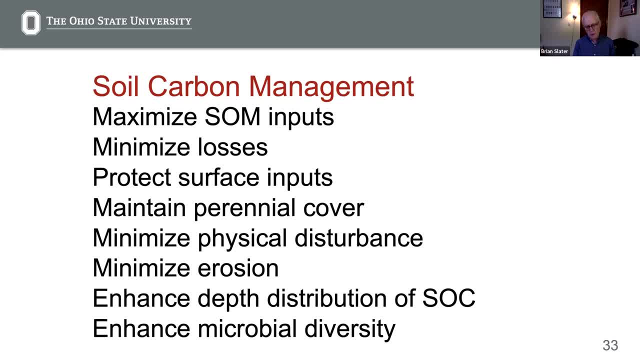 whether it's standing living, cover cover crops or agroforestry systems or anything we can do to keep perennials developing perennial plants that we can harvest rather than than annuals. minimizing soil disturbance is also a very important way that we can influence soil carbon and minimizing erosion. erosion remains. 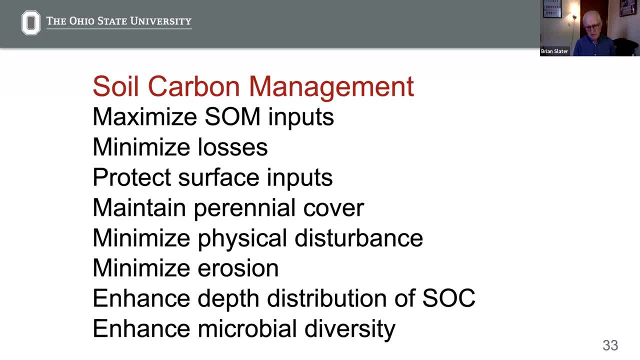 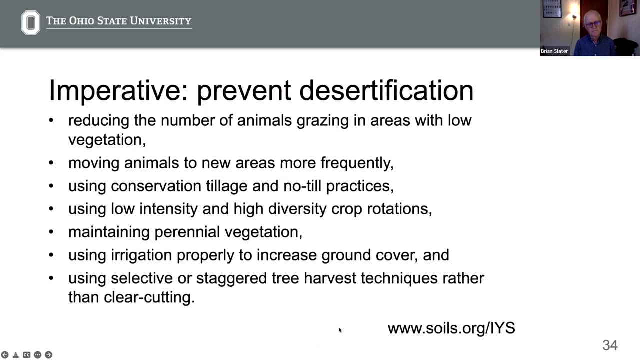 a major way that carbon is lost and redistributed in the environment, anything we can do to enhance this depth distribution, because concentrated carbon towards the surface is most vulnerable, and, finally, what we can do to enhance the balance of different organisms in soils to enhance the microbial diversity. one of the major ways uh that we can have the largest influence uh is preventing. 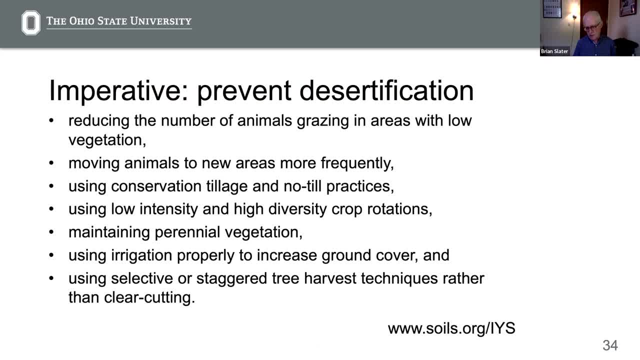 uh, the formation of of deserts. so we soil. we saw that the world's desert store the least amount of carbon and those deserts are increasing. jury to change due to changes in the environment. as we have climate change. uh, we will see the? uh the effects on of those changes would be more obvious. 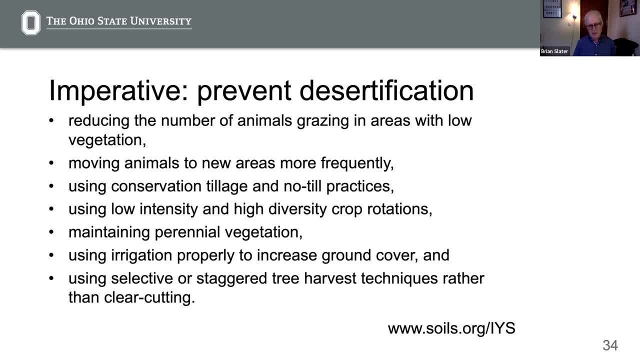 than ever. some of the changes have to be made, however, as we work through the climate change changes in increasing the propensity of desertification. So preventing those things is going to be absolutely fundamental, and this is where the biggest effects on soil carbon can be affected: Reducing the number of grazing animals, moving animals to new areas more. 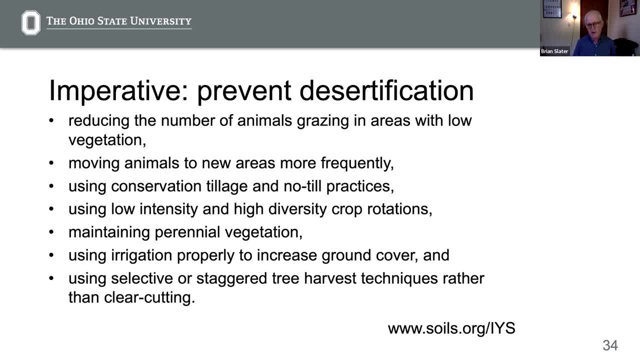 frequently using conservation, tillage and no-till practices in agriculture, using low-intensity, high-diversity crop rotations, agroforestry, for example, maintaining perennial vegetation, forest cover, woodland cover and agroforestry- all kinds of ways of having perennial vegetation. 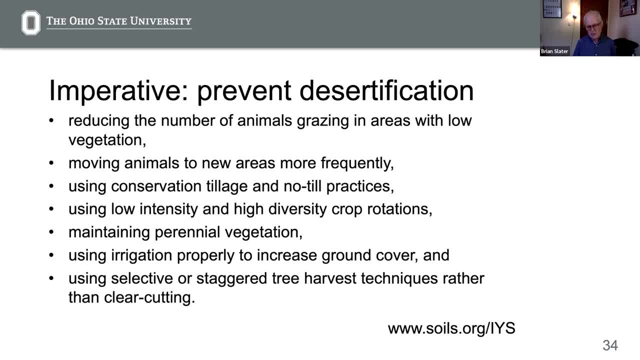 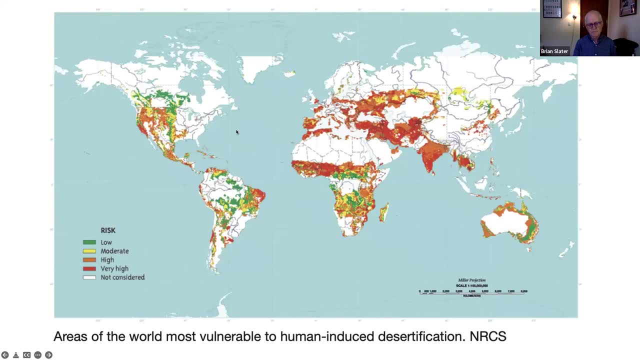 Increasing ground cover with irrigation using selective and staggered tree harvest techniques rather than clear cutting to maintain perennial cover and living organisms in the soil. All of these things we've heard about many times. I won't go into more detail today. So this map. 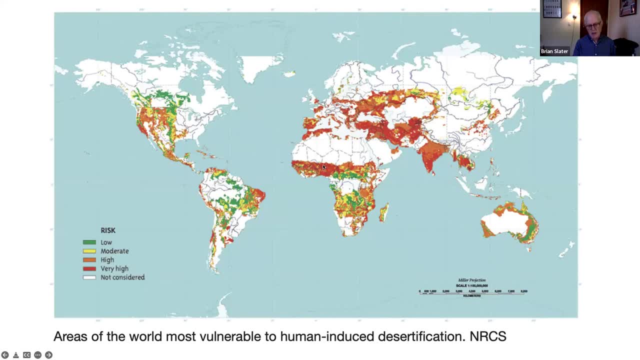 related to the others I've shown, indicates the areas that are now most vulnerable to desertification, to major changes in soil that will result in very much lower levels of vegetation growth, very much lower levels of soil carbon stocks and soil carbon storage long term, And so this is where there needs. 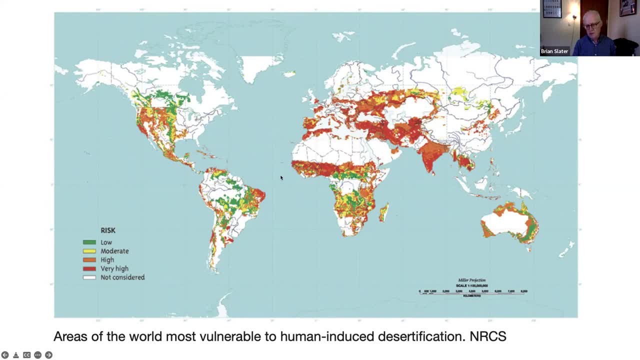 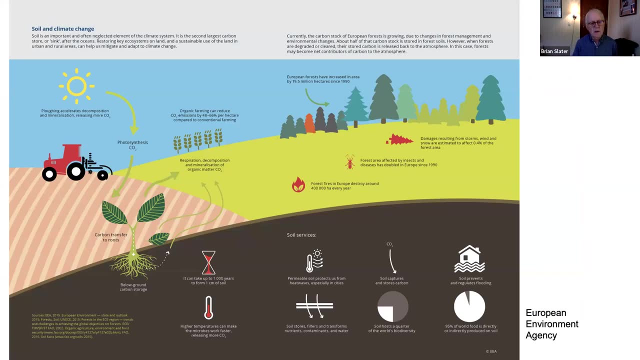 to be very, very strong action to maintain soil carbon levels. So this diagram from the European Environment Agency I think serves as a kind of summary for the things I've talked about related to soils and climate change. So just briefly looking at this, 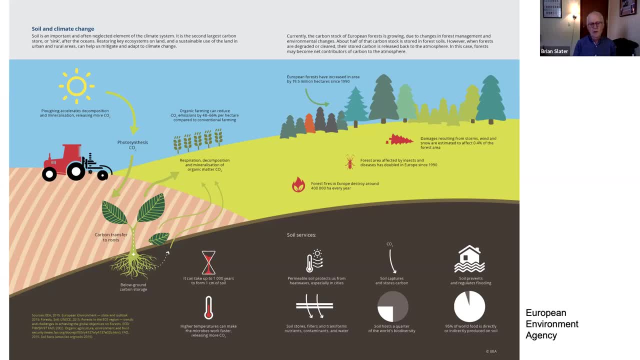 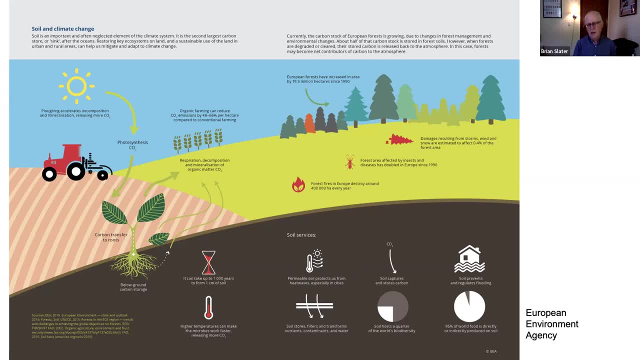 in the cities there Permeable material that has water and air and living organisms. So anything we can do to maintain that condition of soils will help us. Soil stores and fills insulting, transform nutrients, contaminants and water and carbon and living organisms And soil organic matter play a very important. 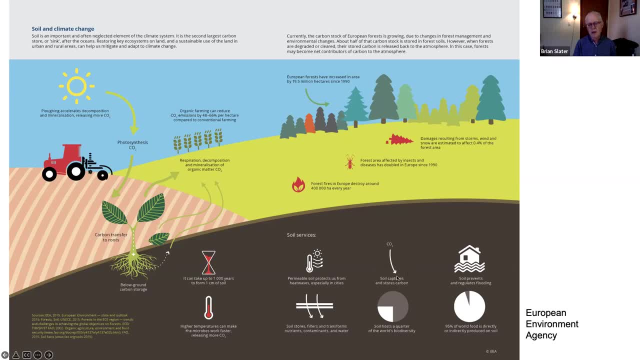 role in that Soil actually catches and stores carbon. Soil hosts one of the world's biodiversity. Soils influence water offsite, preventing and regulating flooding and, of course, provides 95% of the world's food supply, as well as forest products, pharmaceuticals and industrial products that are incredibly important to us. 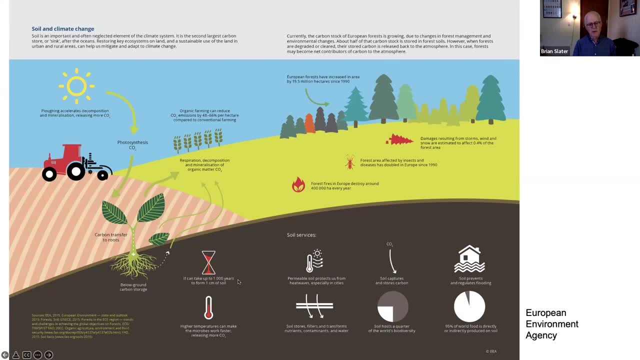 Soils form very, very slowly: between 100 to 1,000 years to form just one centimetre of soil And, as I mentioned, you know, in an afternoon we can lose all of it. Higher temperatures are going to be the key to the effects of climate change because they influence soil, microbial and plant communities and the BAPO. transpiration will increase and carbon dioxide and other greenhouse gases into the atmosphere are going to increase as temperatures go up. 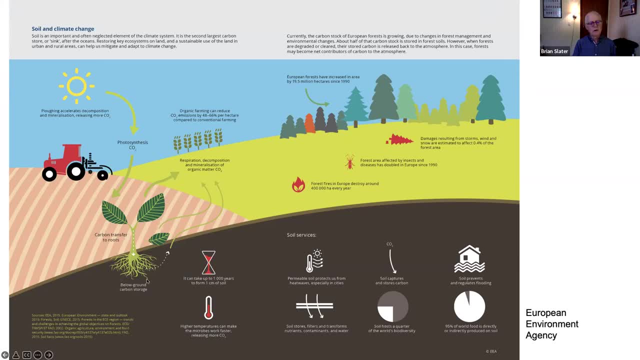 So this below ground Storage is critical. If we can maintain that, then we'll have a very, very strong influence on atmospheric carbon. This means minimal soil disturbance, so that we know. things like soil disturbance, ploughing and other influences on the soil increase decomposition, mineralisation rates, creating more carbon dioxide. 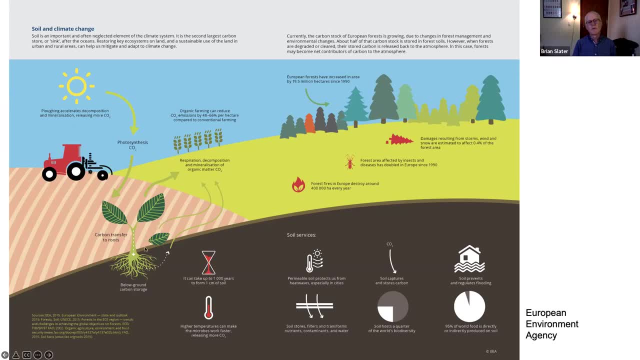 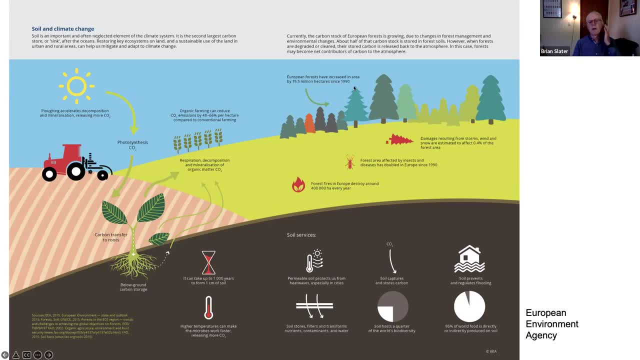 We may have sort of interruptions. Ladies and gentlemen, I can't입니다 if the You know, if it's it's, This allows us is an even more important. if I unlock that, if I unlock this urbic leaf, that is, I fecture like. 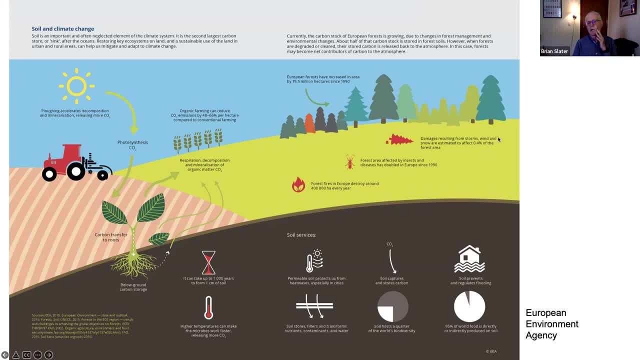 T it 也 sky head. It's important if it's, and things like that will also have long-term effects, as will insects, which are increasing across the world's forests, and also fire, So these are disincentives to production in forests. that will also influence soil carbon. So I'll stop now and we can open this up and I'm very 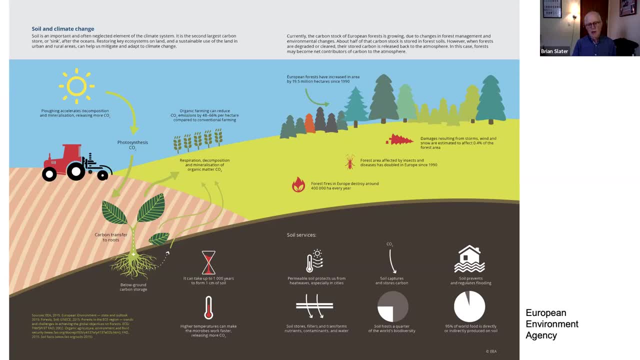 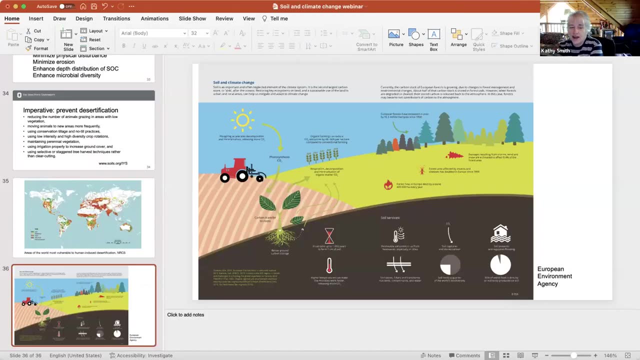 happy to be involved in a conversation and answer some questions. Thanks, Brian. I have to say you have some amazing graphics. I'm jealous. Well, I also have to say that many of these, of course you know I did not make, so you know I've. 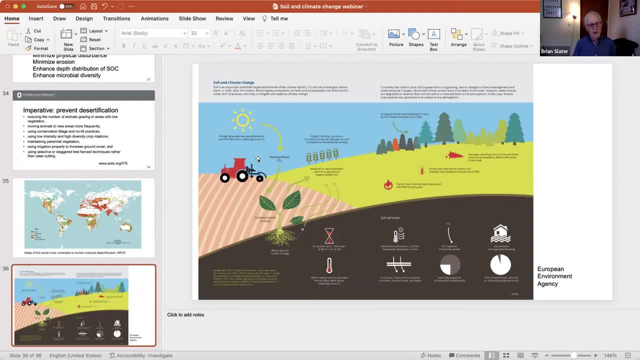 I will provide all of the sources for these, so, but I think it helps us to see these to gain an understanding of what's going on. Yeah, and, like I said, these graphics really do. I'm much more of a visual person, so when you have 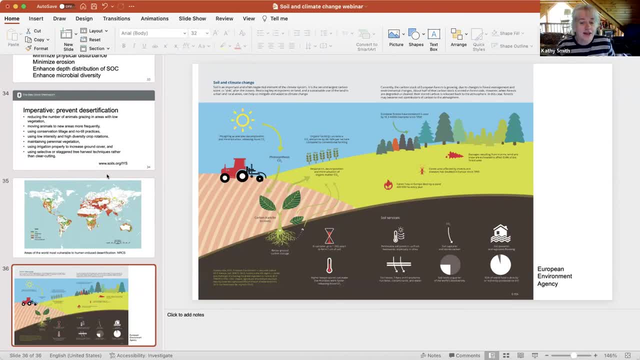 those kind of things. it certainly helps me put things in perspective. so I really appreciate that. I wish that on our forestry side we had some of those kind of graphics, but I think for us they're the same graphics we would have had in the past. 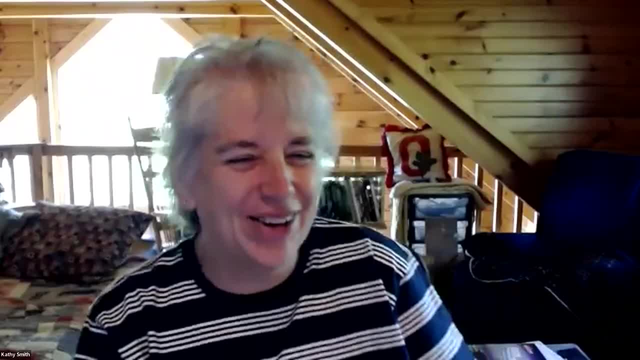 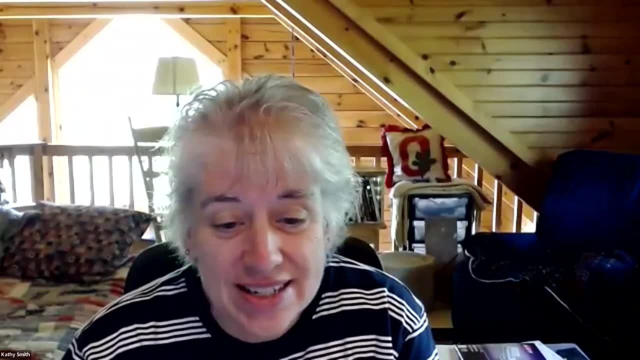 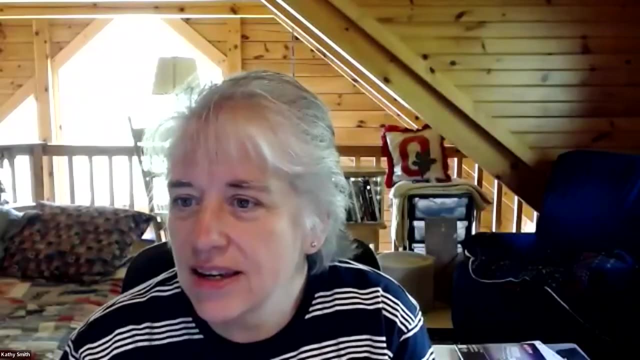 They're the same graphics we would have had in the past, have done 20, 30 years ago. They're not quite as snazzy, but awesome presentation. Thank you very much. And we do have some questions. Let's see here. Okay, So the first one is: Frank says in the: 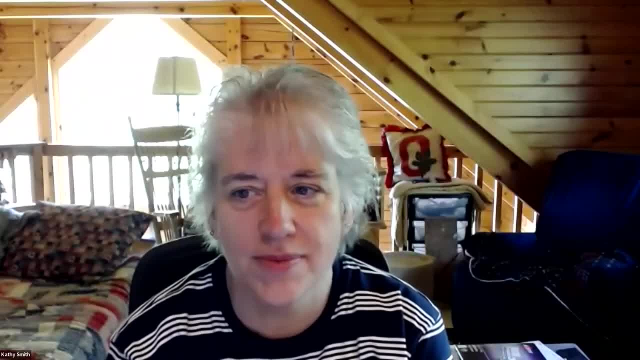 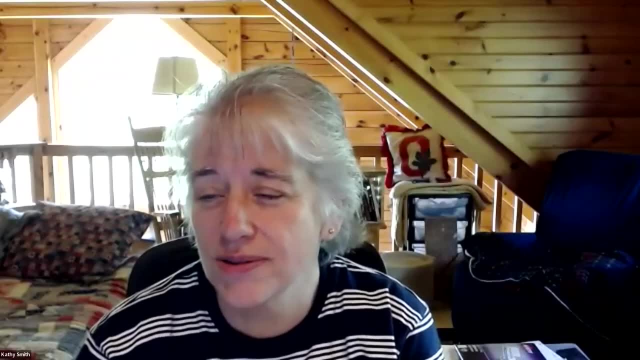 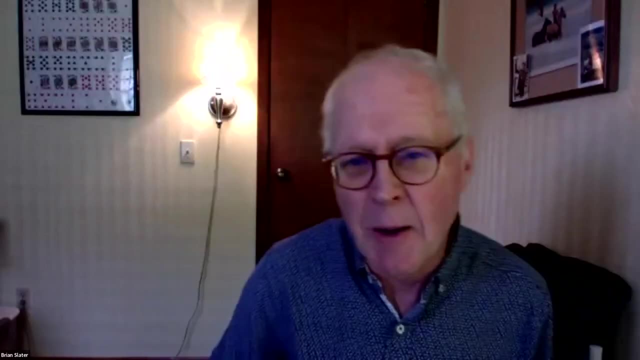 last 2000 years, there have been at least two periods of climate change: medieval warm period and little ice age. Do we know what these periods did to soils? That's a great question And it's something that really interests me And I what I'm going to do. 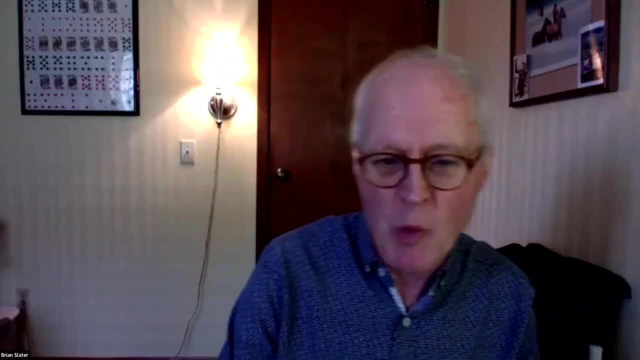 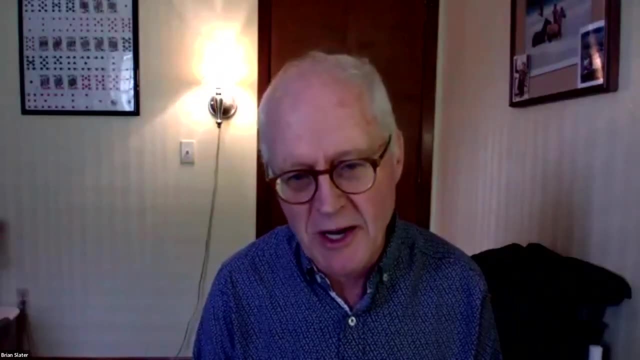 actually is just refer to one place where where I know we know something about this. Now, I am not an expert on those periods in Ohio or North America. I know a little bit about the climate change in Australia, but I'm not an expert on those periods, So I'm not going to go through. 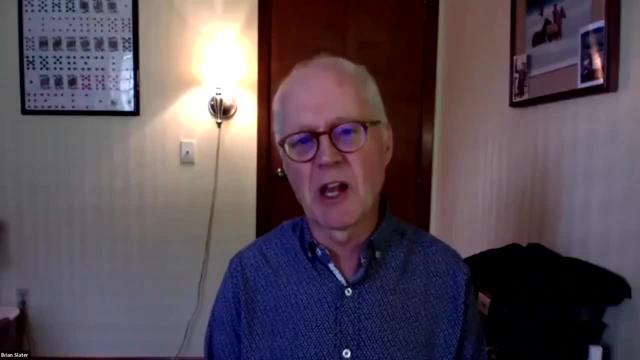 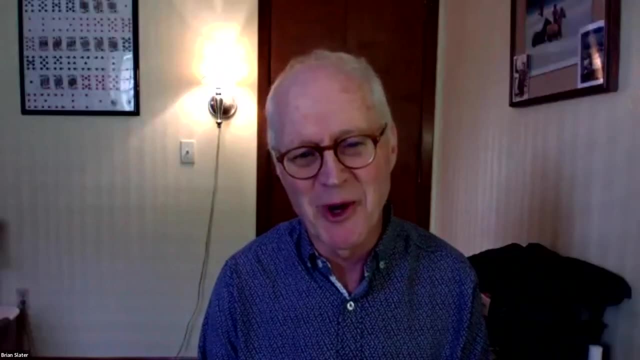 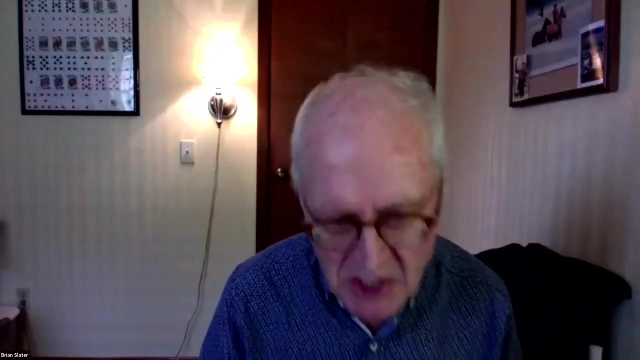 what happened in Australia, but those particular climate change periods were not really influential in Australia. believe it or not, You know, I you know there have been changes, but mostly in Australia there was a warming and drying happened over that period, So there wasn't a little ice age. 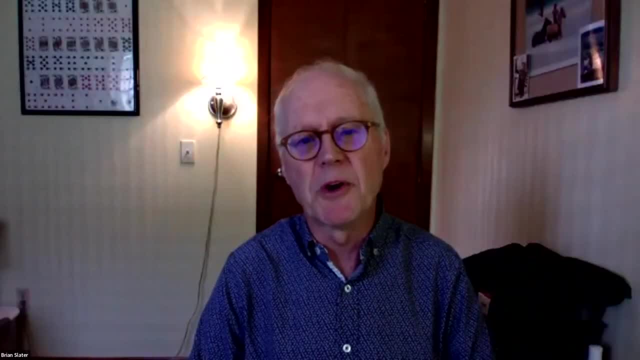 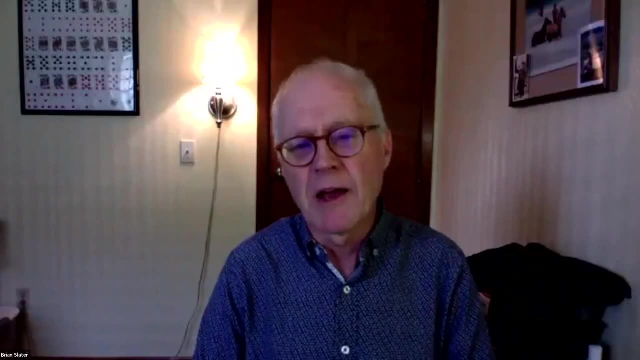 and and there wasn't that medieval warming period in Australia. but I'm going to refer to a place that I've spent a lot of time and that's Iceland, And just to quickly relate what we do know, that's one place where this has been studied intensely. 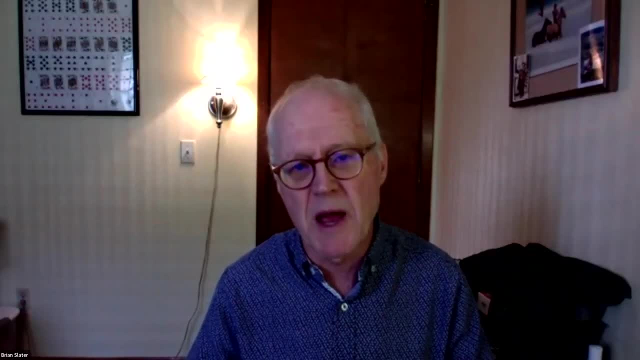 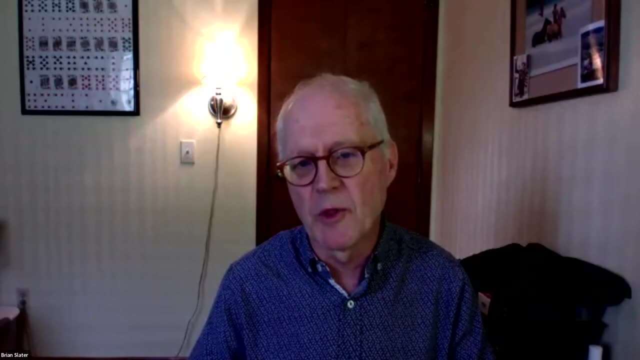 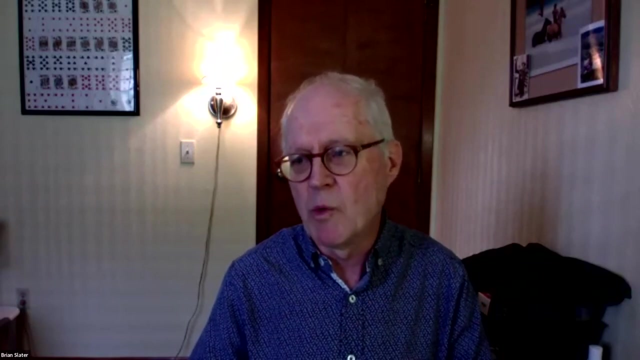 And the reason is that Iceland was settled by Viking settlers about 870 AD, plus or minus a couple of years, So there were no people there before then There were. just about 25% of that country was covered with forests- birch forests. 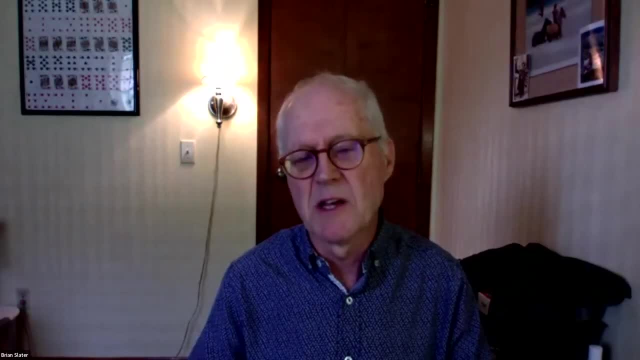 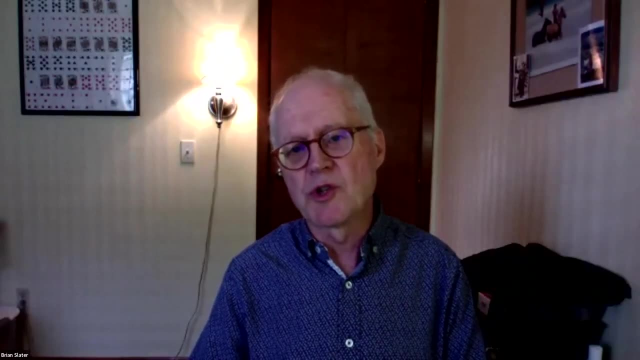 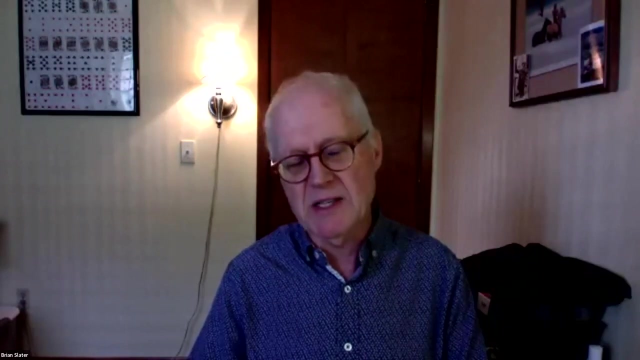 And about 50% of the country was covered with ice. The rest was mostly wetlands. So when, when, when the Viking settlers came, it was during that warm period, So they knew it was warm enough. they found a lovely, warm green place. You know it's cold enough at some times of the year. 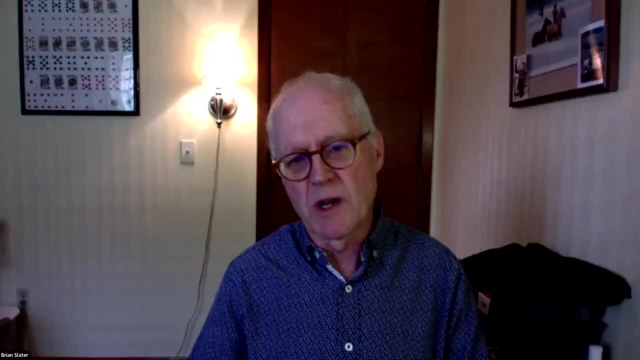 but because of the Gulf Stream, Iceland is relatively warm for its more than 60 degree north latitude So – And so when they came, there were forests and they cut them all down and they brought grazing animals, And so you know they were back to less than one percent forest cover. 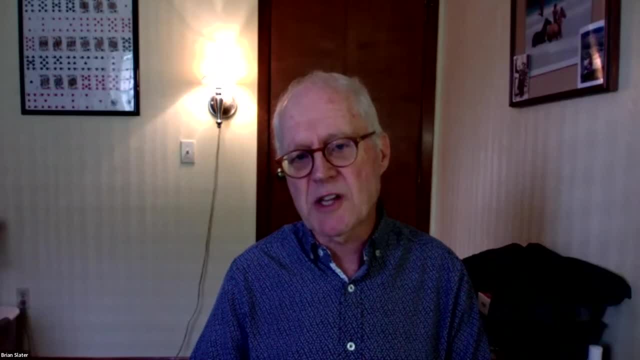 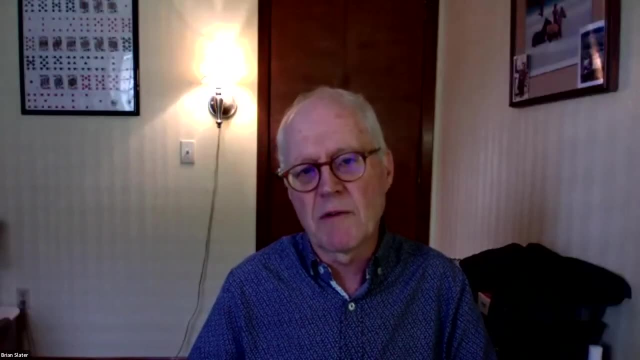 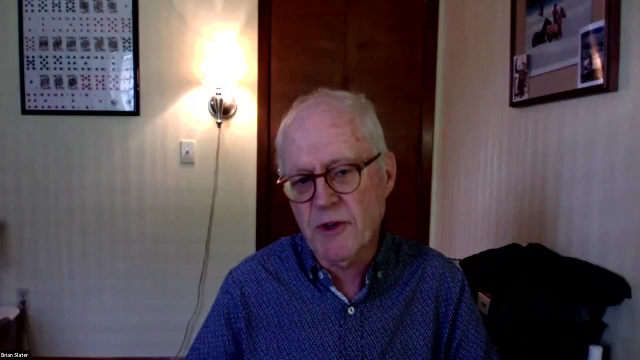 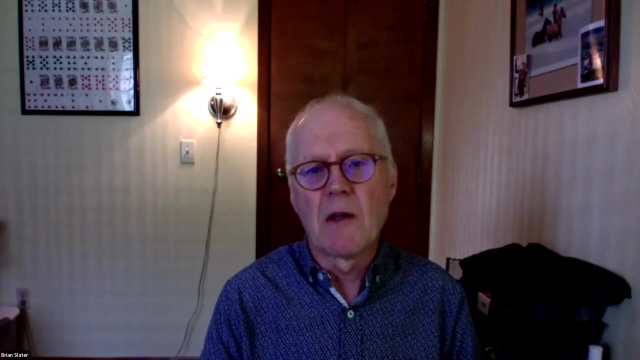 And as, as temperature warmed, those forests had been increasing. We know this from pollen in wetlands and and fossil evidence, And so we know those forests were increasing and organic carbon was increasing significantly over time. And so, as as that happened, those, those, those soils, got carbon. 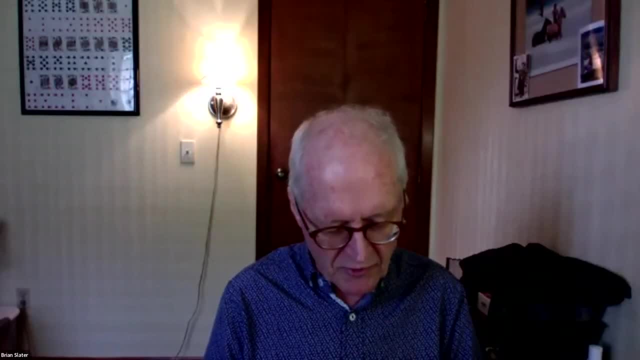 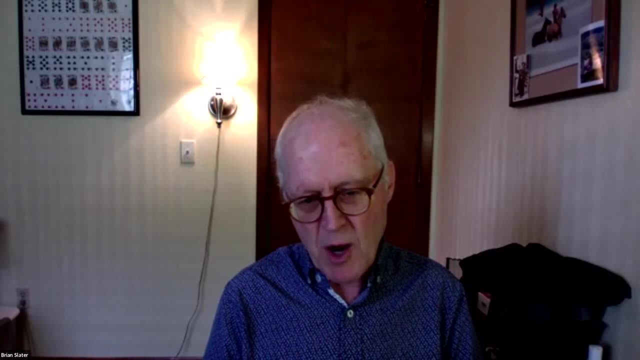 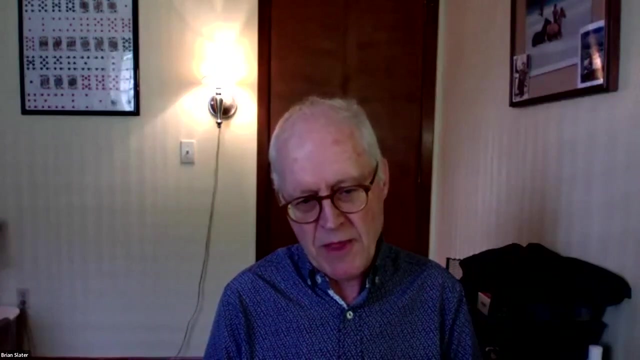 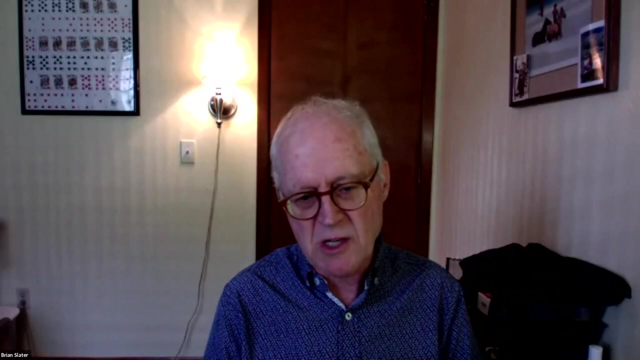 And then humans came along and got rid of all the forests and severe soil erosion followed and loss of soil carbon. So probably most of soil carbon in Iceland was lost after the warm period. And then they head into the little ice age From you know maybe the 13th century, 12th to 13th century onwards, a couple of hundred years after the Vikings had settled, all of the vegetation had been lost, severe soil erosion and large amounts of soil loss ensued. 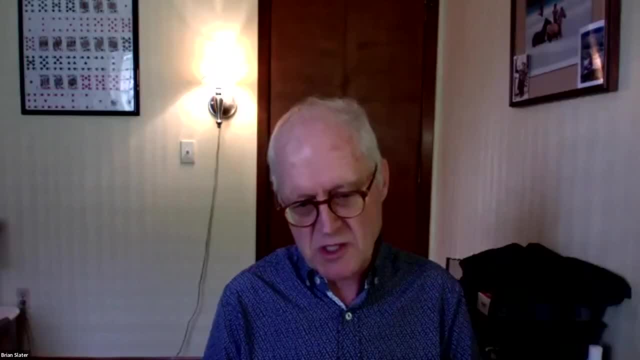 The last 100 years Iceland's been trying to reverse that effect. So that's one place I know how those things happen. So I think we could also extrapolate to North America That during that warm period, even though it was warm, it's not like the kind of temperatures we expect to see in the coming century. 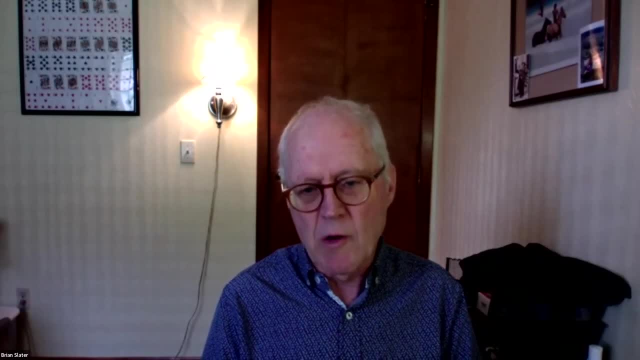 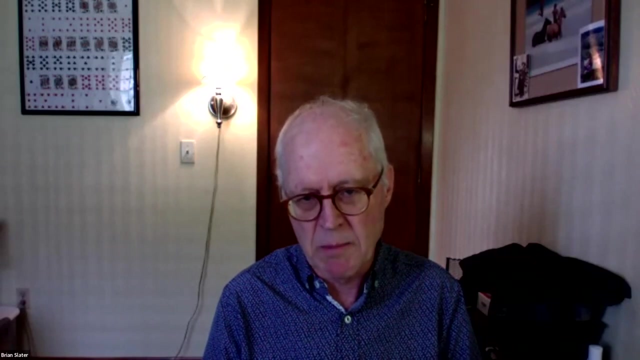 OK, so we're, we're already. you know, interestingly, Iceland was totally free of ice at about 8000 years ago. But you know now we still have ice there, But within 100 years or so most of that ice is going to be gone and we're going to be back to there. 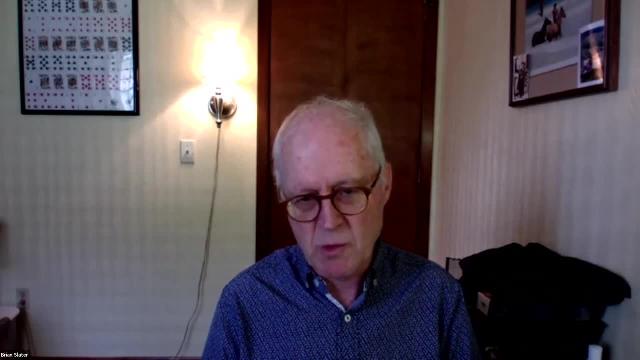 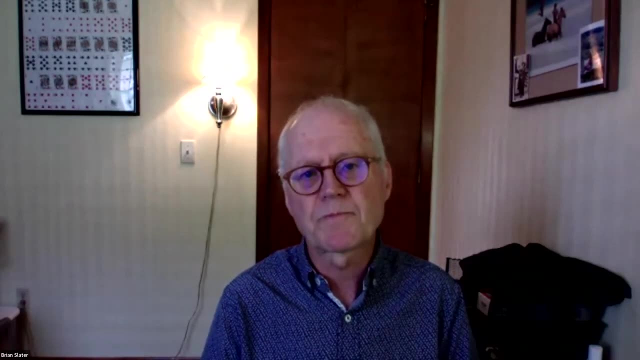 Icelanders are going to have to face kind of what conditions were like about 8000 years ago. So that's a bit of a summary in terms of what I know, which is an area where I've done some work. So that's good. 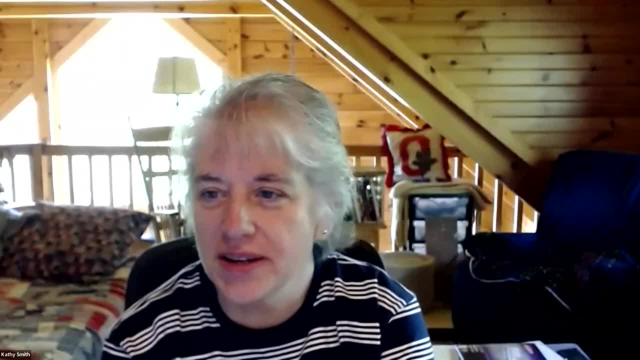 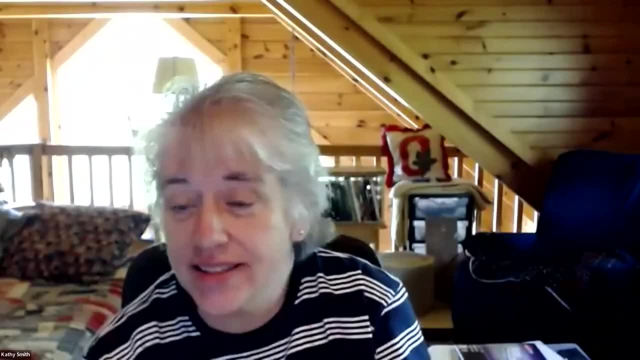 So Kathleen Bradley, she's going to go to the earthworm thing Brian discussed before, but effective earthworms on forest soils in the Great Lakes, how they are ruining it. Will flathead worms that eat earthworms help survive? Will they save the soil? Well, that's a that's something that I can't really answer. I don't expect that predatory worms will greatly influence earthworm amounts in forest soils and whether or not OK, so it's a complex question. Whether earthworms Are totally detrimental, somewhat detrimental, somewhat advantageous or very advantageous in soils, I think in in natural forests they're mostly we would consider invasive, And also in those parts of the country where there were native earthworms they've been very strongly competed against. So we no longer have them too much. you know, to much of an extent The earth in European earthworms are very dominant in many parts, And so they're a very large part of the world. So if you look at cities like North America, the majority of the population are native earthworms. And so you know, in the rest of the world there's a lot of native earthworms. You know, for example, in the rest of the world there's a lot of native earthworms. You know you have the northern parts of the North America. there were probably very few earthworms before European earthworms were introduced. 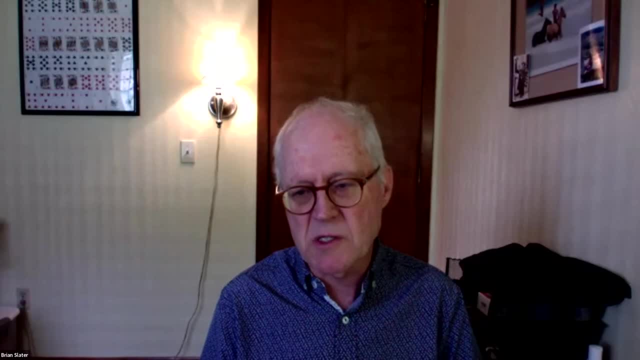 And so you know now they're doing a lot of things in the soil, They're mixing soil, But this might be in some cases advantageous. So if we think about- and again I'm not making a claim one way or another, So if we think about- and again, I'm not making a claim one way or another, I'm just trying to say that, you know- if we think that carbon can be better stored, particularly in deciduous forest systems, by redistributing the carbon away from the surface, then the presence of earthworms may actually be something that is actually a good thing. Again, it's too complex for me to take sides one way or the other, And I don't think there's a lot we can do to turn back to pre-European conditions in forests. But there might be a silver lining in the way earthworms do redistribute materials. Okay. Next, Sue Simon says: is there a difference between fungal and bacterial growth in metabolism with higher temperatures? Does this affect the acidic levels? Yes, So the answer is yes. So typically, bacterial growth is enhanced at higher temperatures and fungal growth is able to be more- how would we say, competitive at somewhat lower temperatures and moisture conditions. Fungi are more sensitive to low moisture conditions than bacteria. Bacteria tend to turn over organic matter much faster and recycle it quicker, And they tend to get to organic matter that fungal hyphae cannot to some extent, So there is a definite difference. As temperatures go up, I think bacterial growth will be enhanced vis-a-vis fungal growth. How does this affect acidic levels in the soil? Well, breakdown of organic matter creates soil acidicity To some extent, but it's more effect on the organisms than the other way around, because fungal systems are more prevalent at low pH, so that I'm I'm I'm inclined to think that higher moisture contents and higher temperatures will tend to bring conditions that will bring water through the soil quicker and therefore leach soils faster. 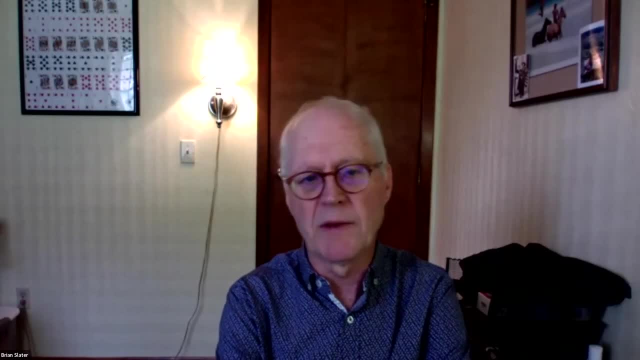 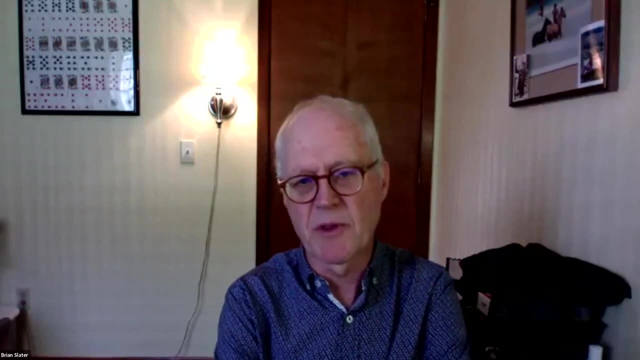 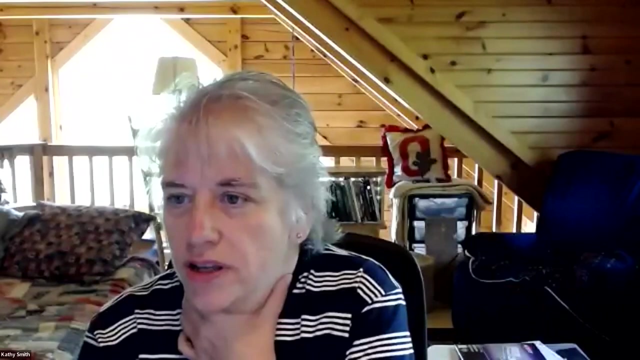 And creating more soil acidity That way, and that will end up end up enhancing fungal growth. So again it's it's fairly complicated, but there are definite differences in some of these aren't well understood. Okay, So Simon also asks: is there carbon stored on the ocean floor? 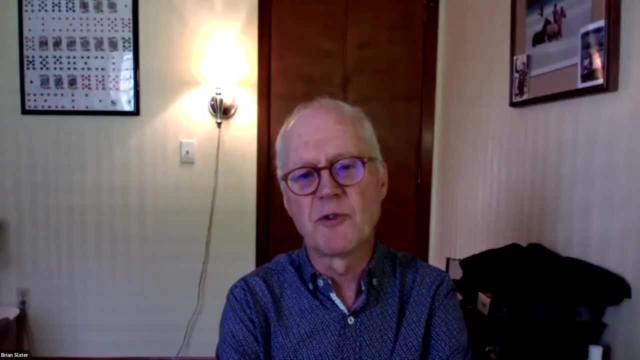 Absolutely So. you know the the ocean floor is a major storage place for carbon in the in the form of carbonate. So you know, millions of little Plankton and shell bearing organisms senesce and die and fall to the bottom of the ocean. 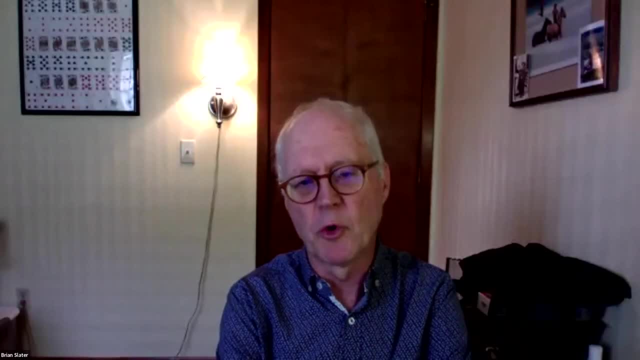 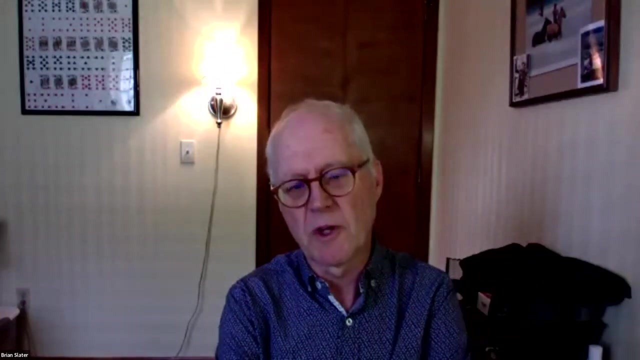 So if, if we think about the greatest carbon store on our planet, it's our carbonate rocks, but we we don't consider those. and you know, most of those were formed at the bottom of the ocean, as as as limestone, over over hundreds of millions of years. 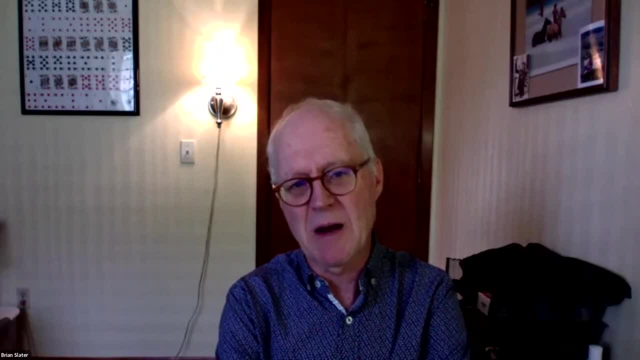 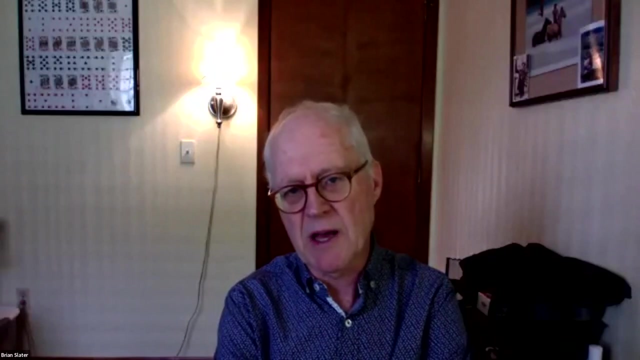 We, we, you know, we, we almost ignore them as part of the carbon cycle, Because they're they're they change, they're less amenable to change. but we- we also at our peril- have ignored them because, for example, the soil acidifies, that carbonate store is, is is affected by, by acids in soil, water in moving water, and and more carbon dioxide is lost. 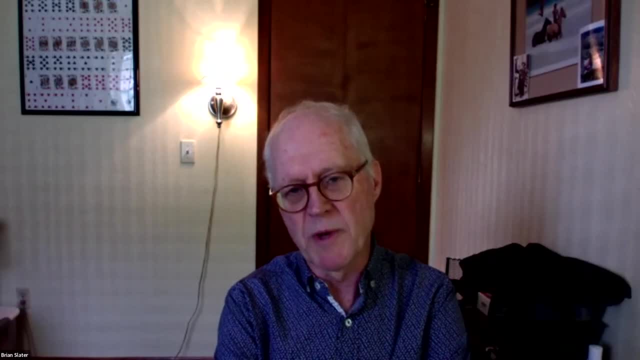 So the, the balance over time will be organic carbon in soils is going to be also very strong. So, anyway, that's getting off the point. but yes, yes, the the bottom of the ocean is, you know, over hundreds and hundreds of millions of years, the major place that that that carbon actually gets. carbon gets stored. 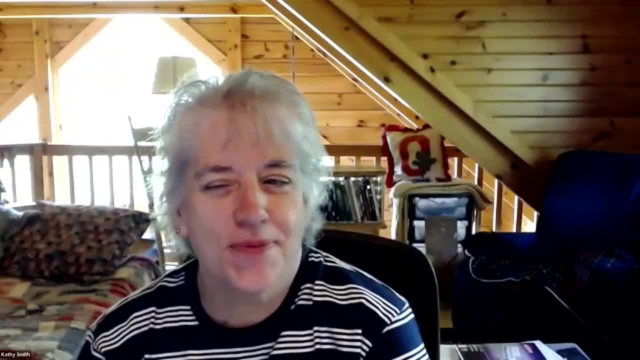 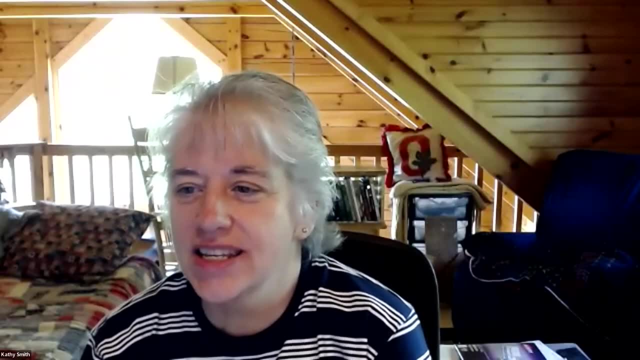 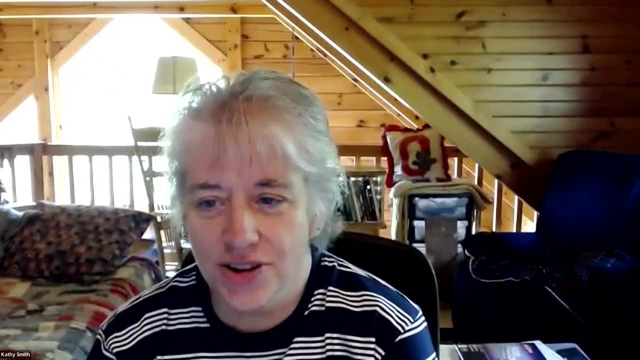 Okay, So here's a name from the past: Brian Bob Bertry says as Northern soils, like tundra, warm, it is not only CO2 that increases, but methane is perhaps, So even a greater impact on greenhouse increases correct. 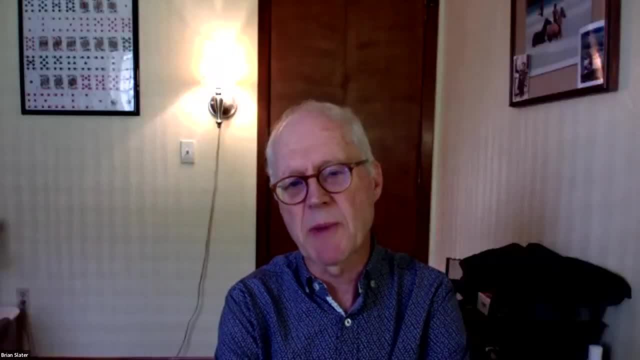 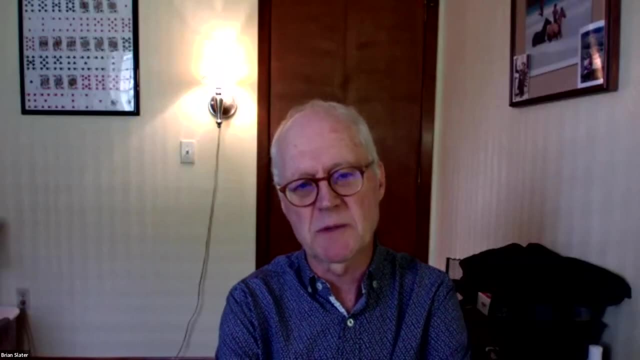 Absolutely So, you know. so you know. we think just about carbon dioxide. carbon dioxide is the end product of, of aerobic respiration of organisms like us and trees and microorganisms that respire when they can get oxygen, and and and and. when they can't, microorganisms need to still respire. And so they go around Looking for something else. they might find something like. they might find something like iron oxides they can use in wet soils. They might find something like sulfate they use, And eventually, if they can't find those- they can't find oxygen oxides or or or sulfate- they may go looking for carbon containing compounds which they can respire. And the end product in those very anoxic anaerobics. And the end product in those very anaerobic environments is methane, like in the stomachs of cows, in very wet soils, and and and. in cold wet soils in particular, there's more methane production. 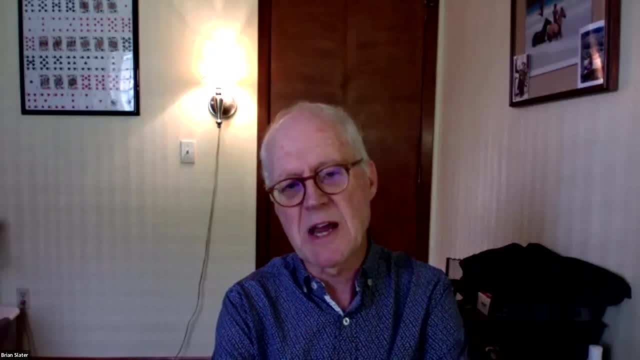 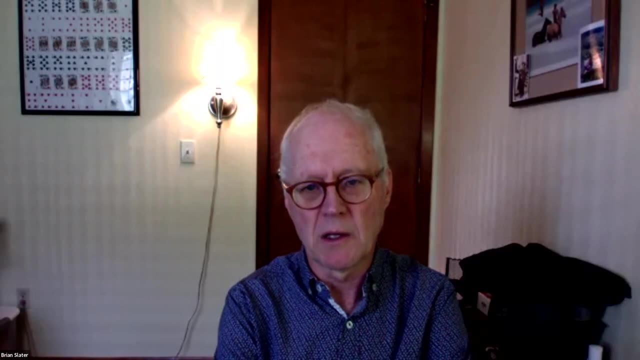 And so, yes, you're, you're correct. So, but all of the same things that pertain to carbon dioxide in aerobic respiration also happens in in in anaerobic respiration in terms of greenhouse gases. Yeah, Maybe he was just testing you, Brian. 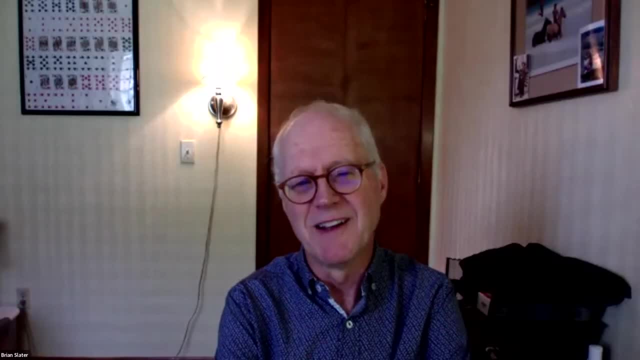 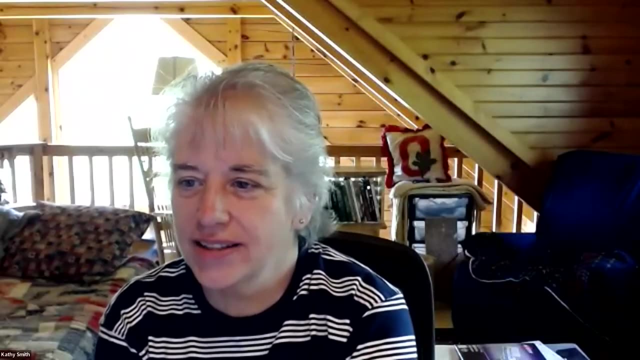 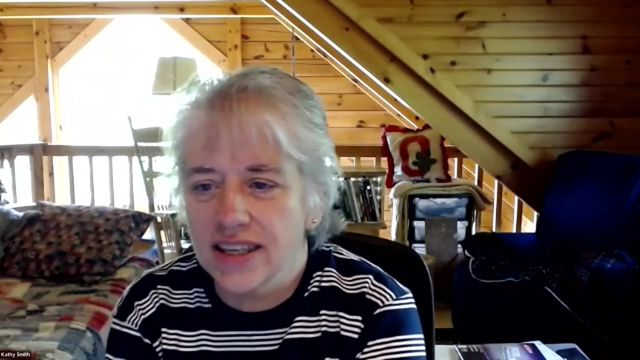 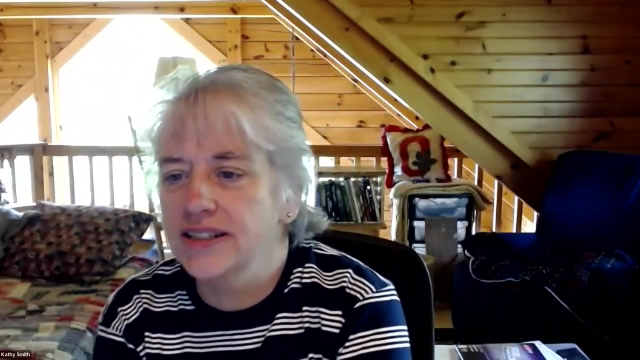 Bob always He's good at that. So Sue Magnus says: what are your thoughts about biochar, compost activation for planting and ideal soil mixes? city of Cincinnati is in planning stage of getting a kiln to make biochar. What type of solid mixes would be best for to make for planting trees to store carbon? 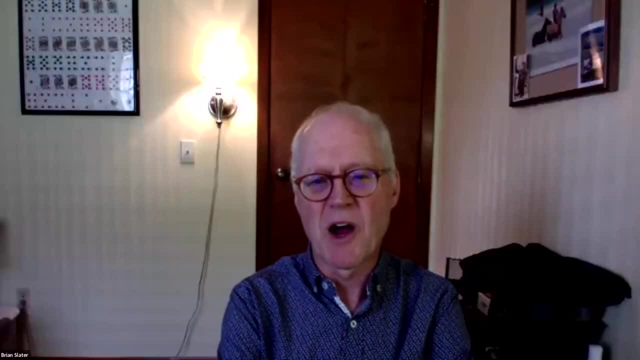 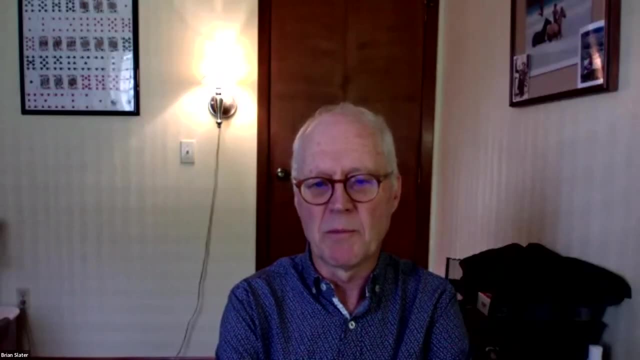 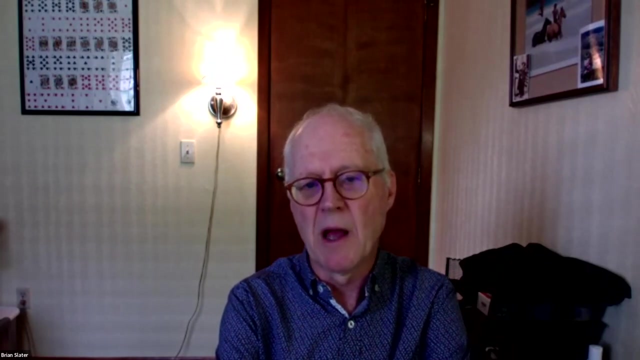 So there's a lot of questions in there. Okay, there's a lot of questions there. So biochar is is a form of carbon that's made in, you know, made by burning materials in a low oxygen environment, so basically creates long term carbon that doesn't create carbon dioxide and it's. it has excellent, many excellent effects of organic matter on soils. 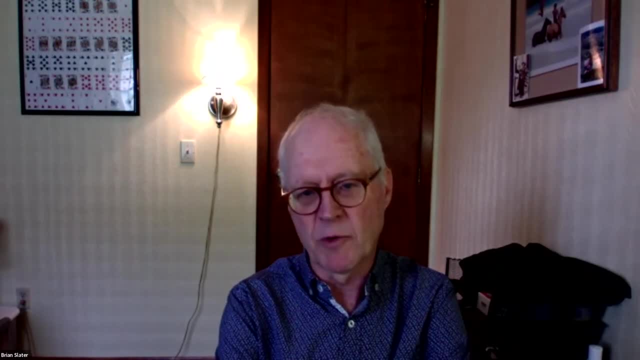 It's a very hot topic of research in the soils and other communities. It's a very good topic to talk about now. So you know I'm strongly in favor of it. I'm not sure it. you know that economically it's something that is an ideal way. 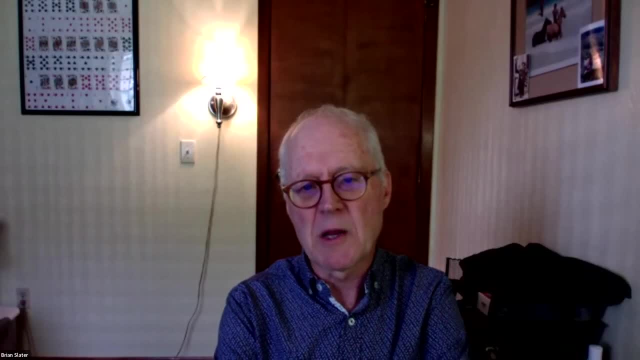 So I think any way we can get organic materials on carbon into the soil is a good thing. I I don't really have much to say about ideal soil mixes Generally. the more organic matter, the better and more stable forms of organic matter the better. 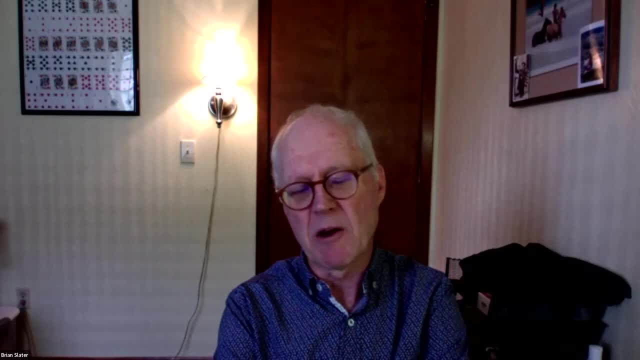 of organic matter, the better. so uh i. but you know, i think uh, if excess energy or burning of of waste products can be uh used to make biochar, uh, that's probably a good use of energy, uh, in terms of uh, in terms of creating a material that does have positive effects on the soil. 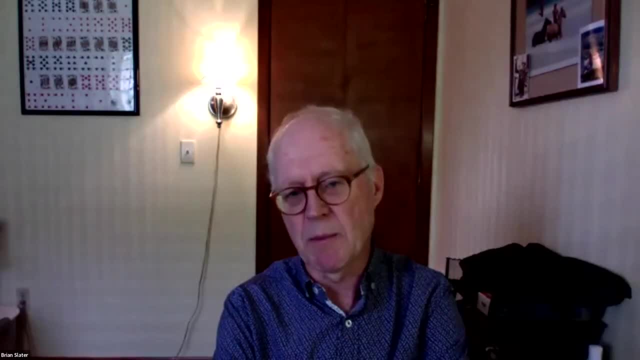 not just in sequestering carbon but also improving soil physical and other properties. so i i you know i'm not an expert on soil mixes, uh, but you know, i certainly think you know anything you can do to to uh involve organic matter uh, whether it be renewal or compost or 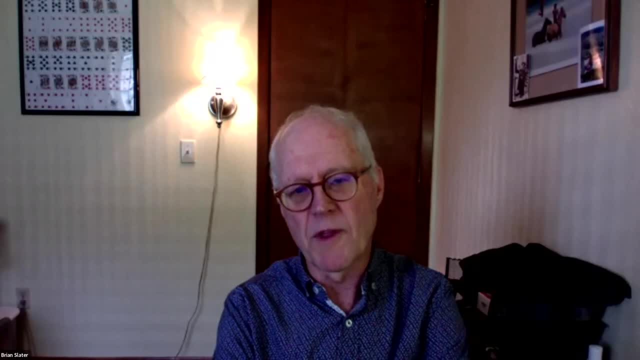 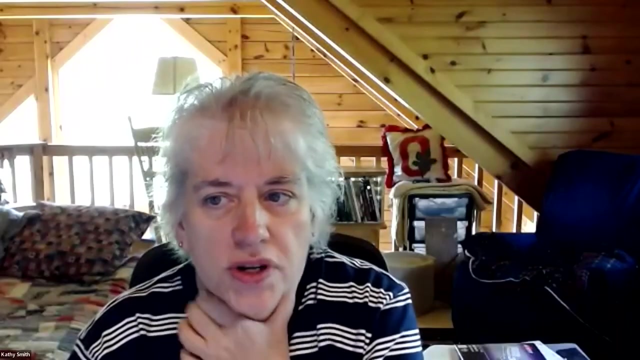 biochar, uh, uh, all of those things are excellent for using in mixes, uh, but it'll depend on the kind of plants you're trying to grow. uh, the balance of different materials that you would need, okay, um, what is frank asks: what is the impact for forest regeneration if the quality of the soil 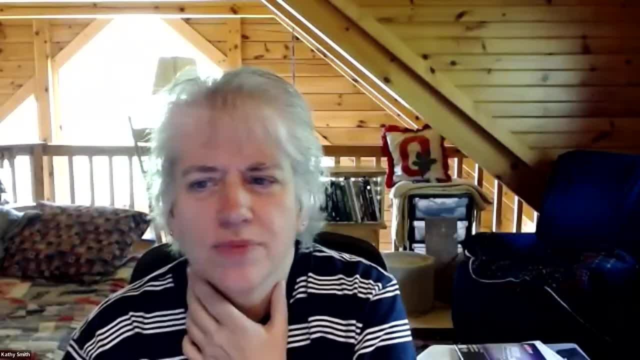 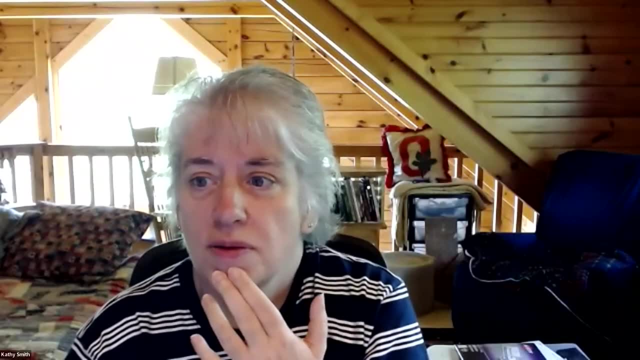 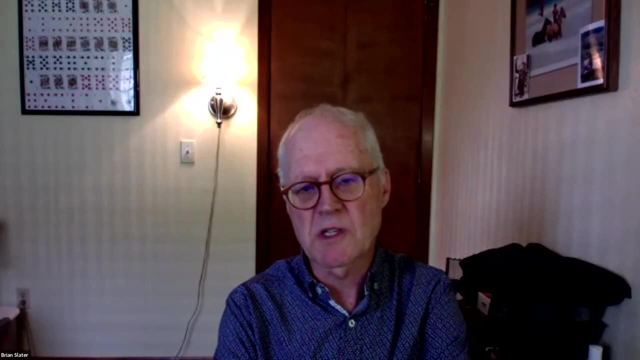 oh, of the quality the soil if it has been subject to a very hot forest fire. so, i guess, do hot forest fires impact that the soil quality for regeneration? yeah well, uh, you know, absolutely. so you know they're a very wide range of effects. uh, these uh. 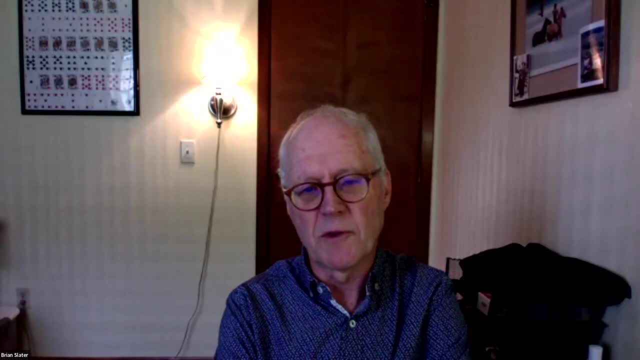 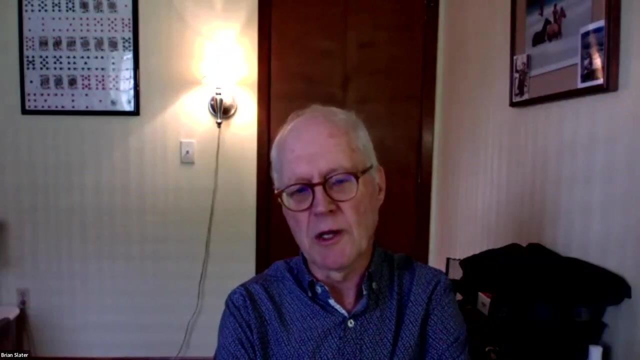 these, you know, include the loss of the. you know of all and most of the above ground biomass. uh, you know, in very hot fires, you know you do not leave much in the way of new uh material, uh for regeneration, uh, you kill even uh microorganisms and all kinds of detritivores in the surface part. 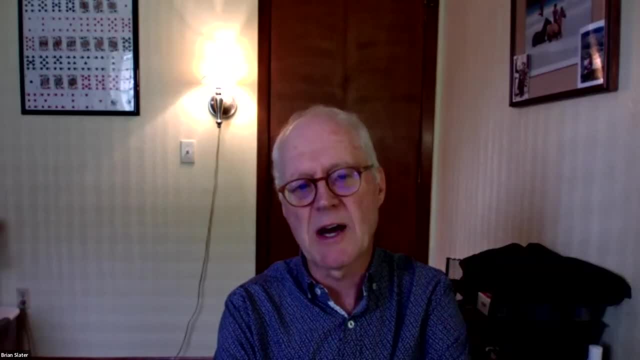 of the soil. uh, you volatilize a lot more of the carbon. so you know the hot, you know the hot. fires are far worse than any others. they also- they also bake the soil in ways that change the soil mineralogy. this may create new clays that tend to cement together. they tend to therefore increase. soil erosion, but i think the most significant effect is the loss of organic matter and the loss of organisms that can be involved in regeneration. the soil, you know everything from new seeds and seedlings that are still there, uh to uh, to vegetative reproduction of the understory that 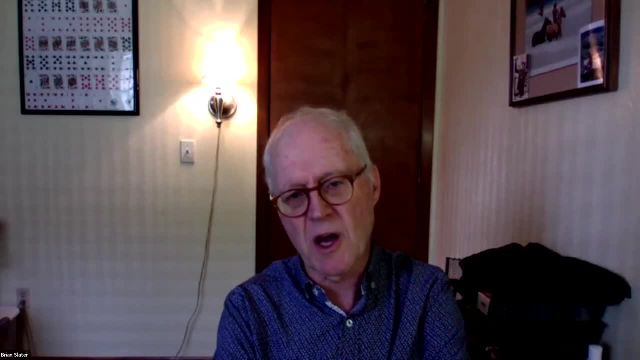 may survive a a lower temperature fire. if you just get rid of everything, you've got a very poor situation uh for regeneration, and the longer it takes to regenerate, the more that negative feedback on on terms of soil quality. so you get more soil erosion, you get more compaction. 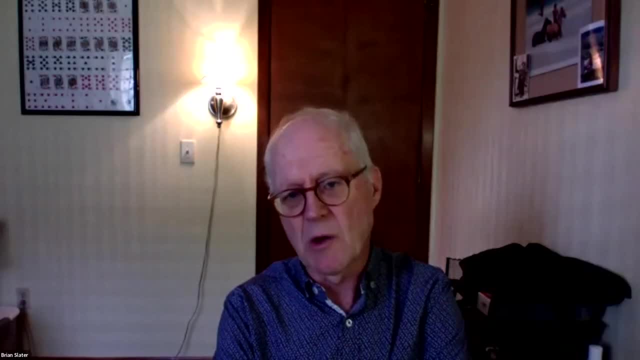 get more loss of physical materials, you get more leaching, you get all kinds of things happening that are disincentives to that regeneration itself. so hot fires are not a good thing in most places. they may have a role in some places, uh uh, you know, in australia, where i come from, you know. 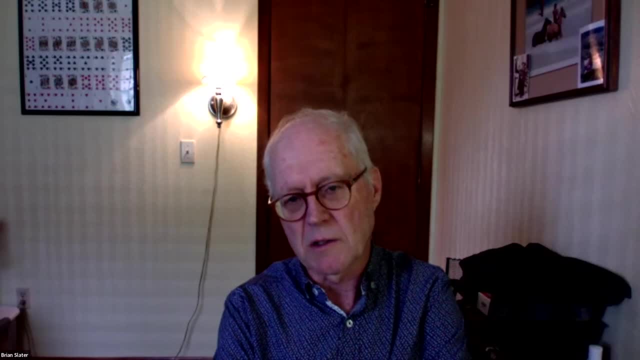 many of the eucalypt forests, uh, uh, you know the, the, the major forest type in australia. uh, they, they are stabilized by hot fires, but you know you have, you have understory that. uh, you know you have plants that are highly have, highly volatile and you know you have plants that are highly volatile. uh constituents of oils in their leaves, and so it. you know they have very hot fires, but it's the top part of the tree that burns rather than getting close to the ground, and many of the seeds are scarified by that burning. so you have no tasty. you know melaleucas and all of these other plants. and eucalypts themselves. many of these actually need to have hot fires, uh, to re-germinate. but you know that's a that's a specific situation in our deciduous forests and, uh, coniferous forests in the united states, most of our forests. 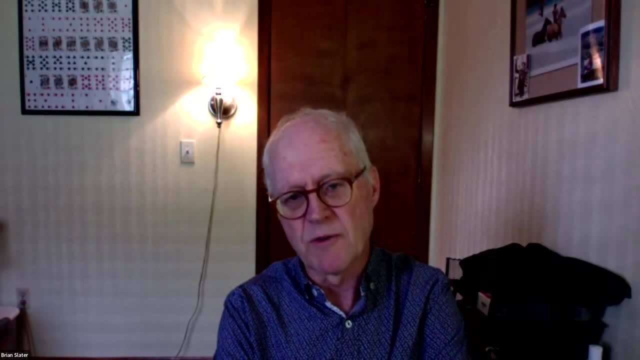 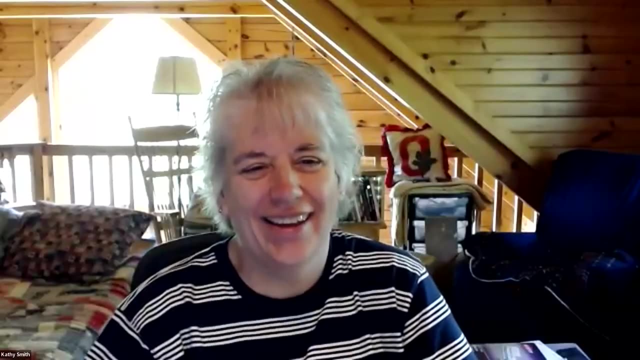 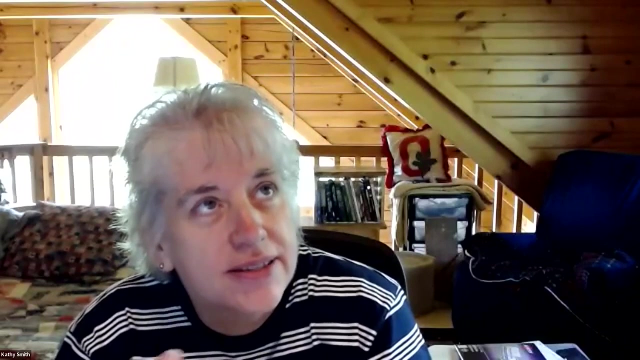 uh, are really not terribly resistant to very hot fires, but i'm i'm also speaking well outside my lane here and you know i, you know there are a few things that i do know. well, we do have conifer species in the west that need the fire to pop. 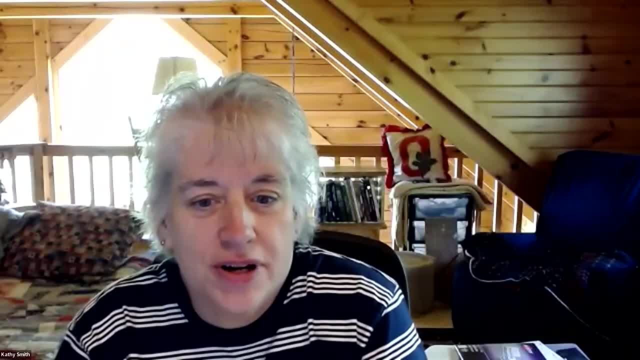 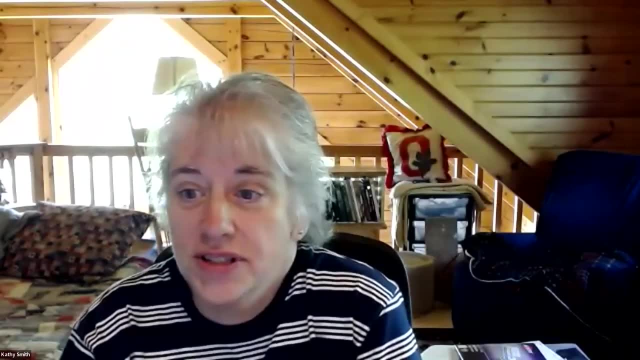 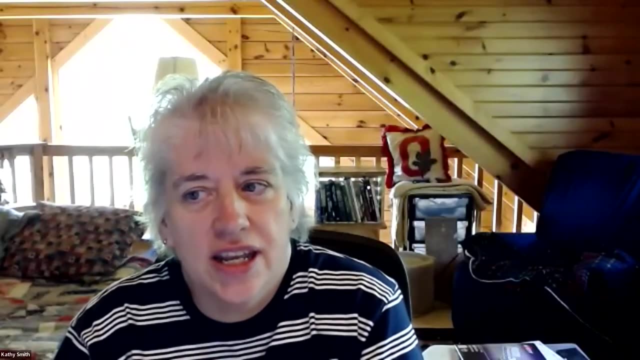 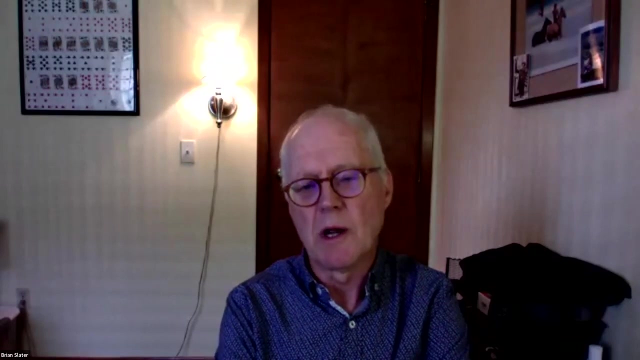 the cones, you know, for regeneration. so, um, there's a need for some, but the hot fires definitely are detrimental to the forest, in the short term at least. um, so sue asks: is there a large amount of carbon stored in antarctica? in antarctica, um, okay, so, uh, if you take the continent as a whole, antarctica has the least amount of carbon storage, but the reason for that is it's ice. okay, those areas of antarctica that are ice free have very large amounts of carbon for two reasons: they're cool and they're wet. so you have tundra vegetation, uh, over some of those areas, uh, and and large amounts, and you know. 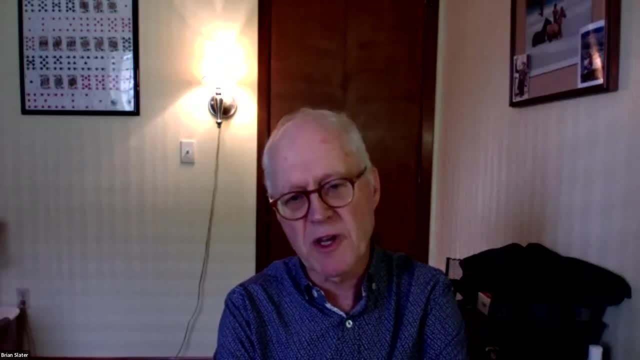 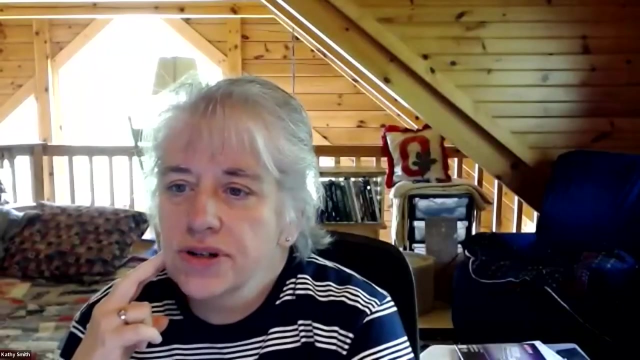 and wetlands, and so, uh, those ice-free areas in antarctica are, amongst per unit area, the highest, but as a continent, very little, because, uh, those areas are quite small compared to the total extent of antarctica. okay, uh, richard asks. well, actually, i think i'm going to go back to the 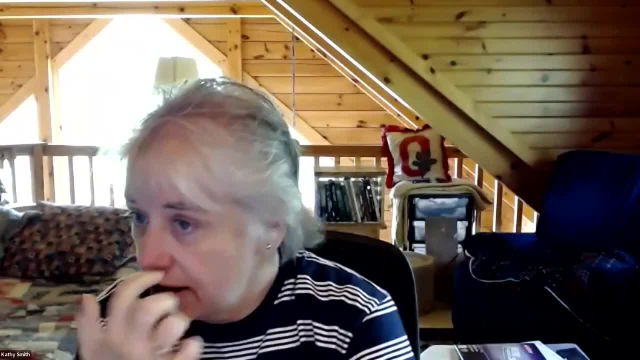 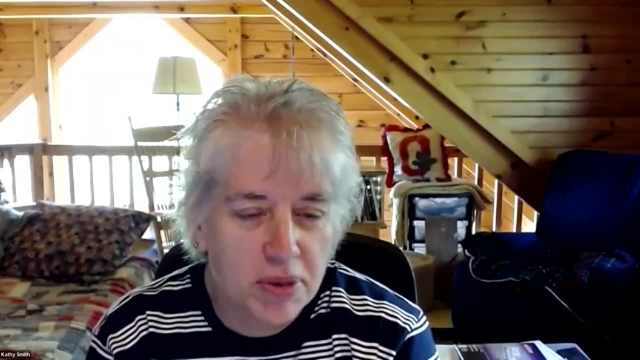 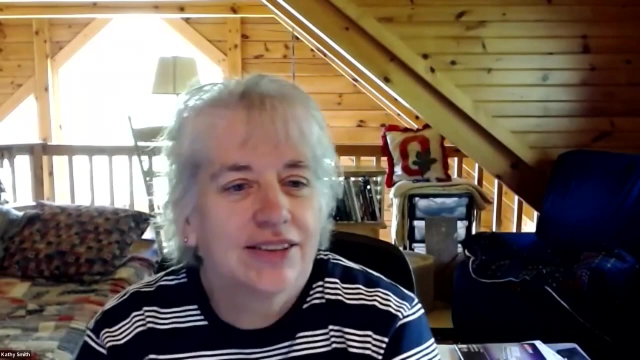 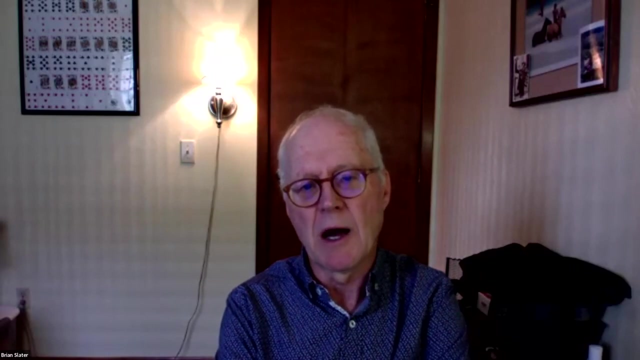 osas in antarcticly, and this is actually a very broad question, you know. you could say: i do care. uh, these forests, uh, and antarctica are now as if they were just deeply underside. uh, uh, one ek, for instance. i think, uh, i think, um, some of the best parts of that area, the 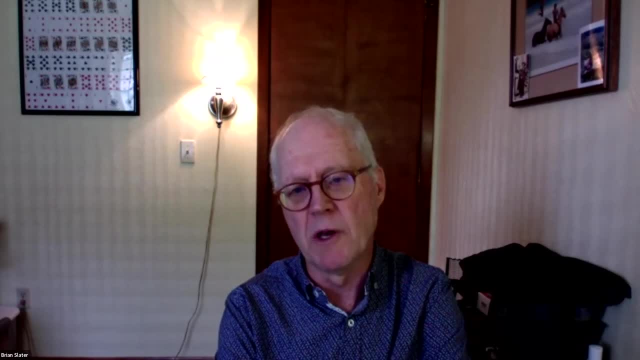 if, if the conditions that are ideal, or even uh, uh required for a particular plant, uh, or even a forest to grow, no longer exist, that forest is not going to be able to to adapt, you will get, you will get ecosystem change. you will uh, you will get, uh, not just habitat change, but you will get a. 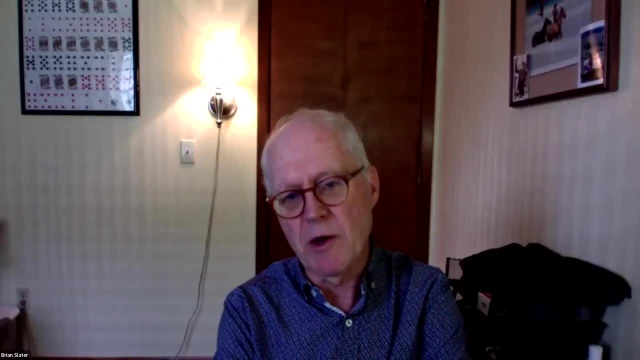 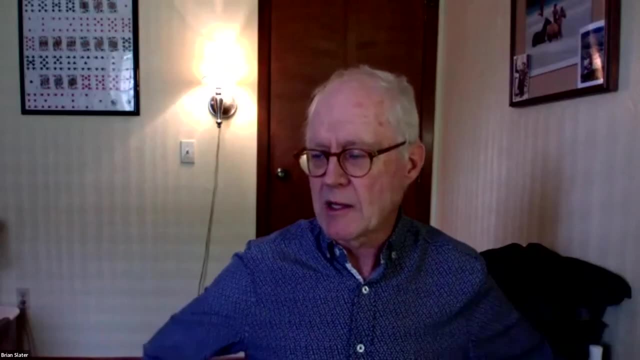 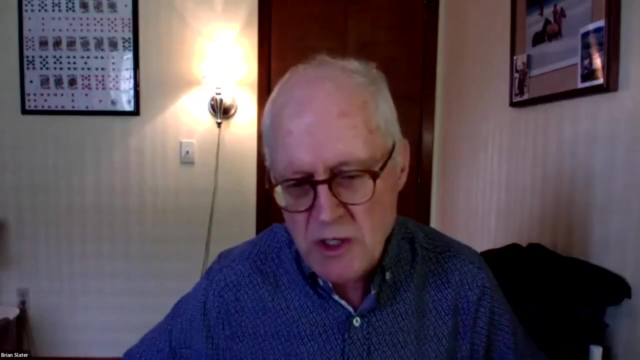 change in species composition. uh, that may or may not result. as i mentioned before, the this uh, we, we, we think that there is some kind of uh uh stasis below ground so that the below ground biomass, uh, the below ground uh plant, uh micro walks in communities probably won't change as fast. as the above ground, because you know, temperatures don't change as quickly as you go down the soil, uh, but that will create some kind of imbalance because these organisms co-evolved, uh, and so i, you know, i, i, i don't think the rate of climate change, uh, that's that we perceive, uh, that we, you know that, that most of us, that many of us. 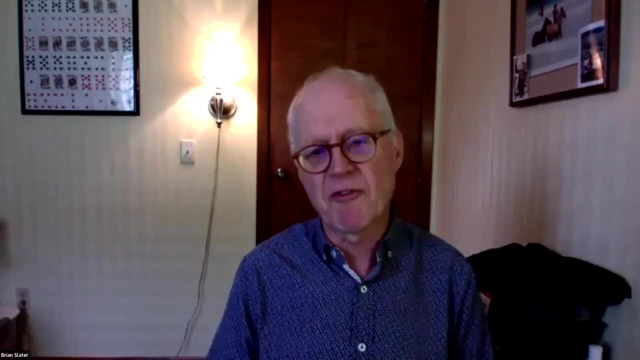 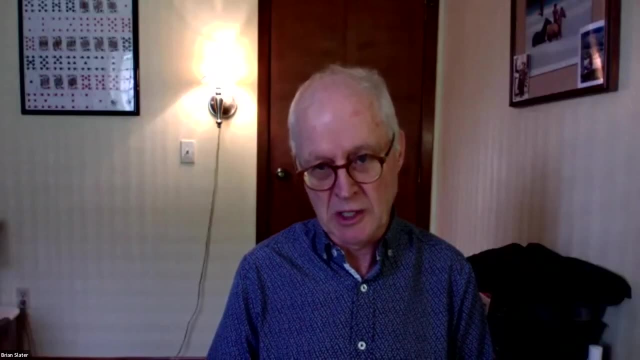 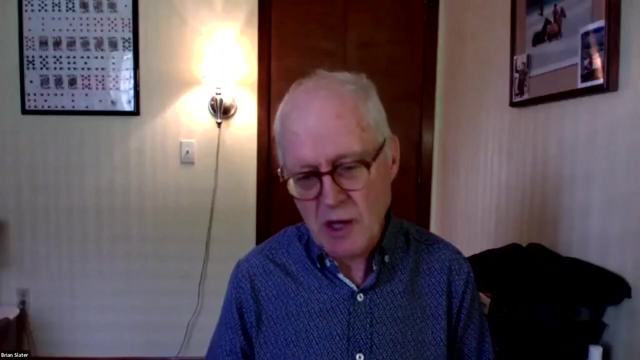 feel is going to happen. uh is far faster than uh the rate of adaptation of uh of individuals, and certainly even uh of of of of whole ecosystems. at least that's that's the way i see it. of course there's some adaptation. you know plants can uh, you know, can mutate uh, and 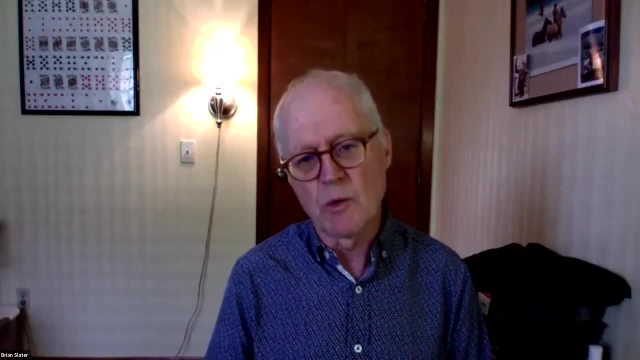 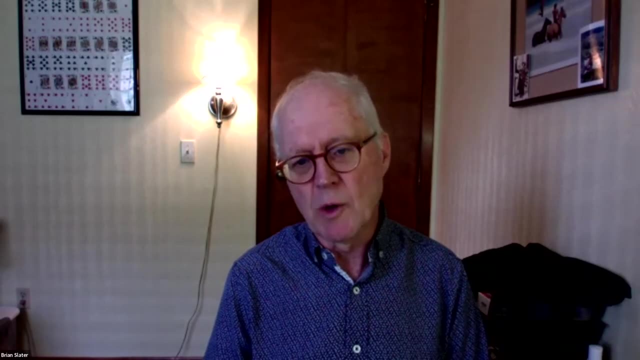 and and the ranges of plants. uh, there's resilience. so resilience is the one thing that that, uh, that has the opposite effect there. so you know, uh, plants don't necessarily have to change straight away, and some are very resilient and some aren't. but the thing is, when you get changed, then 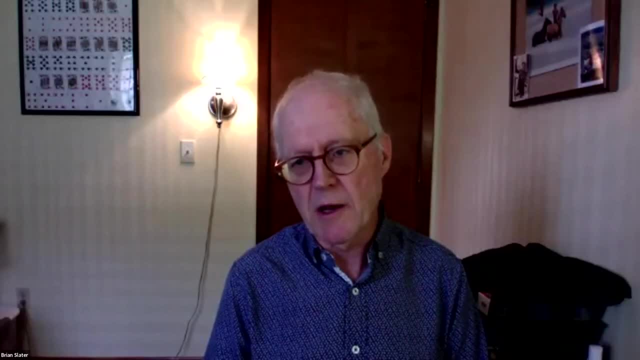 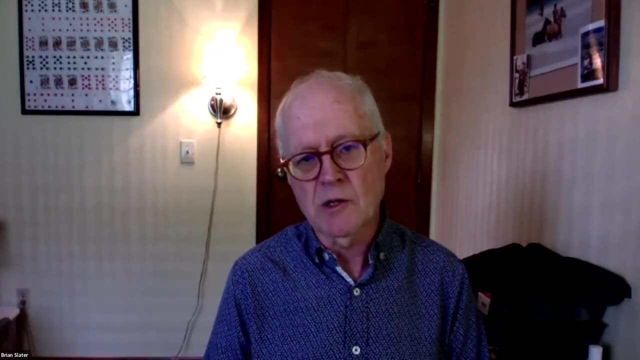 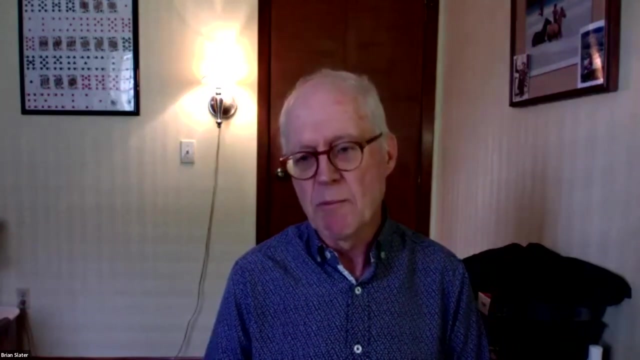 plants that are resilient? uh tend to dominate over those that are sensitive, and among those things that are resilient are things like invasive species. uh, and and so uh, as as as uh, as ecosystems, including forests, come under stress, uh, it's, it's, it's those more resilient uh pioneering, and invasive species that will first take over before there is a shift. 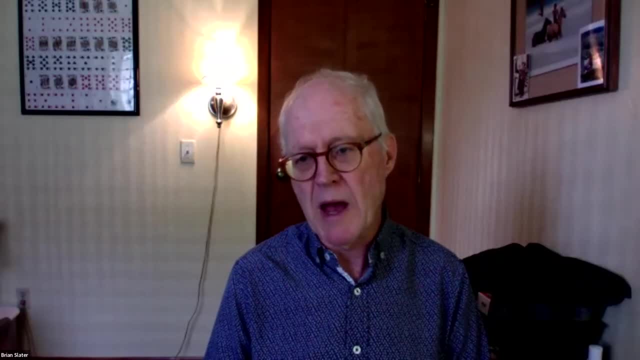 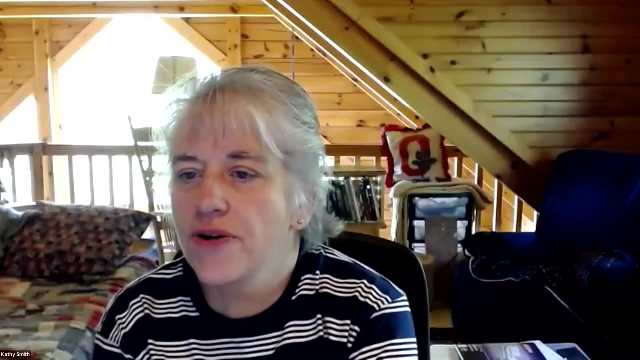 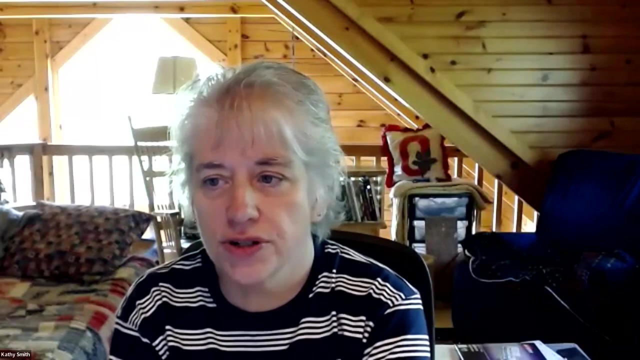 towards- uh, uh, you know- a new balance of plants. okay, michelle asks. let's see, she was wondering how or if the increase in ohio's summer temperature, in the change in soil as a result, will impact agriculture and the types of crops that can be farmed. 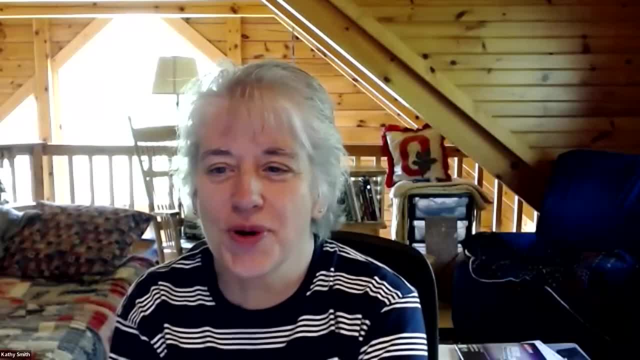 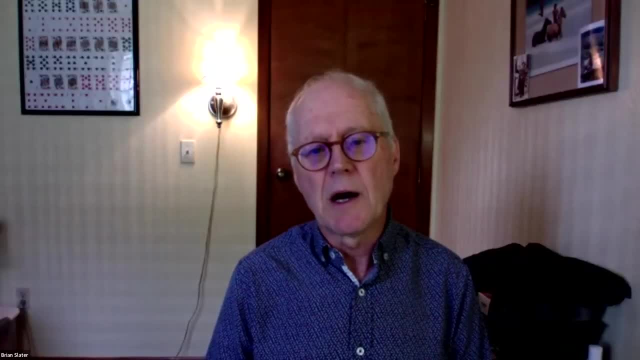 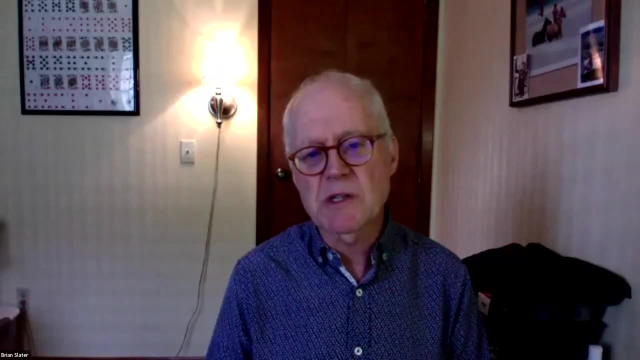 example, will future generations still go to their local farmers market to purchase corn? yeah, good question. and you know, i think, uh, again, we, we don't know what, what's going to happen, but uh, increased summer temperatures, uh, there's two effects there and i i kind of pointed out, you know, warmer temperatures will mean. 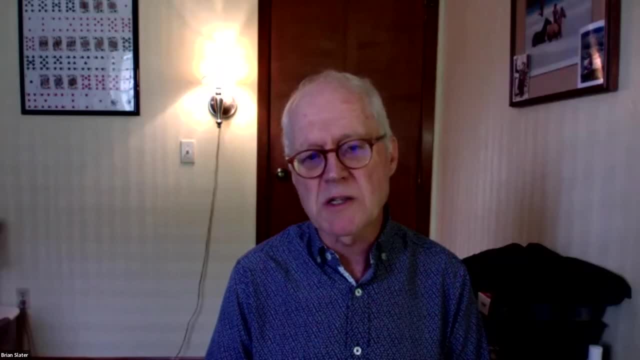 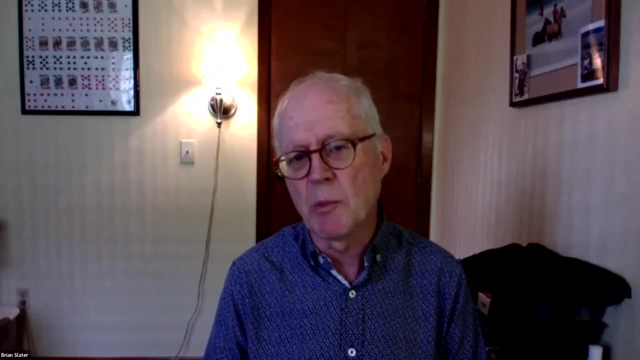 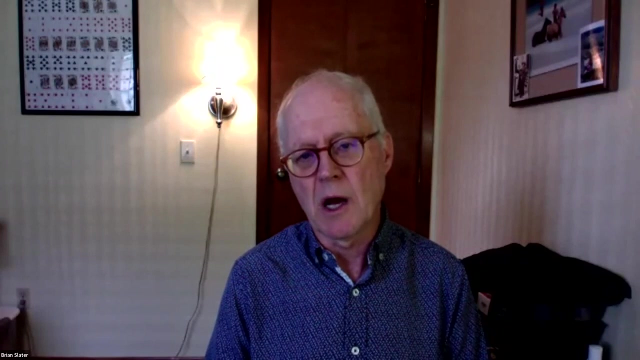 uh, typically, you know, a longer summer growing period. okay, so warmer temperatures early in the summer will allow farmers to get their crops in in a more timely manner. uh, that that could result in better crops in ohio, right, uh and uh. on the other hand, i mentioned the soil water deficit. 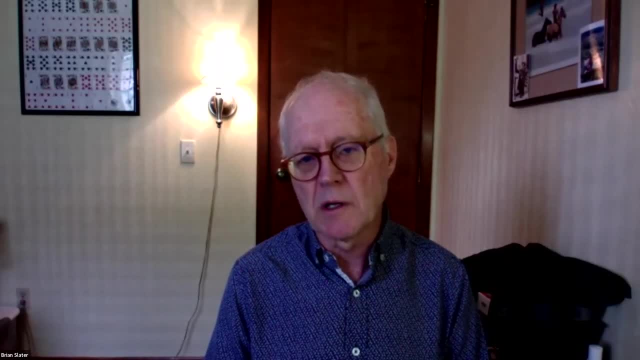 uh, that we have on average, you know, in in uh, late to mid, mid to late summer, uh, that is the major determinant of crop yield. neither of those would mean that corn would be not suited to ohio- i, i, i don't think you know. and to some extent increased productivity, uh, but you know, if we 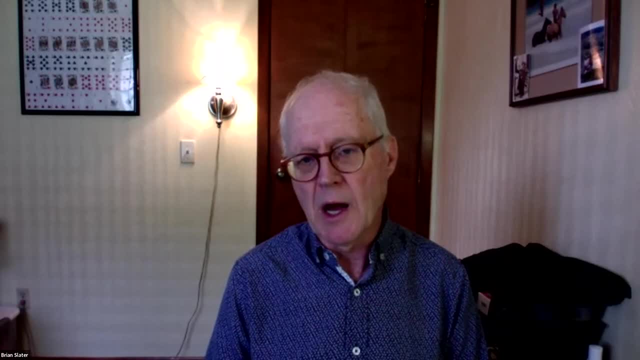 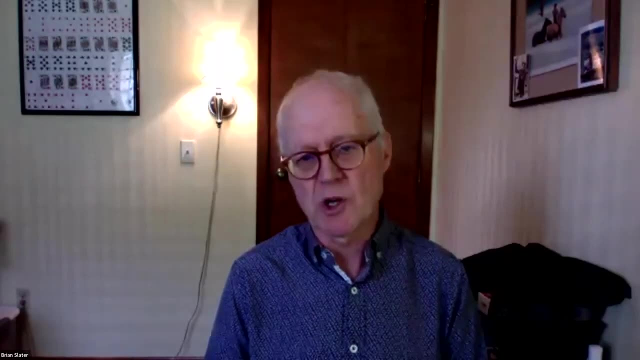 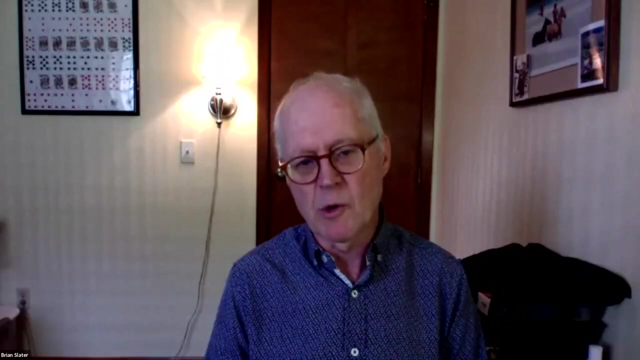 imagine hotter summer temperatures will probably mean uh that that uh, summer deficit period of moisture will be higher. that may be the main influence on crop yields, and and and may reduce overall long-term crop yields in ohio for corn and soybeans. um, but again we we don't really know, but some models do tend to show. that uh, but it's kind of a balance. so some increase uh due to due to increased moisture uh and, and warmer temperatures uh, and earlier planting times will mean uh higher crop yields but a higher risk of of dry conditions uh during the deficit period will reduce that. so how that'll break out it may. 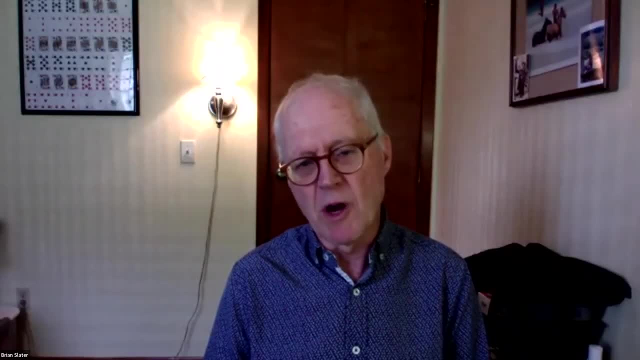 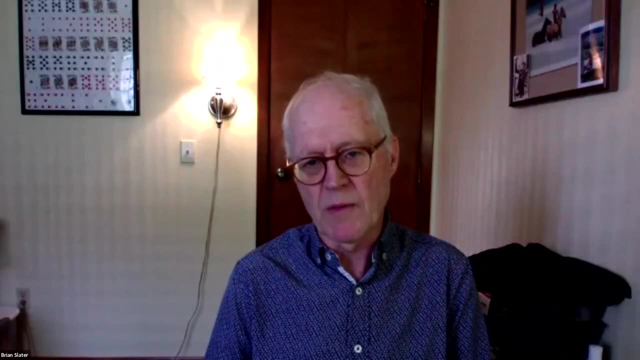 be a wash. it may fall one way or the other. so i, i don't, i don't think, and again, we don't know what the extremes are going to be. uh, you know will. will the environment be even one that's amenable to, to farming? we, we don't know, but i would expect you know the changes that we see. 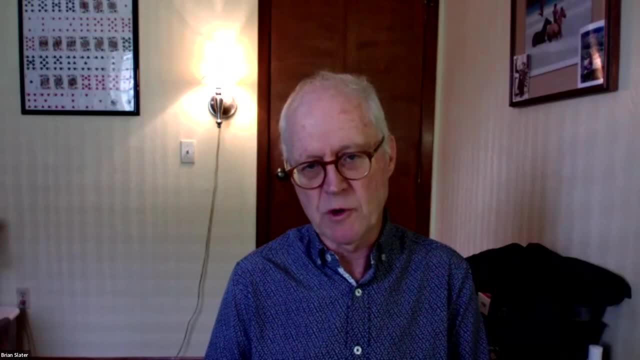 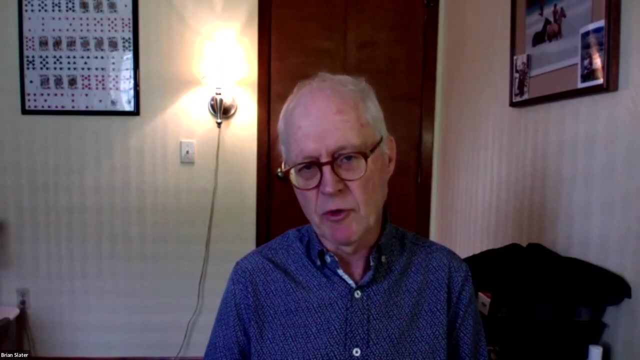 are probably not going to mean we can't grow uh major food crops in ohio. uh, if you're an indian different story, you know uh temperatures uh already getting so hot there that you know it's hard for people to live, let alone get out and do the farming that they have to do to maintain uh you. 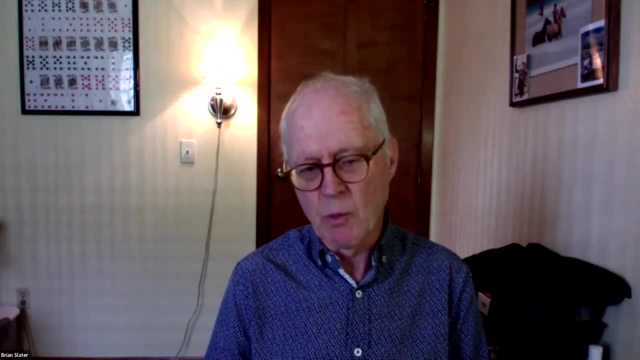 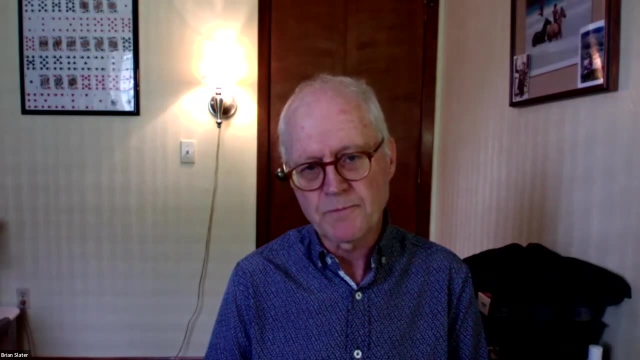 know what's going to be the world's largest population. so, uh, we're in ohio, we have our challenges with climate change, but nothing like, uh, particular other areas of the world. so, brian, just to kind of follow up on that, do you see? then you know, we typically think of like. say corn harvest starts mid to late september into october, do you see, maybe that starting in late august, early september, do we see, maybe those harvest patterns change, yes, okay, okay. so if you look at let's, i don't know, but if you look at those university of massachusetts predictions, 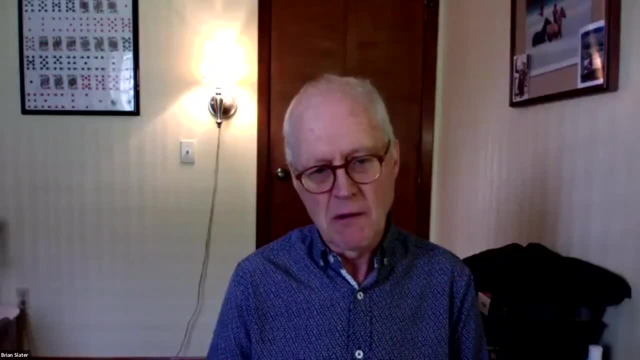 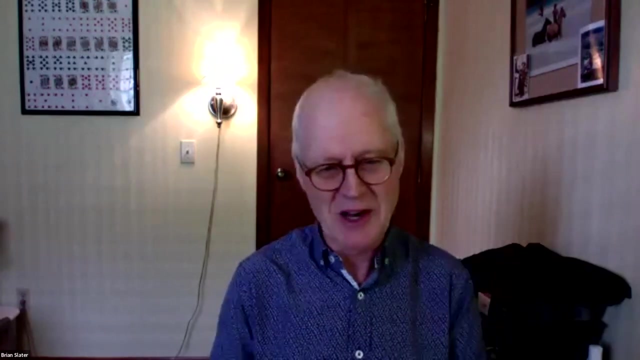 you know, if ohio summer is more like arkansas, then uh, you know where they. you know we've got more soils than them. right, it's got. you know, arkansas is going to be more like, uh, mexico, i think you know, in terms of their, their temperatures. but, um, you know, at least you know again, i'm not. 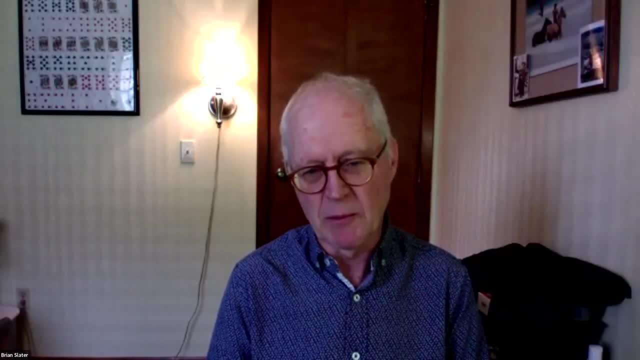 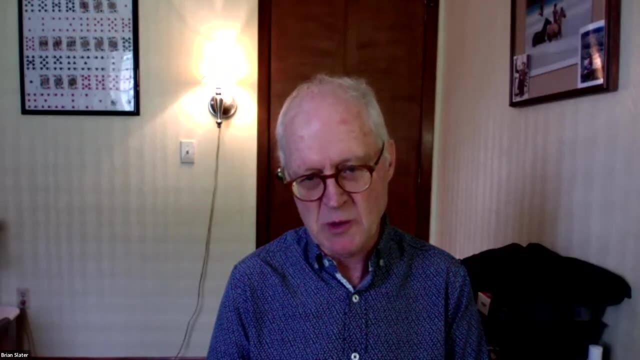 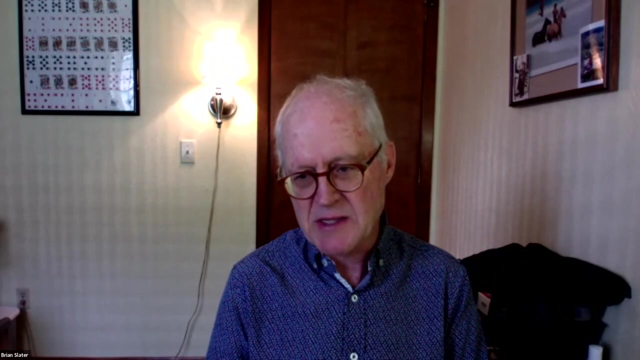 i'm not an expert on making these predictions, or a model even, but you know i do read this stuff, like the rest of us do. uh, and as a scientist, you know, i i think some of this is, is is what we're most likely to see. um, uh, given that, uh, you know, if you see planning dates. uh, now, uh, and winters are still going to stay much colder than arkansas, probably, or a bit colder, so uh, so that may uh that that kind of limits how early we're going to be able to plant. but uh, i would think, if a few weeks earlier i would think things uh maturing a little bit faster. 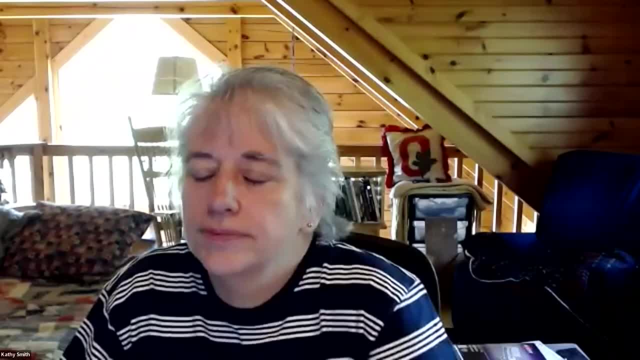 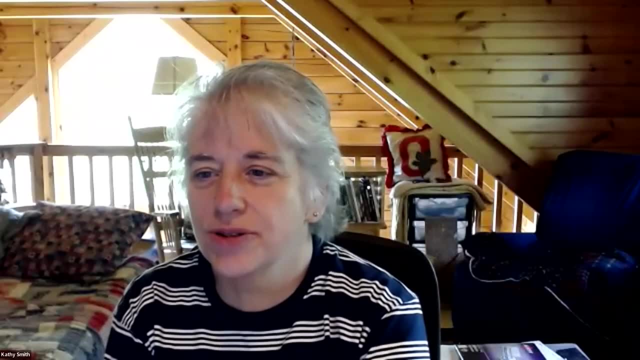 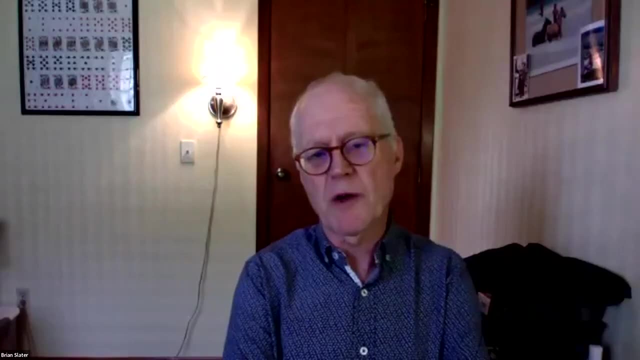 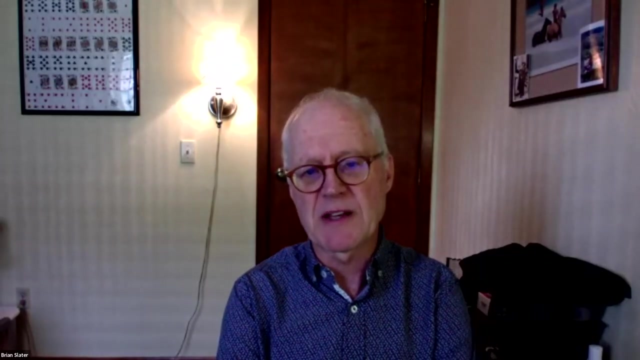 and and probably earlier harvests. okay, um, we have anonymous asking: is ohio at risk of desertification, perhaps during the drier times of the year? you know it. so desertification has got a wide range of, of, of definitions. um and uh, you know, if we think the actual formation of a desert a desert. maybe being defined as a place that has less than 90 days of uh cumulative rainfall, putting soil into a situation where there's stored moisture or enough moisture for normal plants to grow. uh, i, i don't think we're going to be able to do that, so i think it's going to be a little bit. 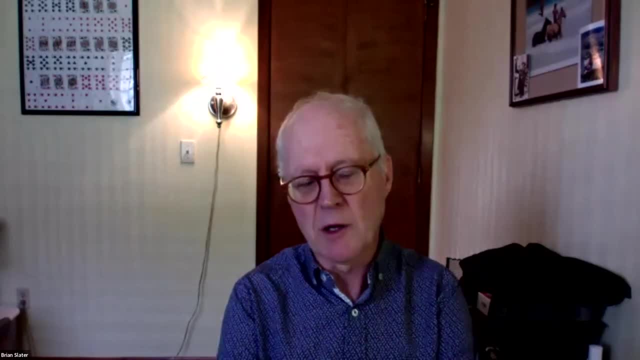 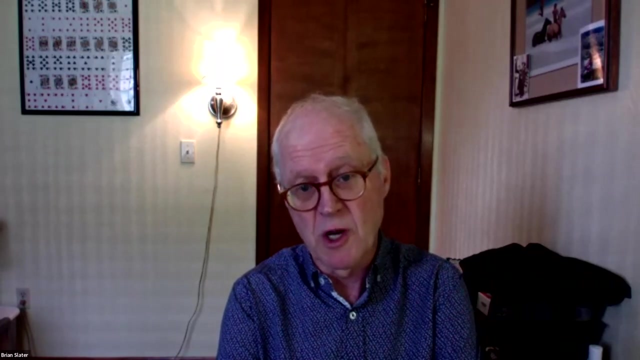 harder to see. that you know, um, uh, you know. however, desertification, that broad definition includes, uh, you know, destruction of soils to the extent that they can't support much vegetation, uh, but might still get enough rainfall, but they're not supporting vegetation due to severe erosion and compaction, for example. they're all parts of desertification. 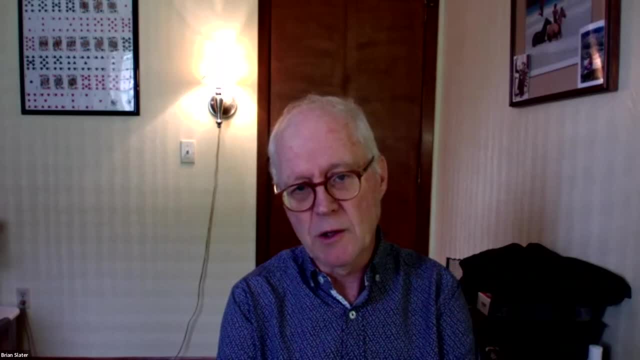 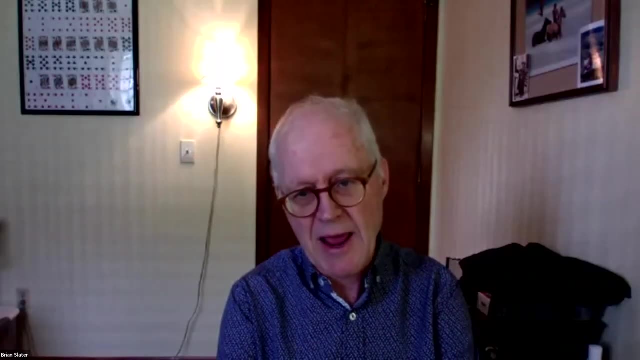 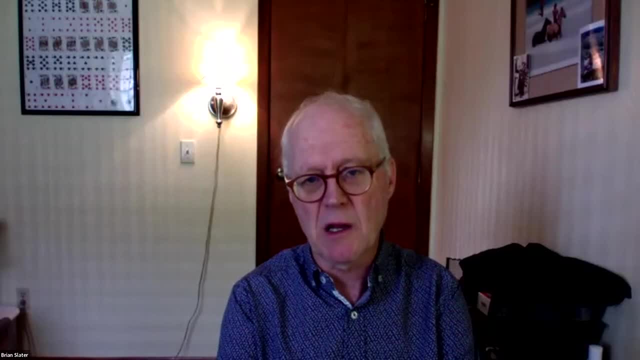 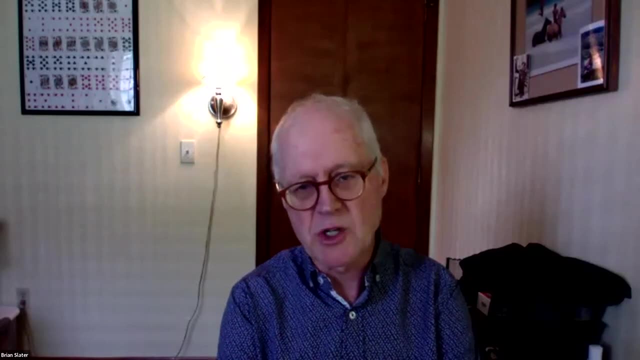 terms of like, actually you know making desert soils, that you know at least the way we see predictions going. you know- again i pointed out, you know, uh, warmer conditions, uh, perhaps a bit more moisture, but very intense storms, uh, more drought. you know, uh, more summer moisture deficit. 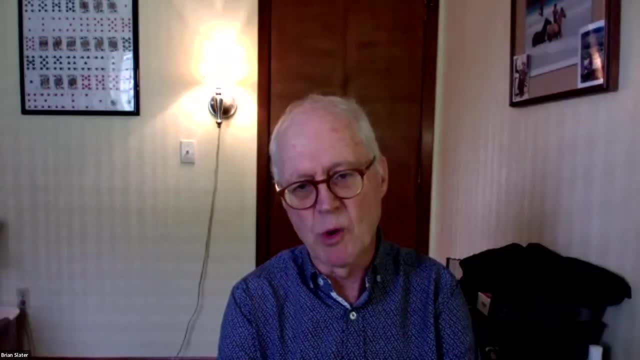 some years, all of those things, uh, you know, perhaps some more, you know, strong winds at some time of year, you know we might get more tornadoes, uh, these are things that we might worry about but i don't think they, you know, equate to desert. so desertification, if you look at that map, uh, the the big areas, uh, of worry for desertification, 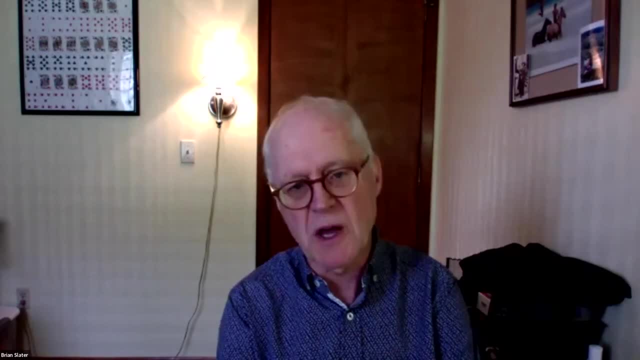 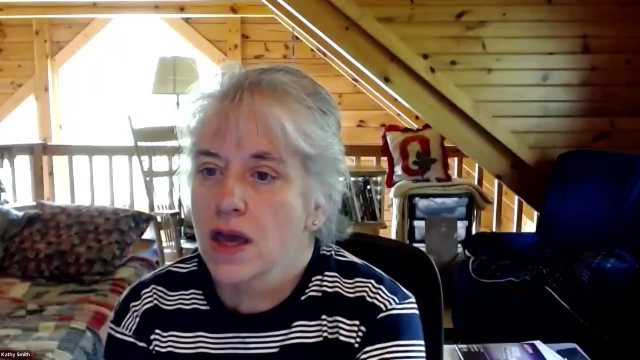 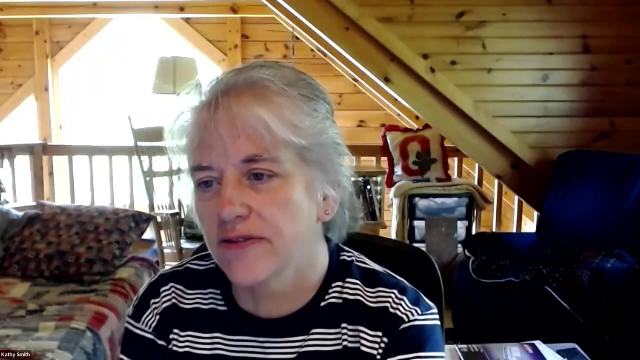 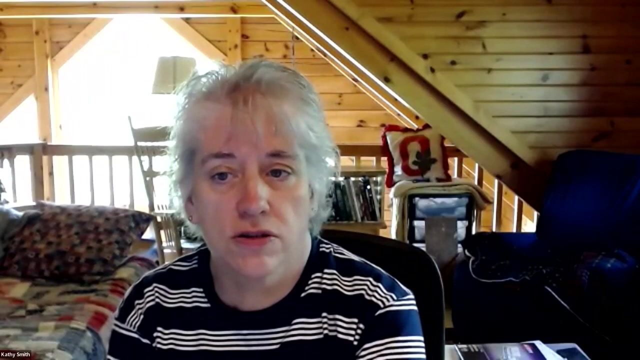 in the world? uh, are the the margins of current deserts? yeah, okay, and tropical areas? okay, um. sarah browning asks, as of our work. our work involves the removal and of invasive plants. could some of this activity, such as using forestry mulchers or herbicides, be doing more harm than good to the soil? 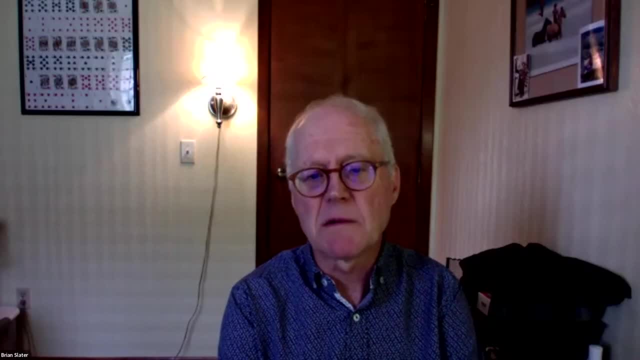 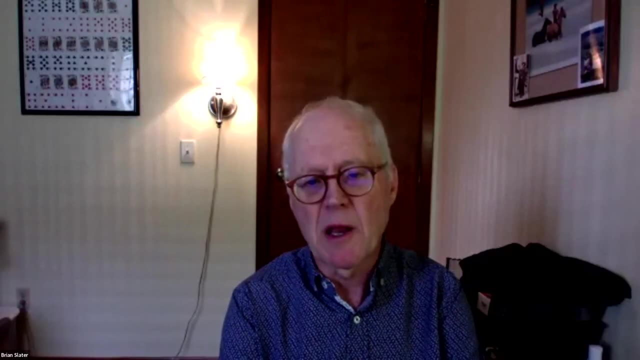 um, you know, yes, i, you know, just thinking about that, and again, i'm not, i'm not a forest manager and uh, uh, uh, you know. but but i think you know invasive plants are still plants, you know they. uh, you know, weeds, weeds have their role and you know i'm inclined to think invasive plants are there. because there's an imbalance, uh, generally, we've we've done things that are detrimental to the balance, uh, of of the original plant communities or those that are, you know, in balance with the environment. so, uh, i i think just at just removing them and not doing anything to uh, to. address those imbalances, uh, is is not a good thing. i think anything that disturbs the soil is going to reduce organic matter, uh, and, and you know, so, uh. so you know, as, as i mentioned, some of these things may not be necessarily intuitive. i mean the things that create above ground. 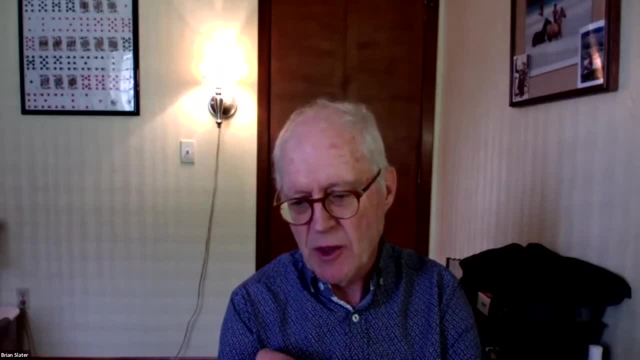 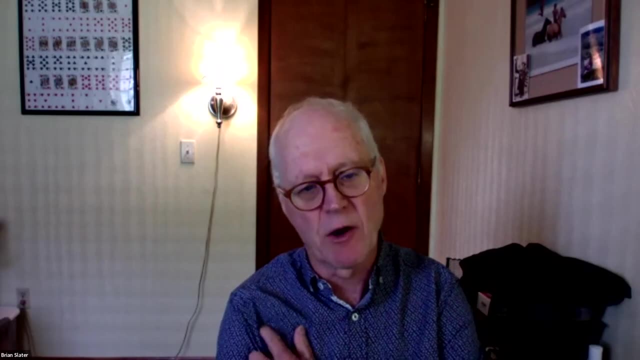 biomass in forests that store carbon may not be the the things that are going to store the most below ground carbon in the soil. so, you know, as managers we have to make uh trade offs here, you know. uh, you know that's not not a reason for not growing forests or keeping forests. 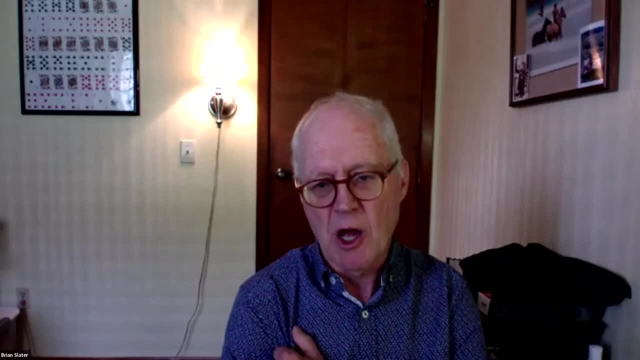 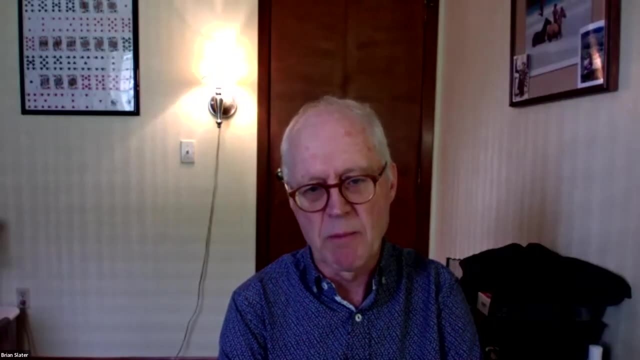 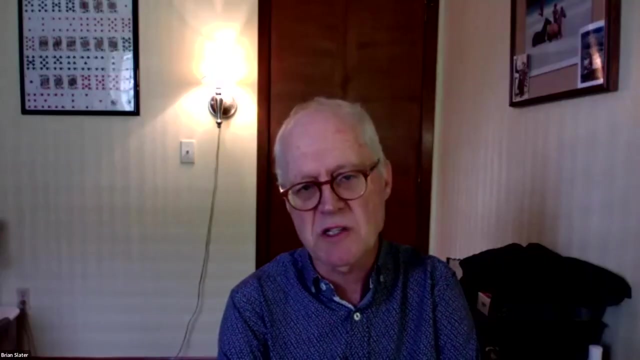 growing. uh uh, we may not get the most. uh uh, you know, to create the most soil carbon sequestration. we might want to have grasslands everywhere, but that that's not a good thing, you know. we we don't want to do that. so you know there are trade-offs for other ecosystem services costs, uh. 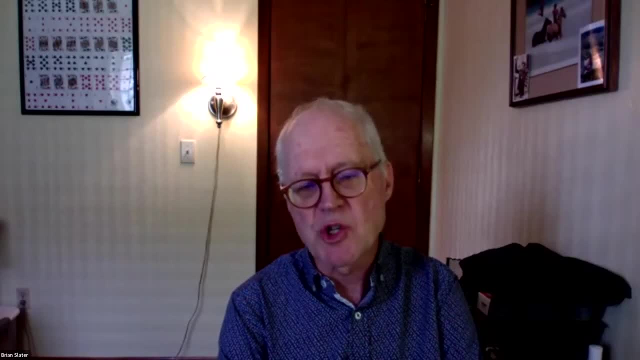 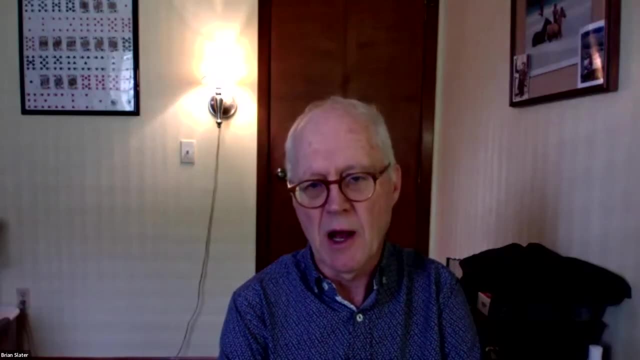 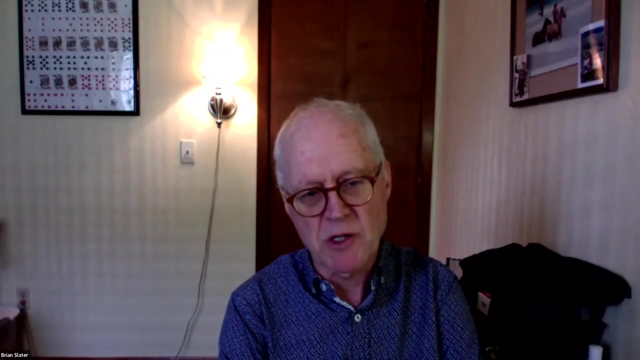 and everything else. so, in answer to your question, i i'm sure there are ways to uh to deal with uh- invasive species and uh and land preparation and land management within forests that minimize soil disturbance, and i've talked about some of those, you know, when i talked about soil health uh. 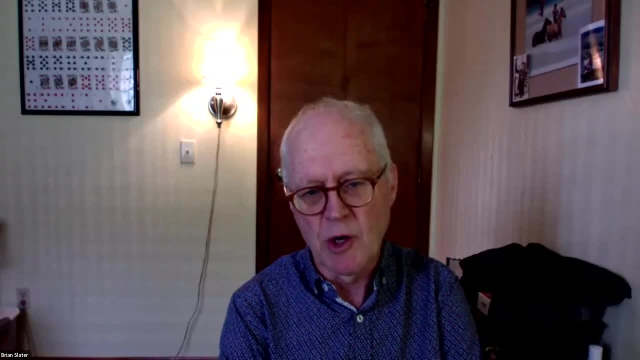 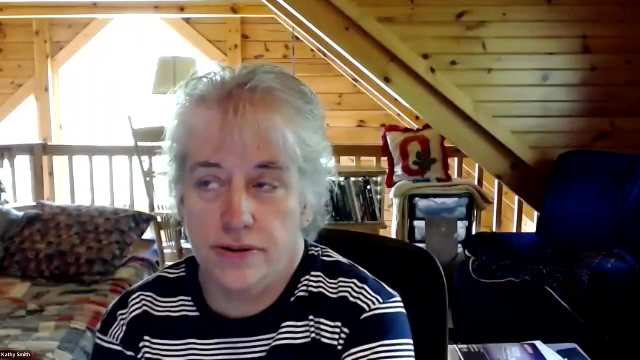 last year, you know i did talk about some of those, but uh, you know, that's definitely something that i think it, you know, ought to be something that's researched and uh and improved in terms of forest management. yeah, and i think that on the invasive plant side, i've been doing some 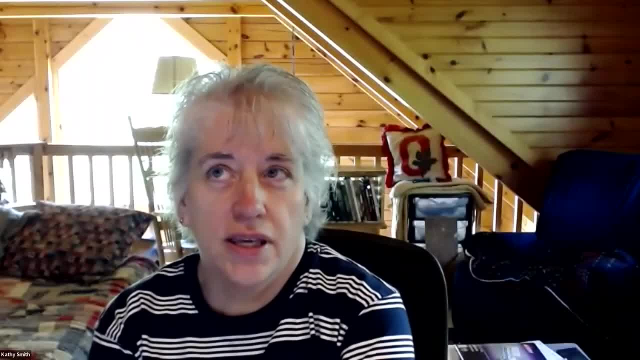 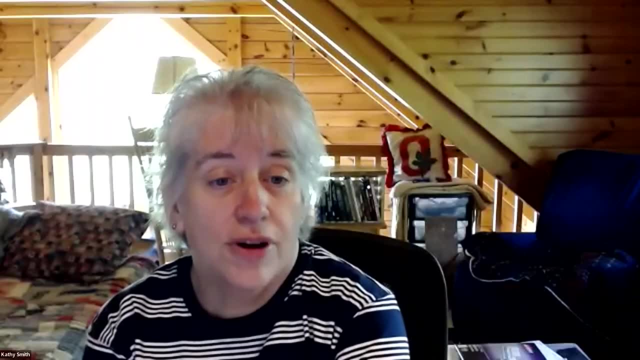 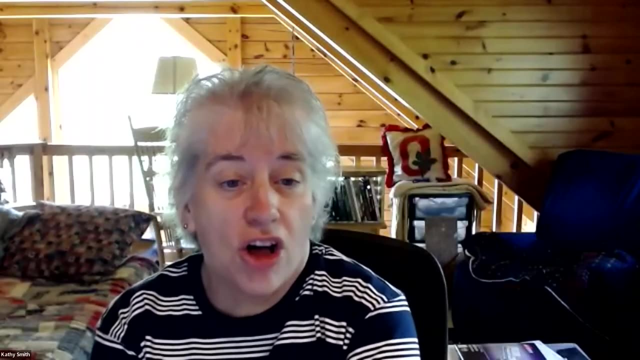 digging through the research about the impacts the invasive plants have on the soil. so some of them, you know, increase the ph um. some of them add things like calcium and manganese and other things. they all seem to have some kind of impact on the soil and i think you have to balance that out. 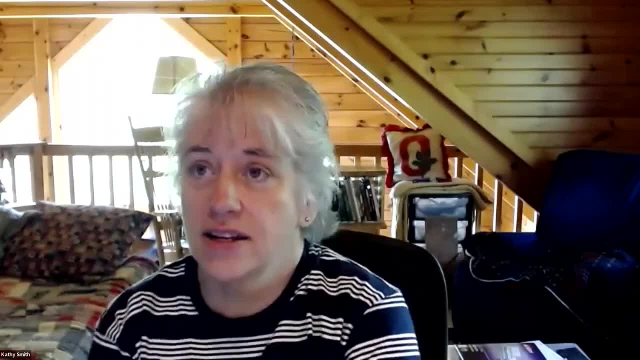 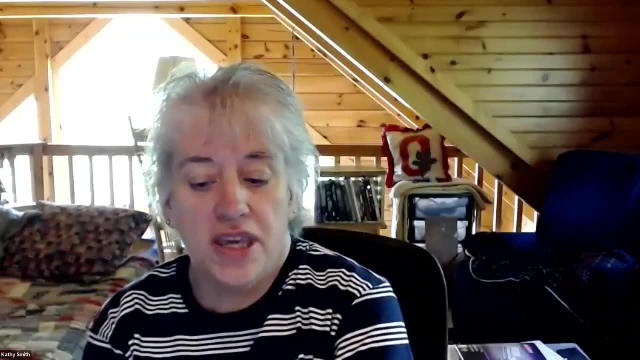 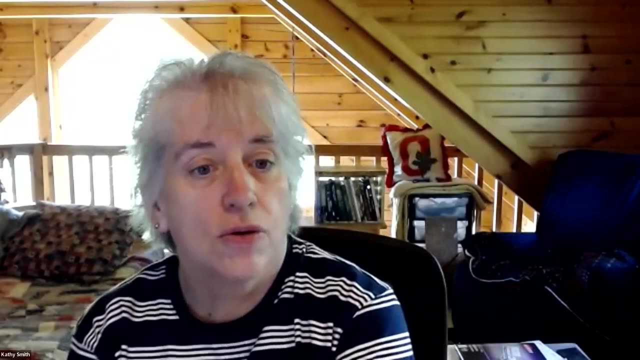 with. i mean if the ph changes. where i've seen that the most is a couple park districts that have removed buckthorn and the ph has changed so drastically that the plants they want to put back in that were there before will no longer survive in those phs. so those are the kind of 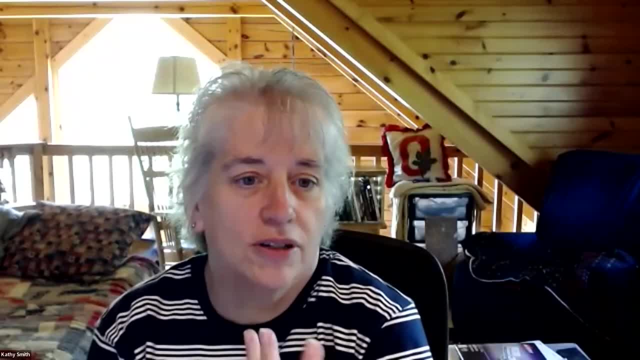 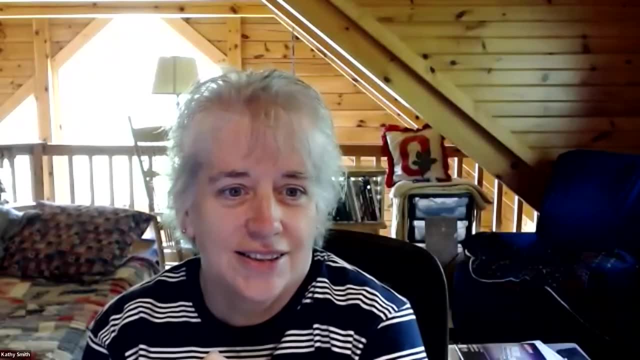 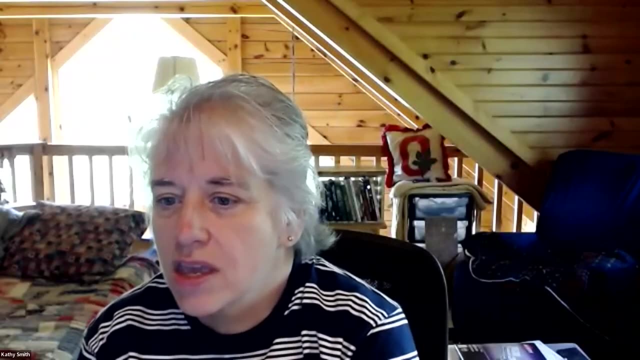 decisions that managers i mean, because they do impact the soil and what that characteristic is, and so it's not an easy yay or nay. each site's going to be different. so, um, kathy, i did notice a a comment from kathleen bradley that earthworms do not leave. 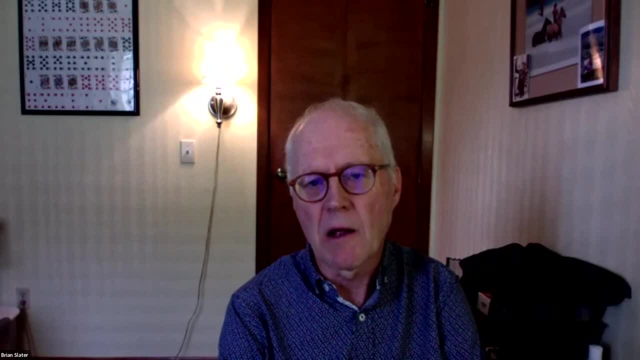 any organic matter in northeast ohio forest. uh, uh, now this, this may be true at the surface, but it's it's not true in the soil. um, you know, earthworms are detroit awards and they, uh, they break up surface organic matter and they take it into boroughs and they take it into the soil and they. 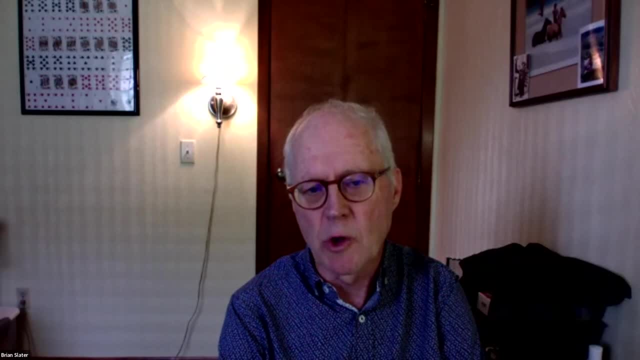 do this? uh, you know european night crawlers do this. uh, they take that soil, organic matter into boroughs and they also pass soil through their elementary systems and, uh, uh, and, and, during that process, organic matter is actually, uh, incorporated deeper into the soil than it would have been. 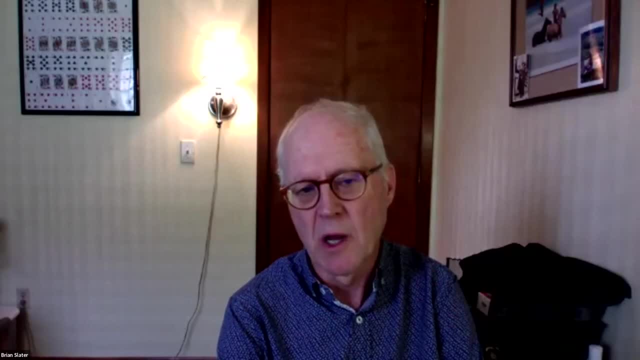 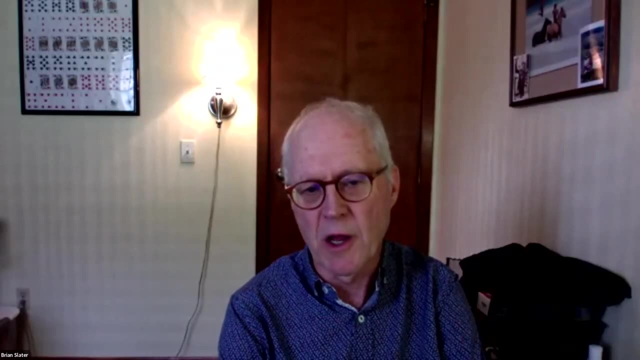 uh, otherwise, so you, you definitely do lose. i agree that that surface stuff, layers and horizons, uh, are strongly influenced by earthworms, but, uh, it's, it's. it's not correct that that that if you consider the forest to be, you know, if you consider the forest to be, you know, if you consider. 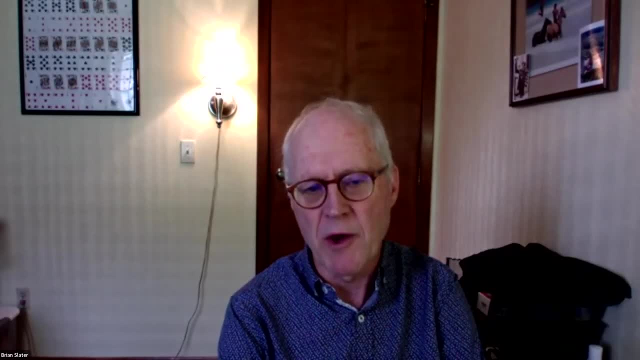 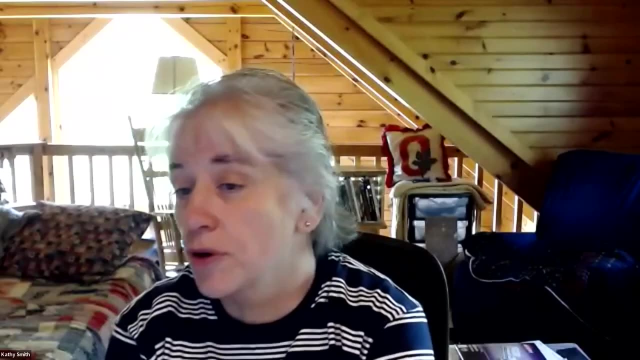 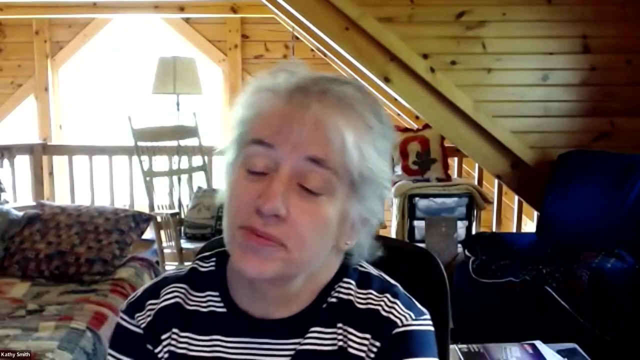 the forest to be more than the above ground cover. uh, they, they don't remove all the carbon. that's not right, okay, um frank talks about ohio's forest cover. since 1990, our forest cover's gone from um well, actually it was like from the early 1900s. we were at about 10 percent forested and now we're at 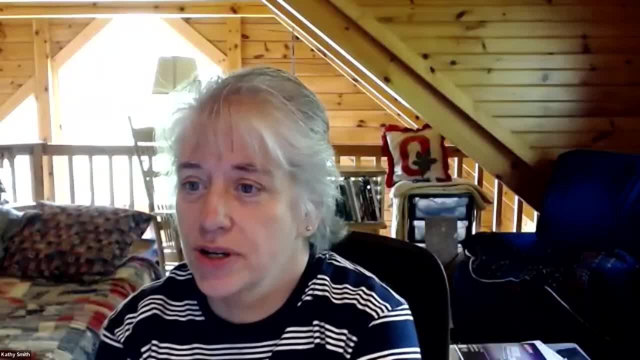 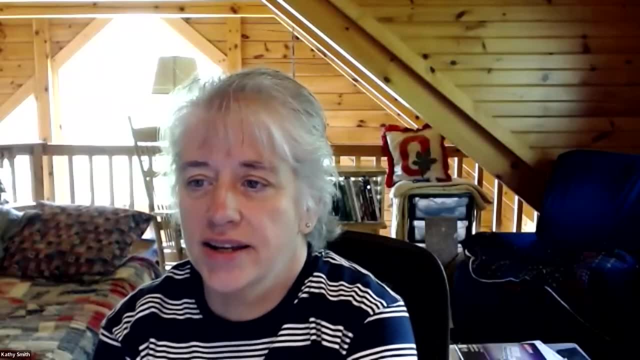 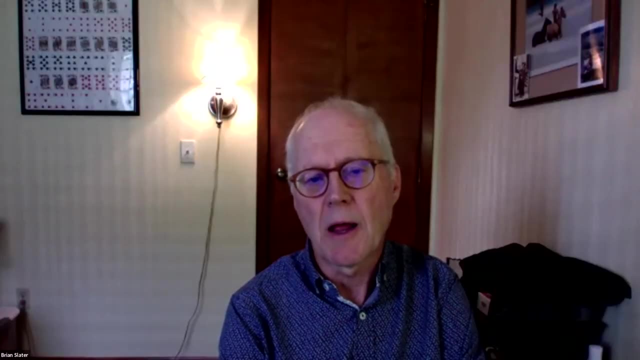 about 31 percent. it varies a little bit- 30- 31.. um, i believe other states such as pennsylvania, michigan, etc. have seen similar changes. how big of an impact has that had on carbon storage in soils? it's, it's had a large influence. uh, however, uh, the the the issue actually is that sequestering carbon. 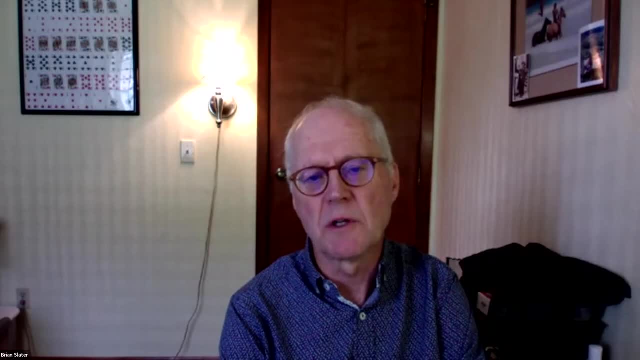 in soil in a forest is a relatively uh, slow process. okay, so when forests were removed in ohio, they were mostly replaced with earthworms. they were mostly replaced with earthworms. they were mostly with earthworms. they were mostly replaced with earthworms. they were mostly replaced with earthworms. 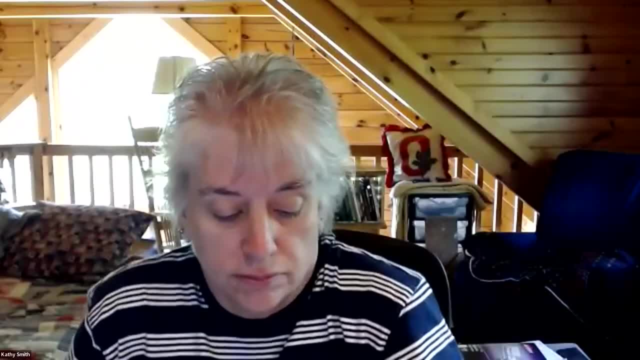 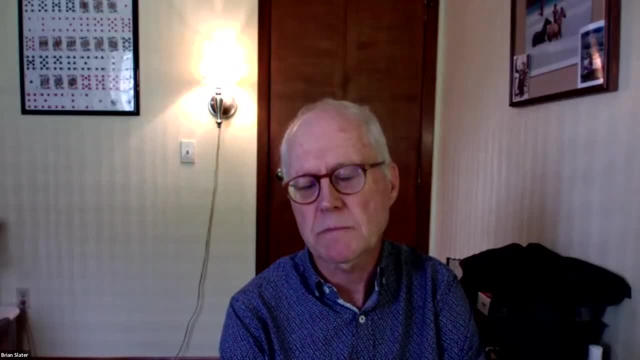 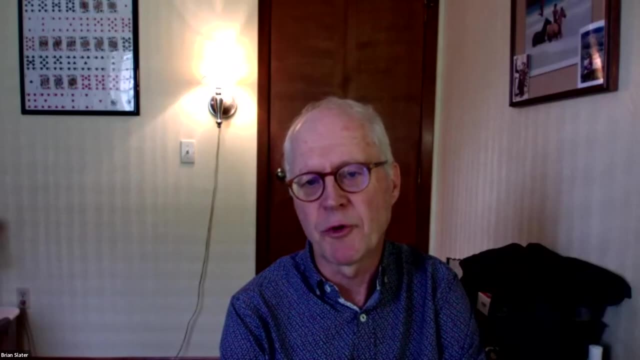 agriculture mostly right. the soils were plowed, uh, they may have not been plowed long term, but when they were plowed, a lot of soil loss happened too through erosion, and during that period you know, approximately 30 percent on average, uh, of soil organic carbon was lost from ohio soils, approximately. 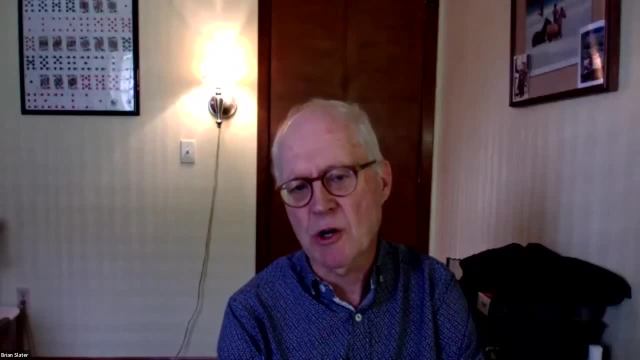 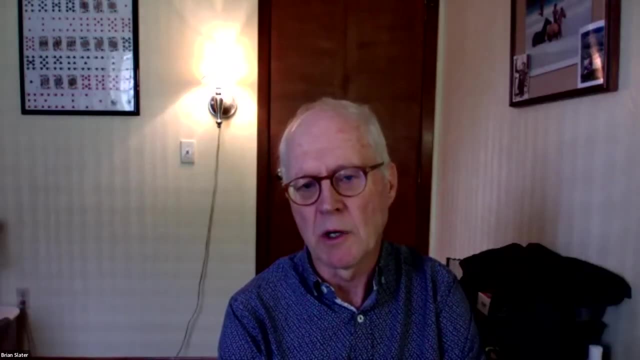 30 percent, um, and that's across across the state. so, uh, we know this from long-term studies. uh, uh, you know, uh, particularly a study that was done by my deceased colleague, uh, frank calhoun, in northwest ohio. he went back in the very first day i arrived in ohio from australia. uh, i went out with 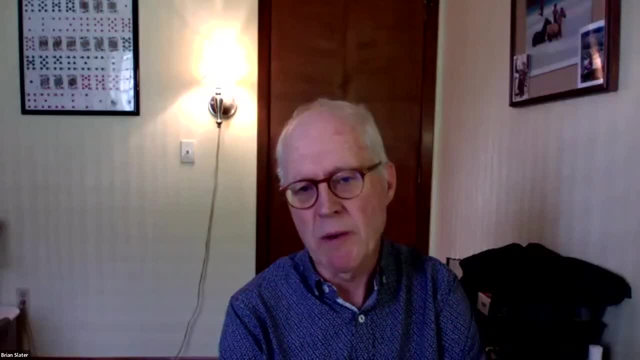 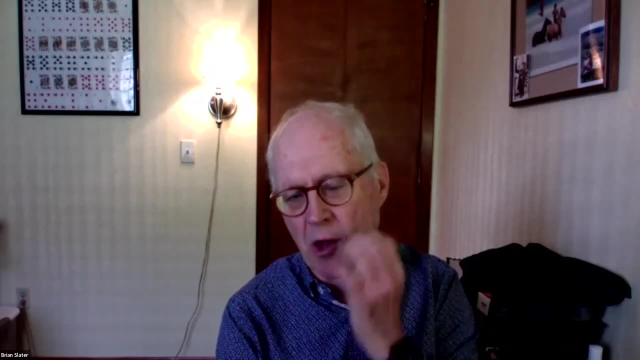 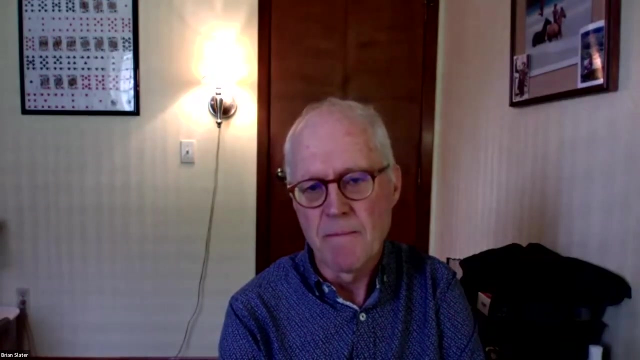 frank. and then through that first winter we we went out and went back to the old soil survey sites in northwest ohio and redug the soil. so those soils were initially analyzed in the 1950s- uh and uh and, and you know by by and uh and, and you know by the 1990s, uh, they, you know many of them had changed and 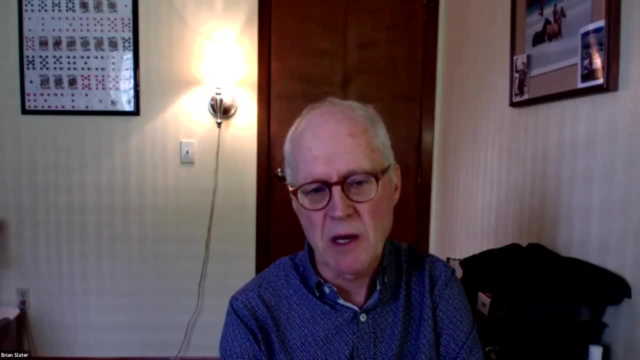 increased back in carbon but compared to- and we compared- areas that were still under wood lots, uh, you know, with with many of the other soils, and the loss is about 30 percent. um, this, this has been backed up, you know, in multiple studies and long-term sites across. 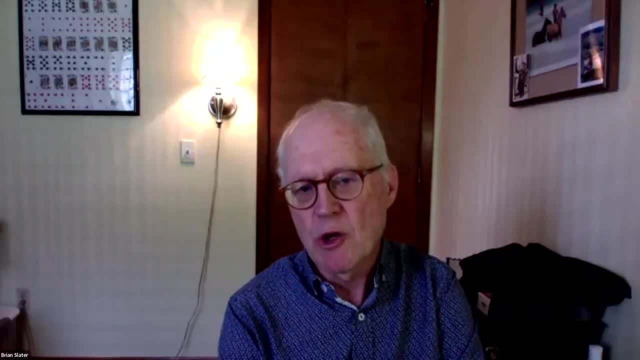 the united states. so when you re-establish forests, you know you do increase carbon again, you know, but it's it's relatively slow to be incorporated in the soil. it's a slower process. that happens, say in, uh in like uh lay farming or uh or rotating uh cropland, uh. 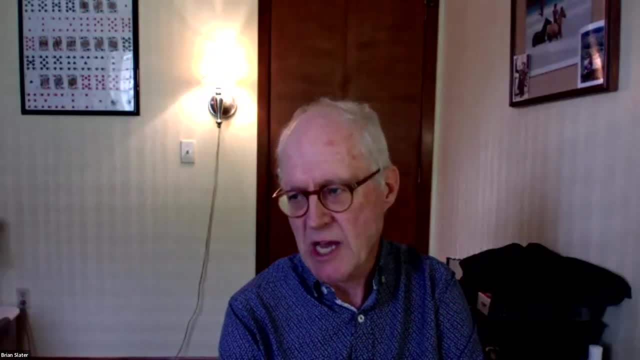 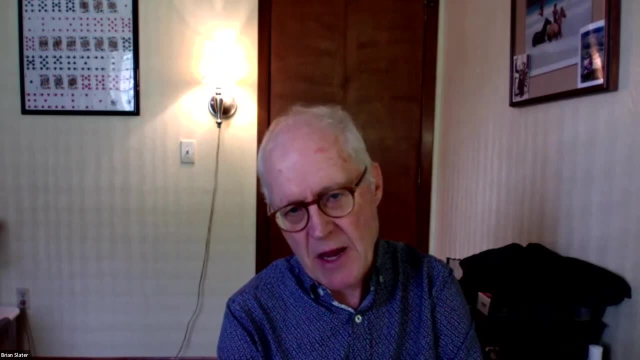 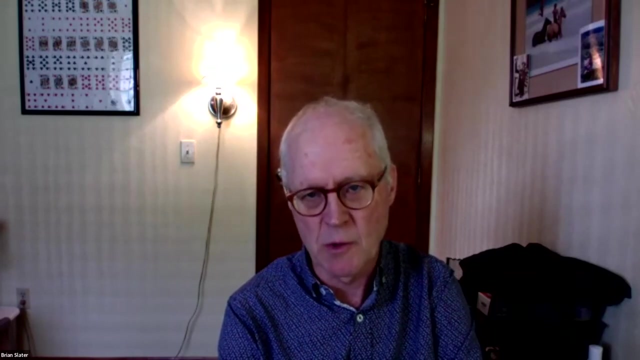 into cover crops and and uh and and rotations that put carbon directly into the below ground biomass. um, but uh. but on the other hand there's more, you know, that increases the above ground biomass. so forests are a good thing and that increase from 10 to 30 percent or so, uh, has been extremely. 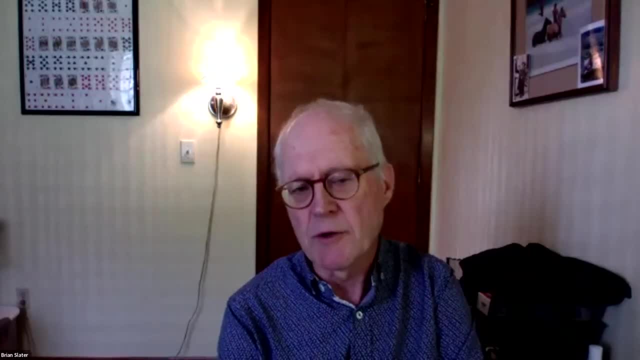 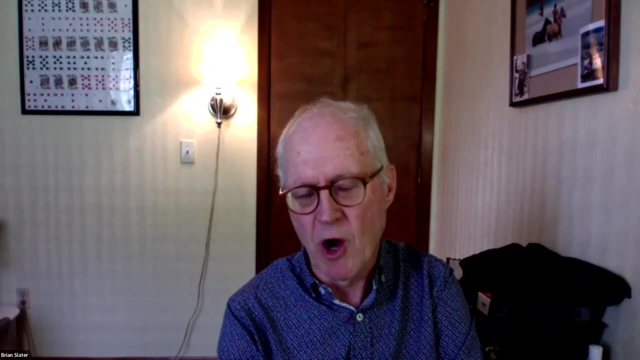 important for sequestering carbon in ohio. so don't get me wrong. but in terms of changing the soil, it's an ongoing process and and studies show that the changes have not been- uh you know, nearly as strong in the soil as in the above ground violence. but over time you would expect that. 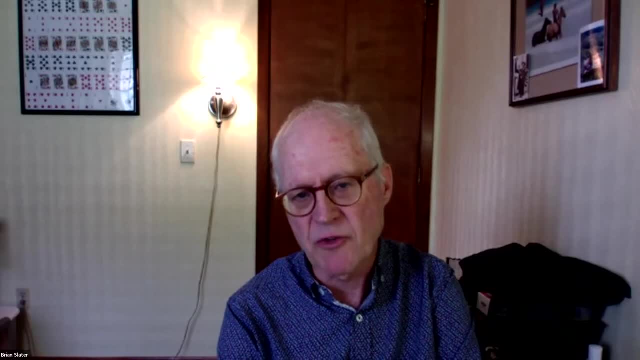 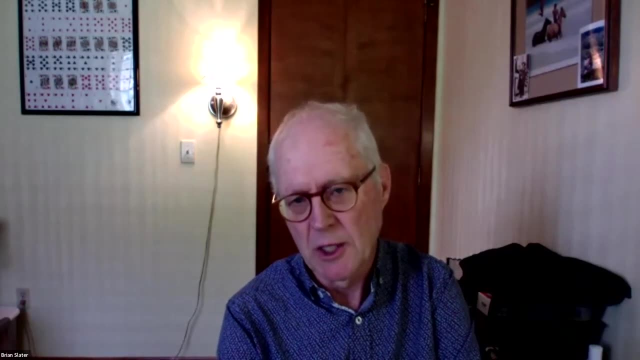 to increase. uh, you know, but these are managed forests in many cases too, so it takes a long time for that soil carbon to build up. yeah, we're talking about uh, decadal, uh, to centuries, to thousands of years, so it's, it's, it's pretty slow okay. 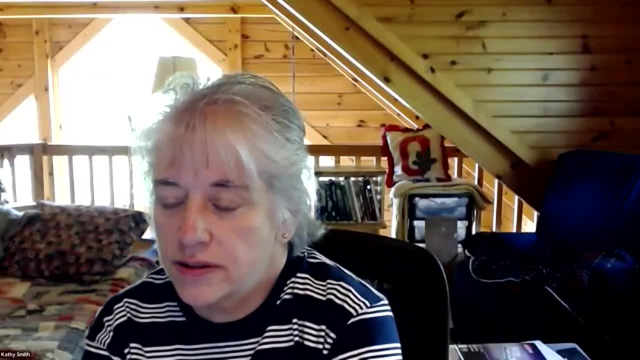 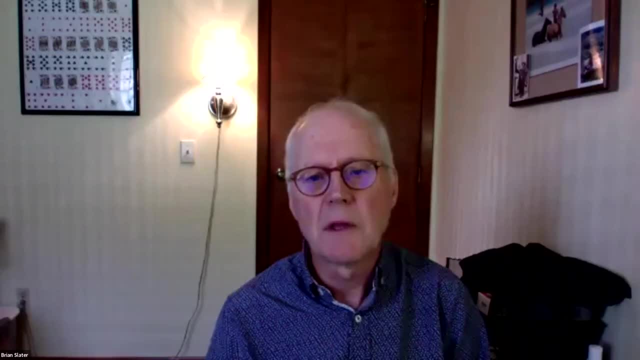 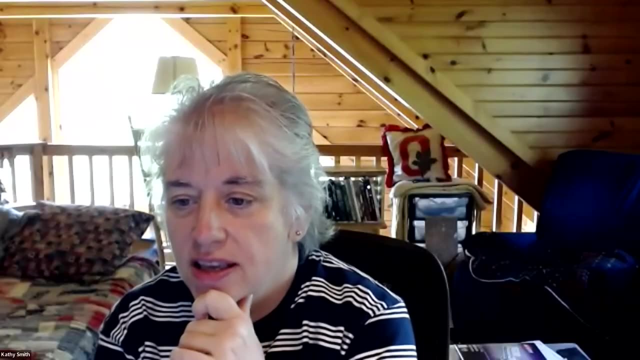 i'm gonna skip down to this anonymous one, um, because it seems like there's a lot here. can you see these? are you looking at these, brian? uh, the anonymous one down there. temperature increases, evaporation from the warmer seas and fresh water increases. the sun's energy is used in. the summer for a longer period of time. the temperature increases and that causes more precipitation. so the summer does not occur more, but as the weather changes more, then it's a little bit more dense, so it's not going to continue to cause more winter precipitation. so you see, the models i just showed you over here are, you can see, the summer accretion. 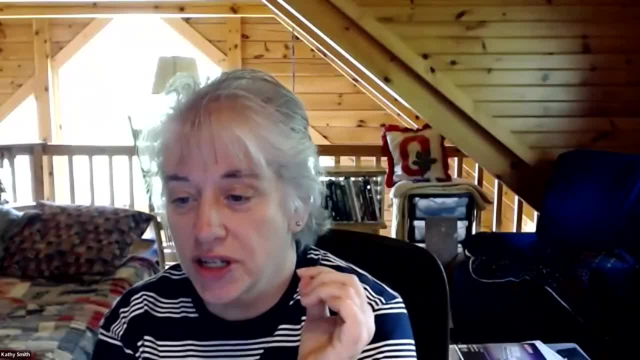 going back to what we had before we went back to summer. it changed the temperature exactly like what we saw yesterday, so it's going to increase. it does a lot of work to take some of the temperature into account. so what we're trying to do is we're trying to do is to 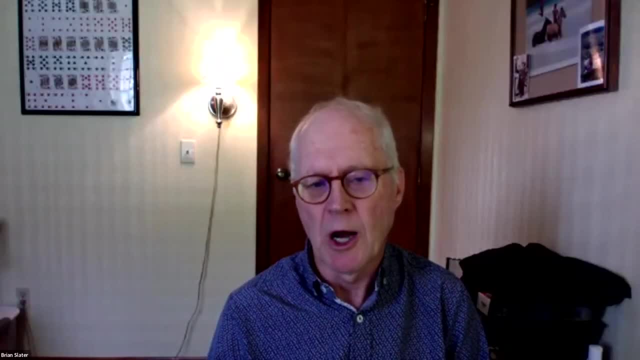 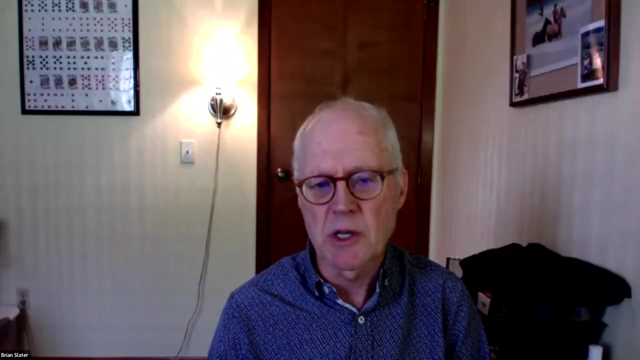 absolutely, this is exactly right. so, uh, erosion is already uh becoming a more and more serious problem in ohio. so you know, we imagine that. you know we did a lot about erosion. you know, uh, from the 19, late 20s, 30s. you know when the dust bowl happened and the soil conservation service uh, 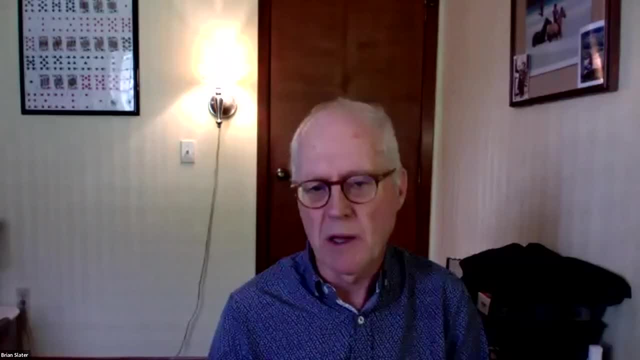 began. you know activity and farm management and uh soil conservation districts, etc. all of the work that's been done in forestry uh for soil erosion, uh in in no-till agriculture and minimum tillage. you know all of those things but uh, soil erosion is still an extremely serious problem and and 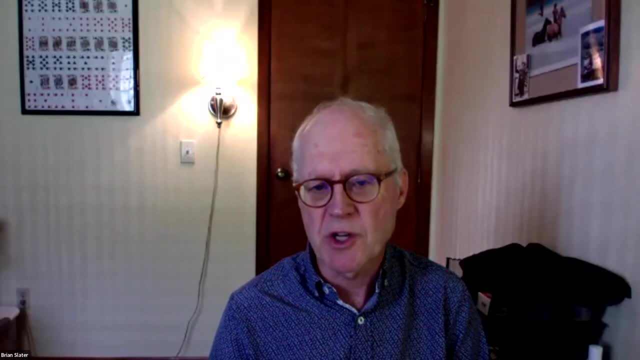 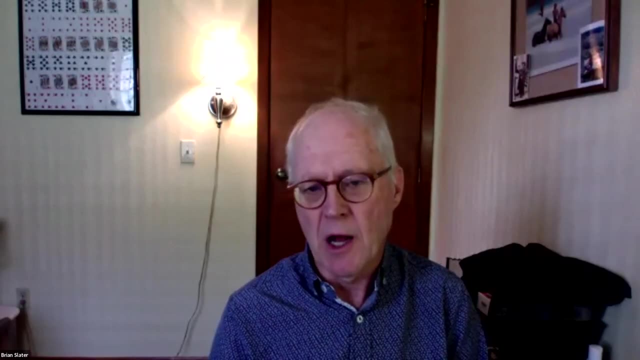 and now we see that the influences of climate change uh will have particular effects and and we know from various studies uh that, uh, that it's. you know, in cropland uh is is the worst place to soil erosion. uh, late in the summer, is is the worst, is the worst time. so before that, the plants completely covered the soil. but when we're starting to get the more intense storms and where, where we have moisture deficit in the soil, uh, so that the soil is relatively dry, so, uh, you know. so what happens? you know and and, in fact, um, i can talk a little bit about this directly because i've some research done by one. 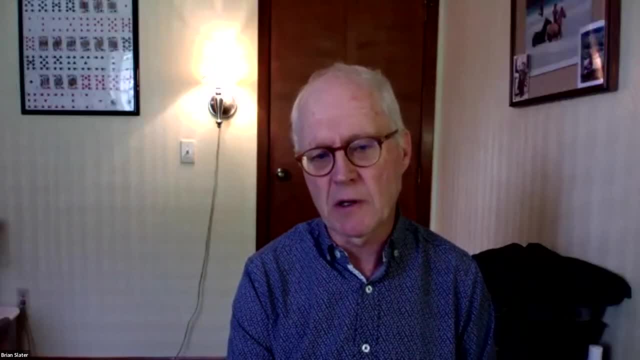 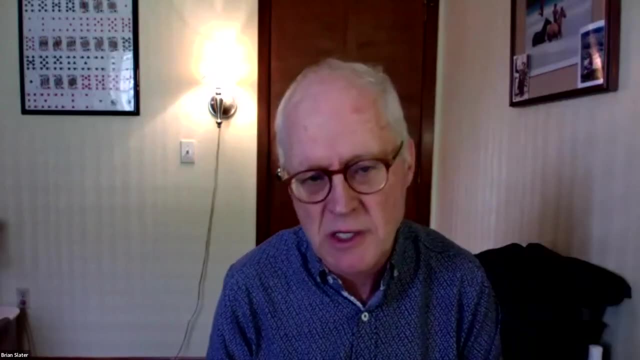 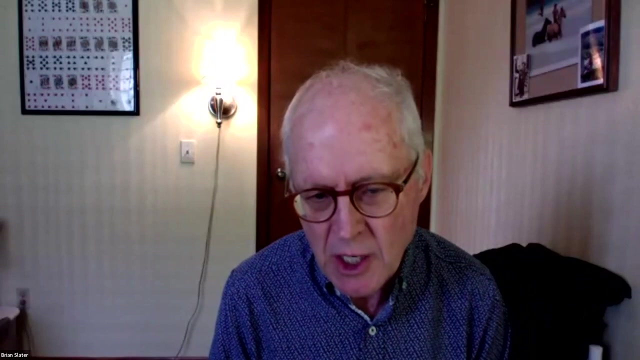 of my students, so we were absolutely stunned. uh, uh, um, emma kurth was her name and she did a research up at the you know what was the construct and research station. and uh, we looked, she looked at, uh, you know measuring actual soil loss and runoff during the growing season and uh, it was astounding that even when the crops were, 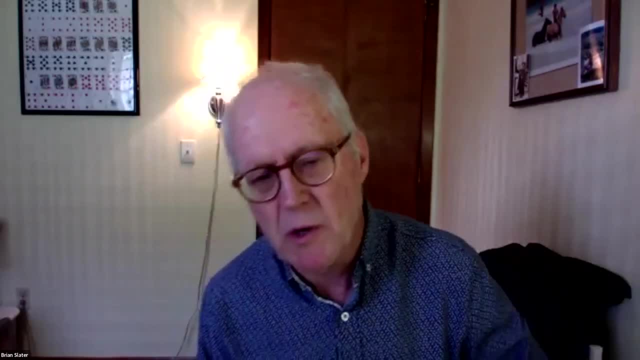 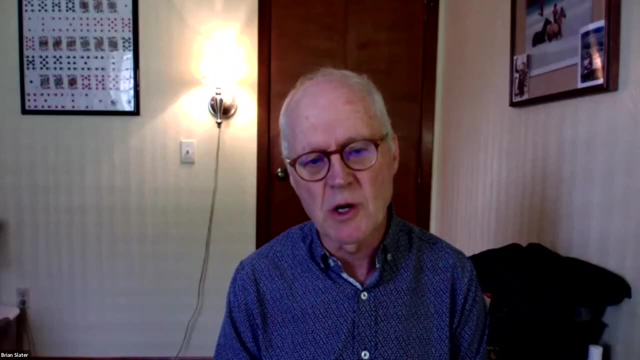 were growing. well, you know, towards the end of july and august, when we got intense storms, there was very serious levels, even even under no till uh of of soil erosion. so we we know that uh erosion is is a very serious problem and we know that uh erosion is is a very serious problem and we know. 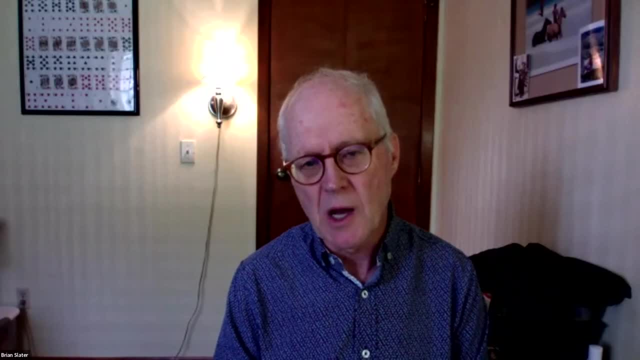 that uh, erosion is is a very serious problem and we know that uh, erosion is is important. and if we is important, and if we increase the intensity of storms, increase the intensity of storms, uh, the the more dry period, uh, uh, uh, the the more dry period, uh, uh, the. the one saving grace here: we, we might. 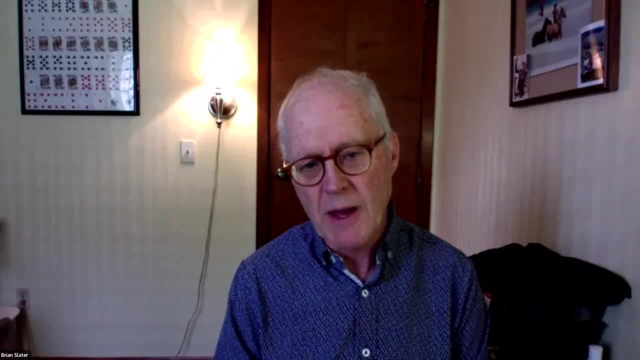 the the one saving grace here: we we might have more mature crops that i talked have more mature crops that i talked about before. so that might be the one about before. so that might be the one thing that influences better cover later thing that influences better cover later in the growing season. but i think, uh, you, 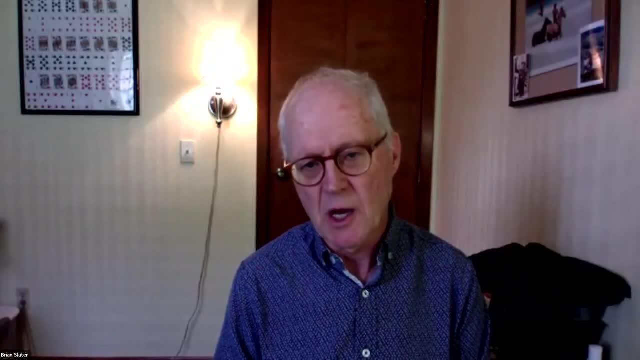 in the growing season. but i think, uh, you know i'm always cognizant of how serious, know i'm always cognizant of how serious erosion is uh in ohio. you know we go, erosion is uh in ohio. you know we go into fields, even though till fields and 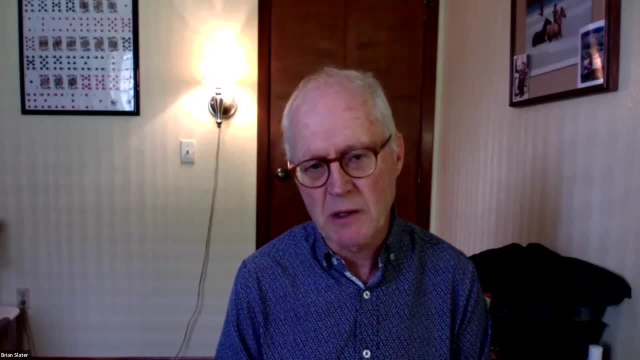 into fields, even though till fields and, uh, we, you know, this spring, you know we had, uh, we, you know this spring, you know, we had this wet spring. we had lots of rain. this wet spring, we had lots of rain. uh, we, you know, when i was out with my 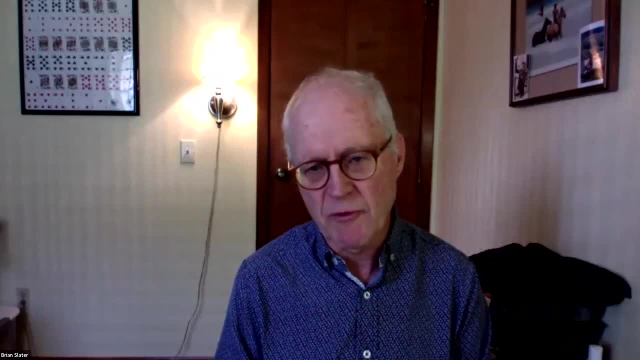 uh, we, you know, when i was out with my, uh, with my colleagues, uh getting these, uh with my colleagues, uh getting these sites ready for my soil judging contest, sites ready for my soil judging contest, all of these were in farm fields and uh, all of these were in farm fields and uh, we saw, you know, and most of them are. 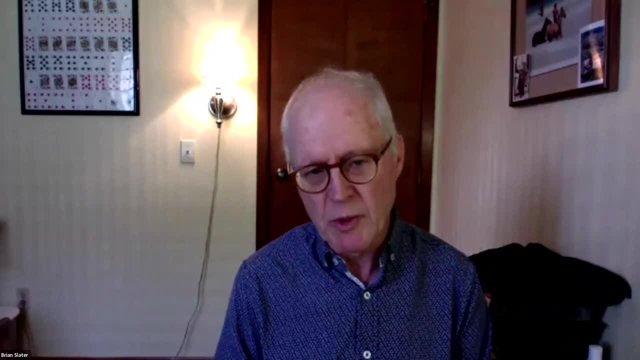 we saw, you know, and most of them are great cooperators. great people who, great cooperators, great people who, uh, you know who are doing the right thing. uh, you know who are doing the right thing- um and uh, significant soil erosion. um and uh, significant soil erosion, and it, you know, it's heartbreaking even for 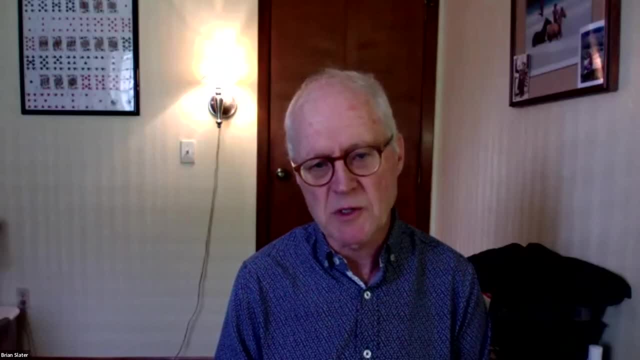 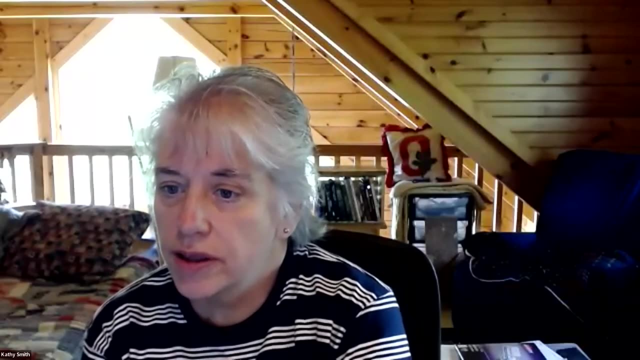 and it, you know it's heartbreaking, even for those farmers, those farmers. so erosion is not a problem, that's gone. so erosion is not a problem, that's gone away. you know away. you know that's true. um, so i'm gonna. that's true. um, so i'm gonna. sue's got a couple here that um, she. 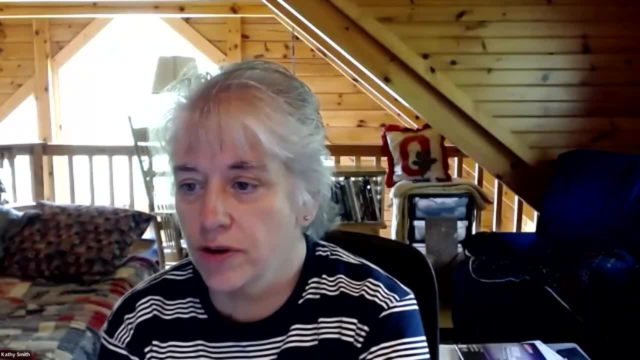 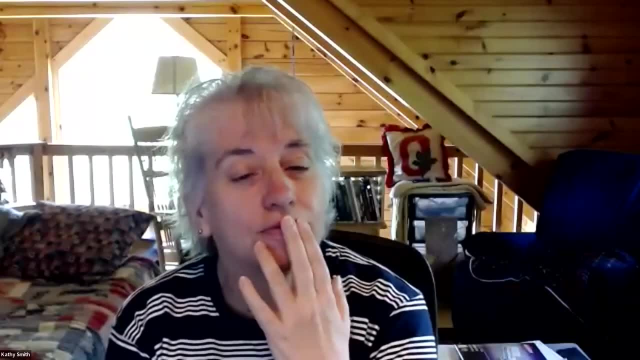 sue's got a couple here that, um, she asked: how do you measure how much? asked: how do you measure how much organic matter has formed? over a million organic matter has formed over a million years years. or how do you measure the carbon that? or how do you measure the carbon that has been forming for millions of years? 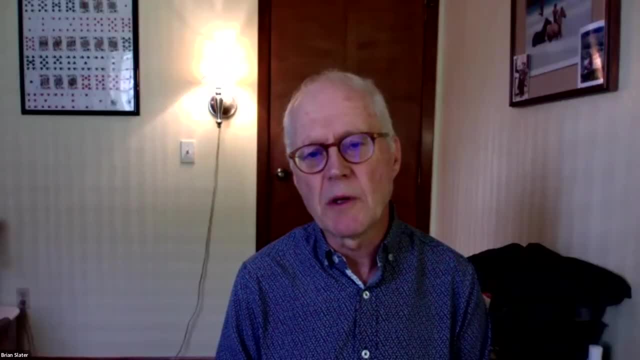 has been forming for millions of years. well, there are multiple ways to do this. well, there are multiple ways to do this. i mean we know that. i mean we know that, okay, over millions of years, um, i presume. okay, over millions of years, um, i presume you're talking about places that are 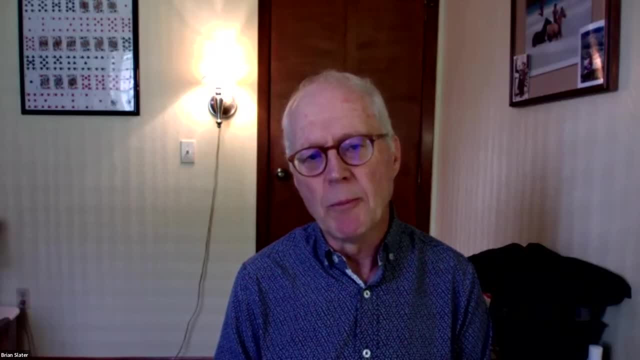 you're talking about places that are outside of ohio. because outside of ohio? because outside of ohio? because um uh, you know carbon in um uh, you know carbon in um uh you know carbon in in uh. ohio soils is much younger than in uh. ohio soils is much younger than. 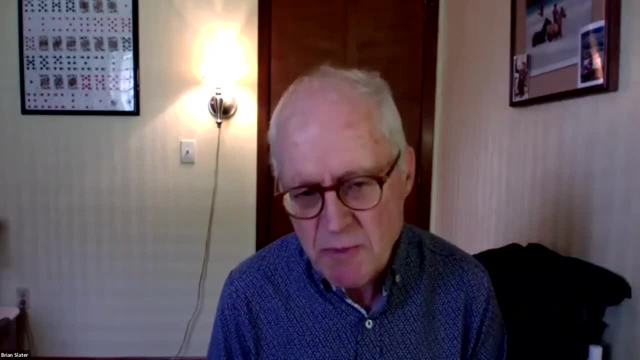 in uh ohio, soils is much younger than that, even in southeastern ohio, most of that. even in southeastern ohio, most of that. even in southeastern ohio, most of the soils were the soils, were the soils were influenced by the glaciation, even if influenced by the glaciation, even if. 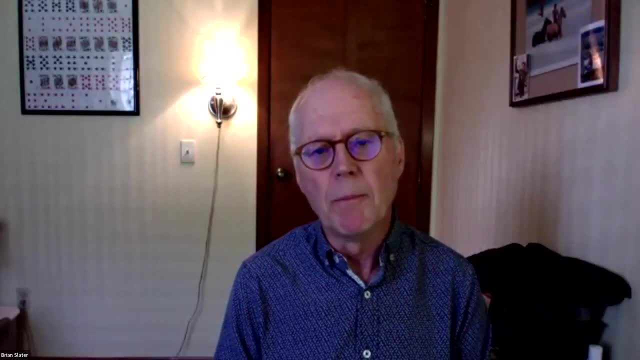 influenced by the glaciation, even if they didn't have ice over the top of they didn't have ice over the top of they didn't have ice over the top of them. so them, so them, so um, i think, um, i think um, i think, uh, you know, but i think over thousands. 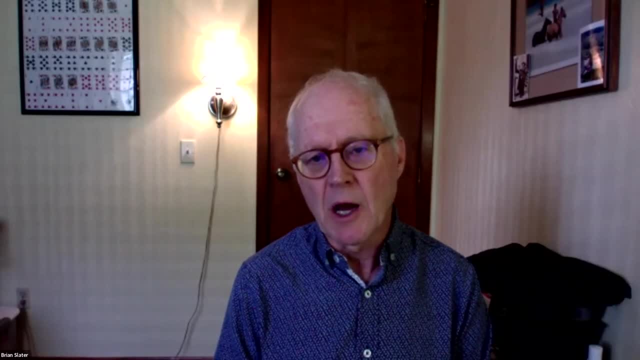 uh, you know, but i think over thousands. uh, you know, but i think over thousands of years of years of years. uh, we can uh, we can actively uh, we can uh, we can actively uh, we can uh, we can actively date carbon in soils, so carbon dating. date carbon in soils, so carbon dating. 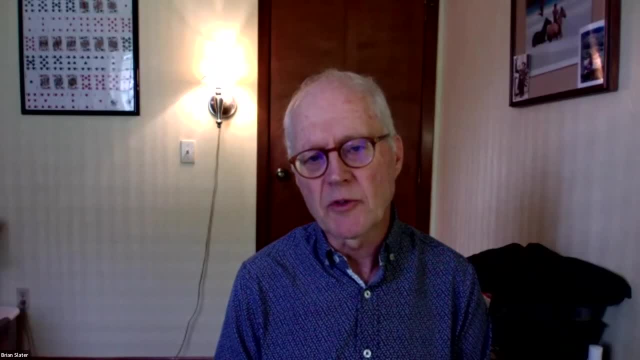 date carbon in soils. so carbon dating is the one way that's been used to do. is the one way that's been used to do? is the one way that's been used to do this, this, this, uh, so that you can take carbon out of. uh, so that you can take carbon out of. 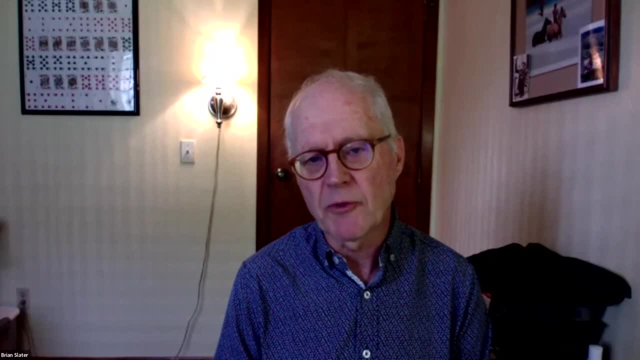 uh, so that you can take carbon out of the soil, the soil, the soil, uh, and work out how old it is by its uh, and work out how old it is by its uh, and work out how old it is by its balance of carbon isotopes. balance of carbon isotopes. 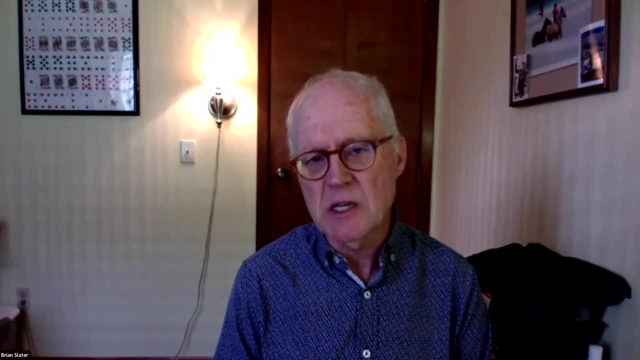 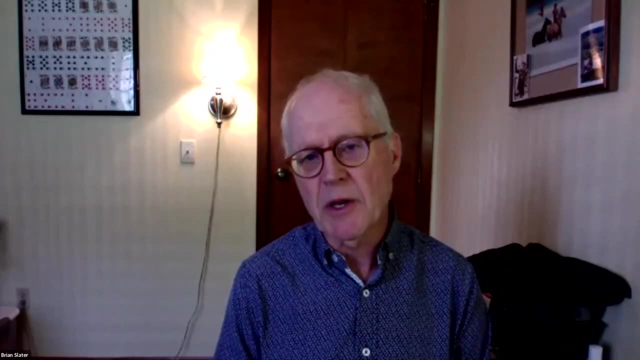 balance of carbon isotopes. um, so you know that that's actually one. um. so you know that that's actually one. um. so you know that that's actually one of the of the of the interactions so as carbon breaks down. interactions, so as carbon breaks down. interactions, so as carbon breaks down, uh, uh, in the soil, we can. 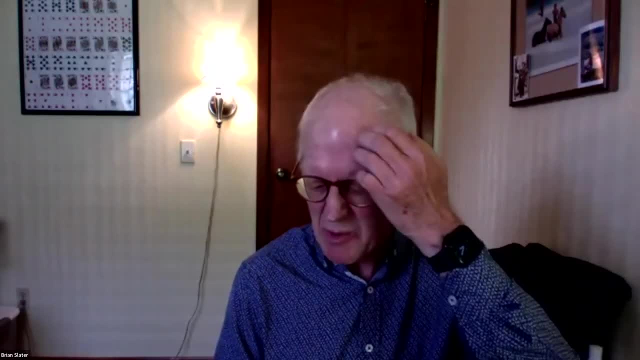 uh uh in the soil. we can uh uh in the soil. we can uh. we can uh measure different kinds of uh. we can uh measure different kinds of uh. we can uh measure different kinds of carbon. we can measure carbon. that's carbon. we can measure carbon. that's. 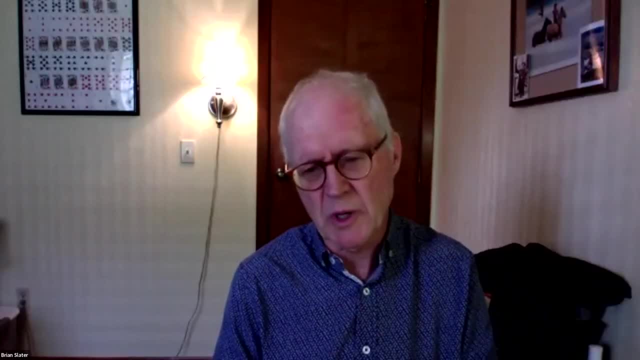 carbon. we can measure carbon. that's uh in the form of particulate matter. we uh in the form of particulate matter. we uh in the form of particulate matter. we can measure dissolved carbon. we can measure dissolved carbon. we can measure dissolved carbon. we we can measure carbon. that is uh changed. 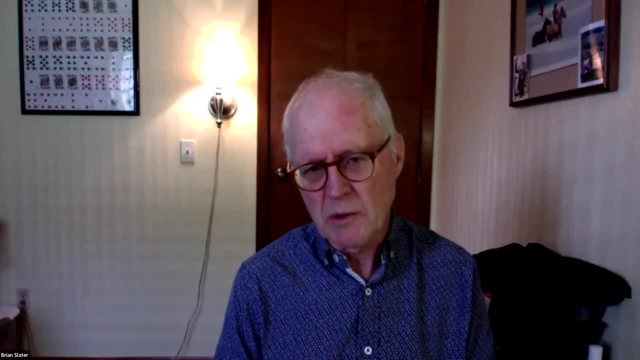 we can measure carbon that is uh changed. we can measure carbon that is uh changed into shorter chain organic carbon, into shorter chain organic carbon, into shorter chain organic carbon compounds, compounds, compounds. we can measure carbon that's protected. we can measure carbon that's protected inside soil aggregates. 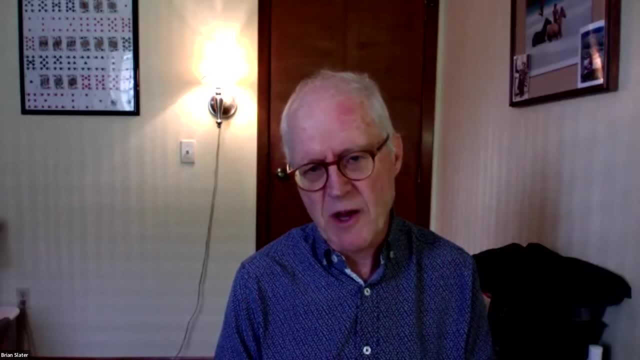 inside soil aggregates. inside soil aggregates: uh, there's so many different kinds and uh, there's so many different kinds and uh, there's so many different kinds, and we can measure those and each of those. we can measure those and each of those, we can measure those, and each of those has a different age profile. 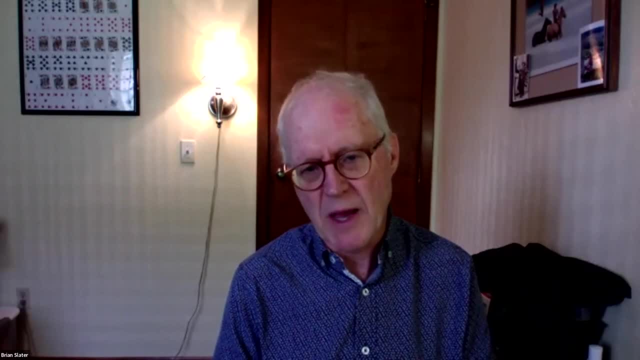 has a different age profile, has a different age profile. uh and, and those can actually be uh and, and those can actually be uh and, and those can actually be related back to. related back to related back to uh to to the different kinds of carbon. uh to to the different kinds of carbon. 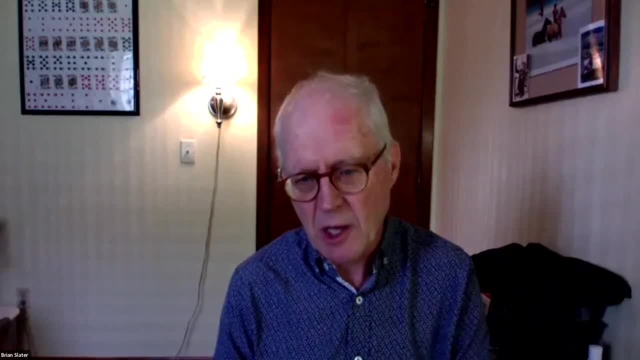 uh, to to the different kinds of carbon in soils, in soils, in soils, um, and so you know various dating has um, and so you know various dating has um, and so you know various dating has been done. i don't know how much has been been done. i don't know how much has been. 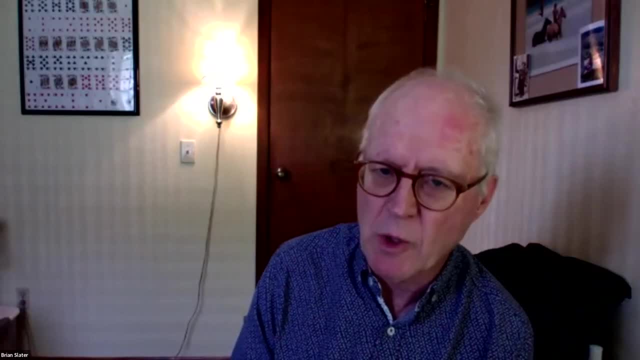 been done. i don't know how much has been done in ohio, but we know done in ohio. but we know done in ohio. but we know fairly. you know fairly generally about fairly. you know fairly generally about fairly. you know fairly generally about the age of carbon in most soils.